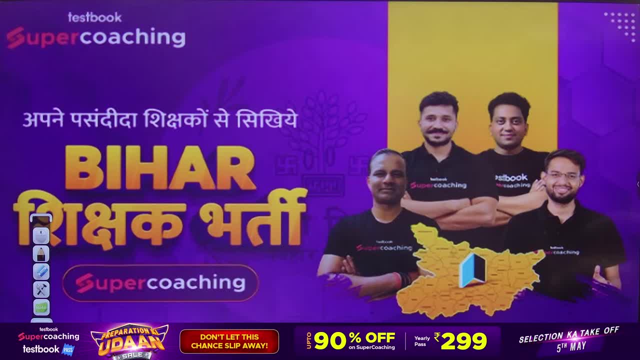 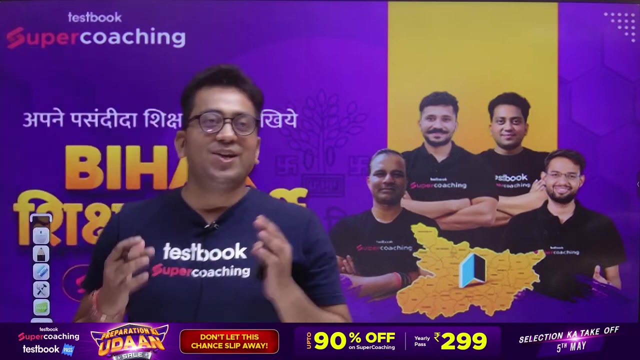 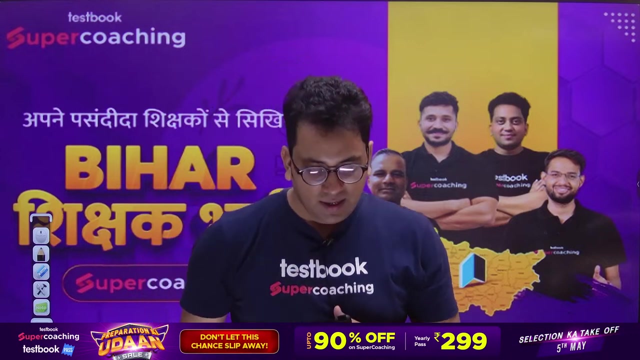 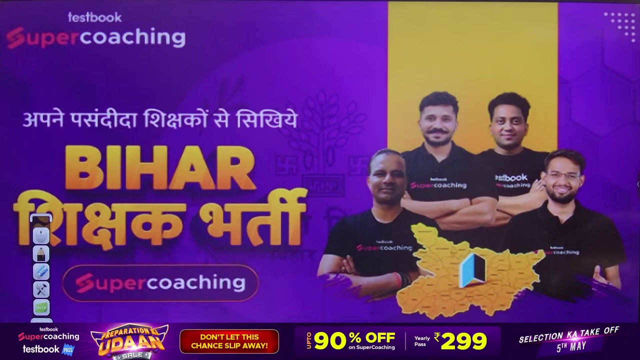 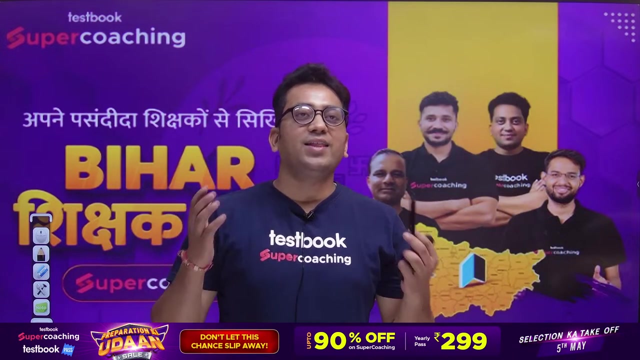 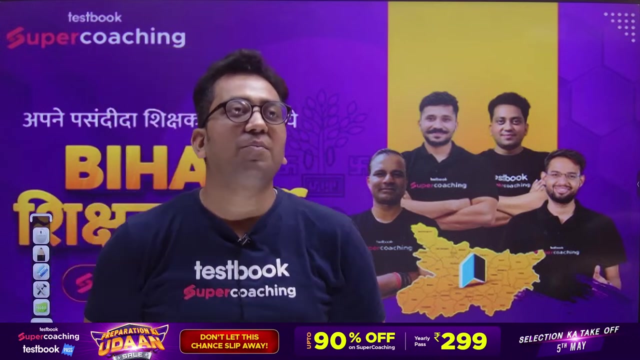 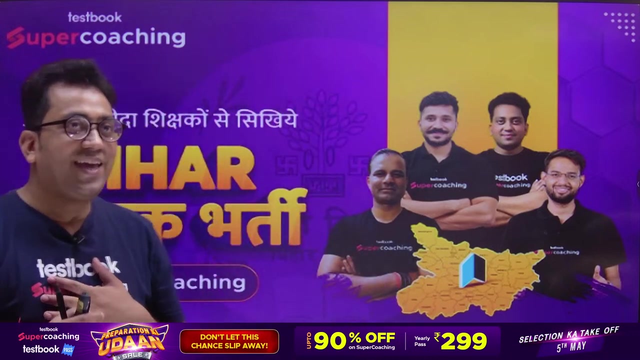 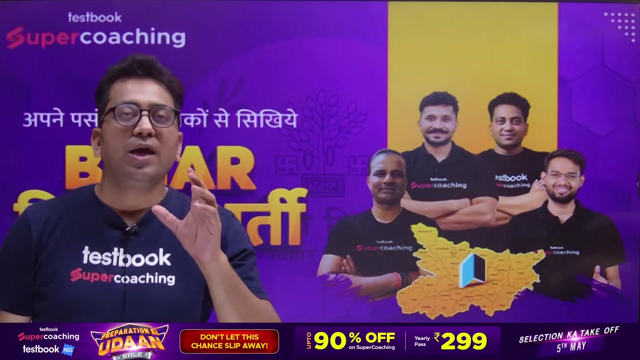 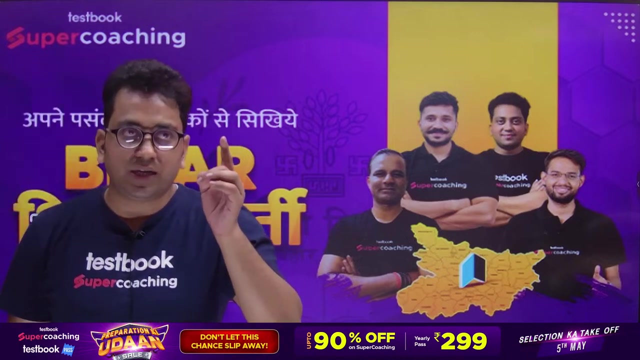 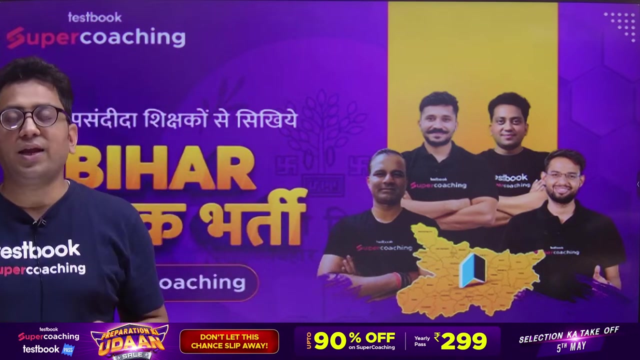 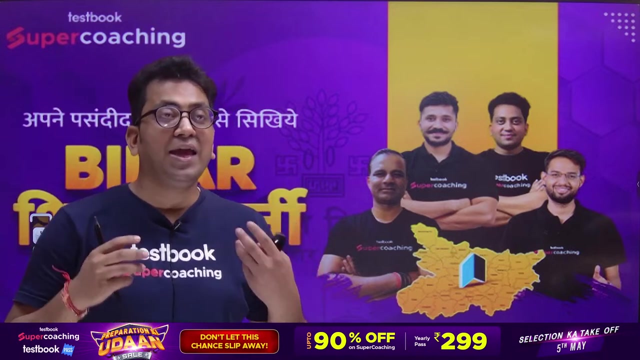 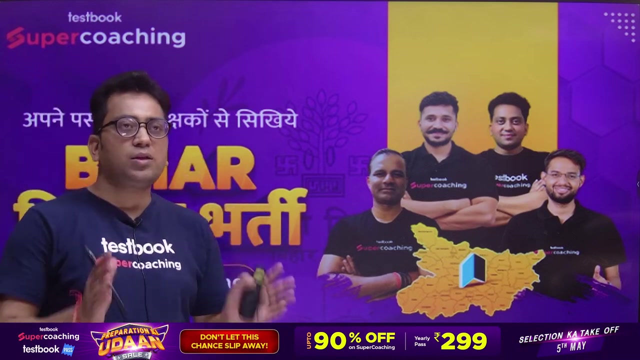 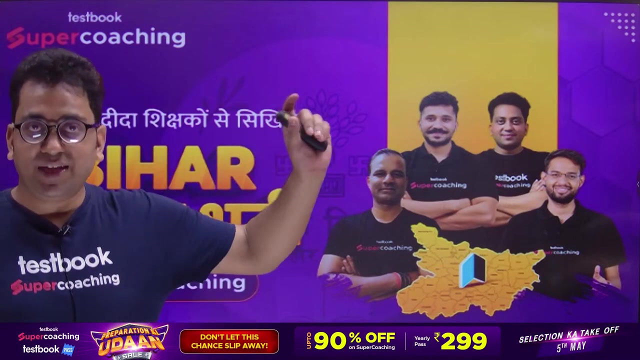 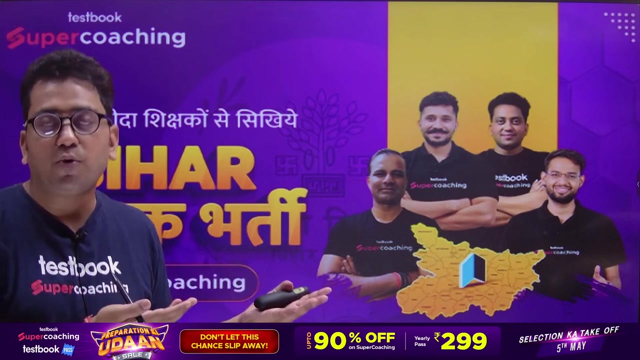 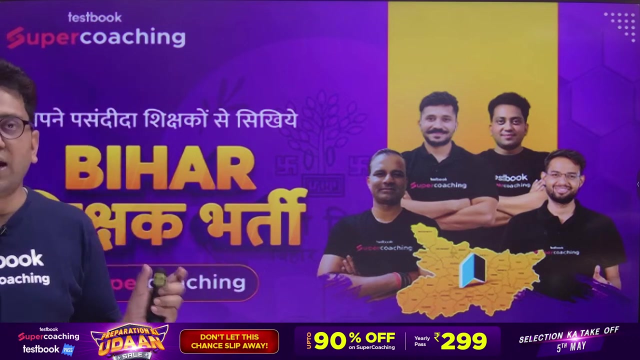 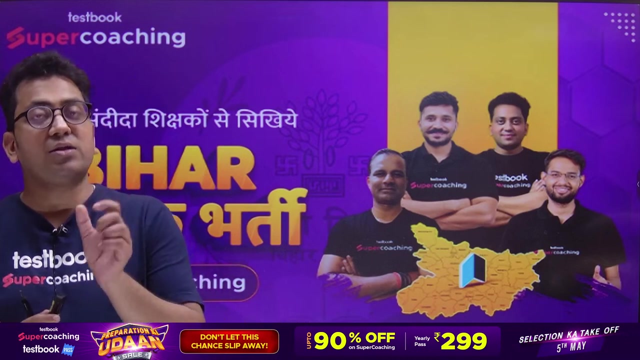 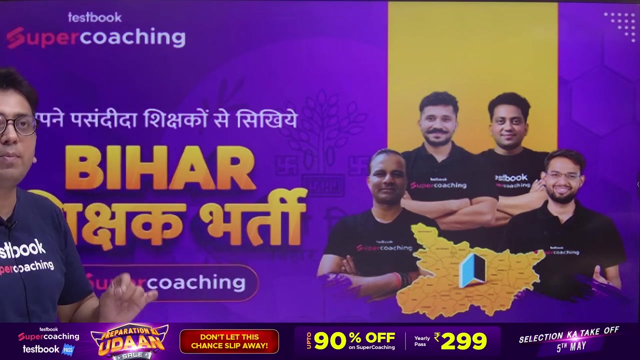 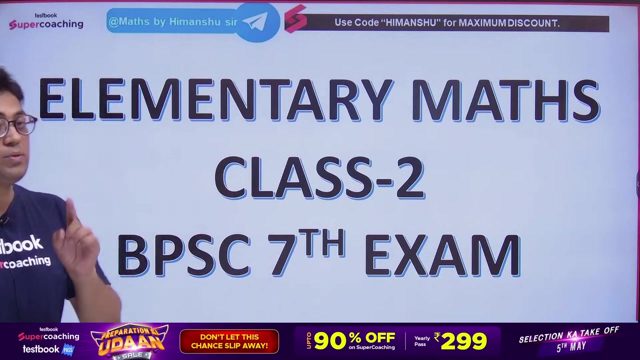 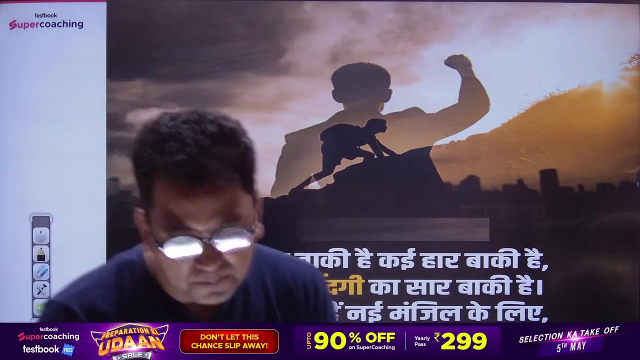 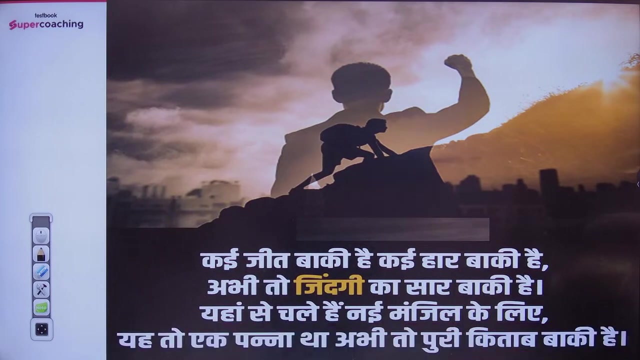 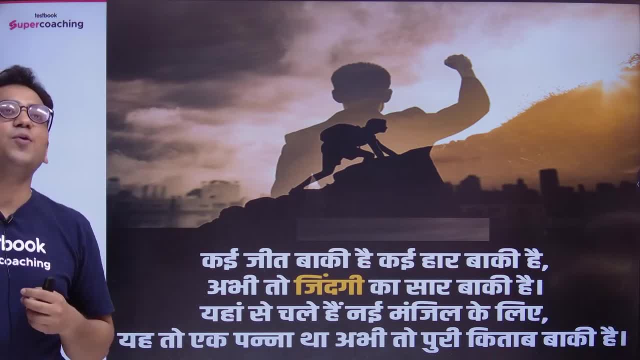 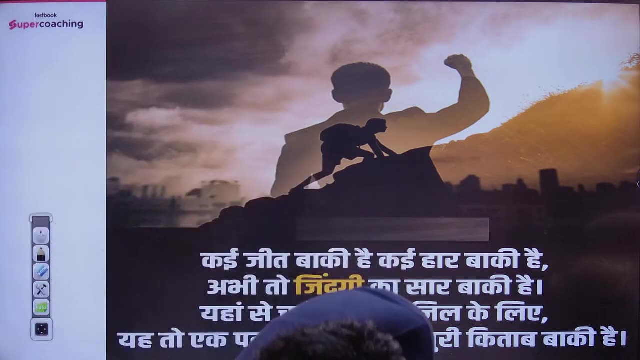 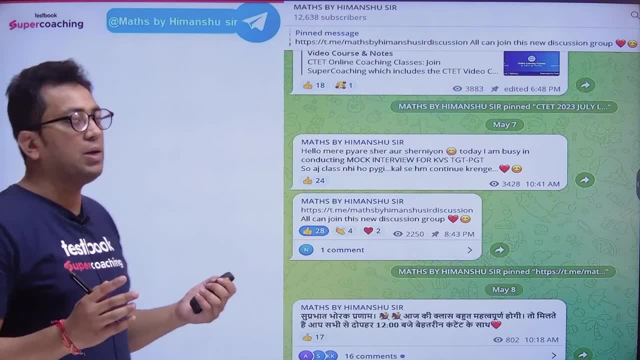 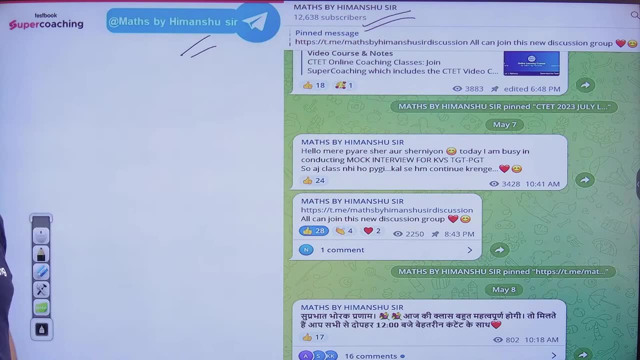 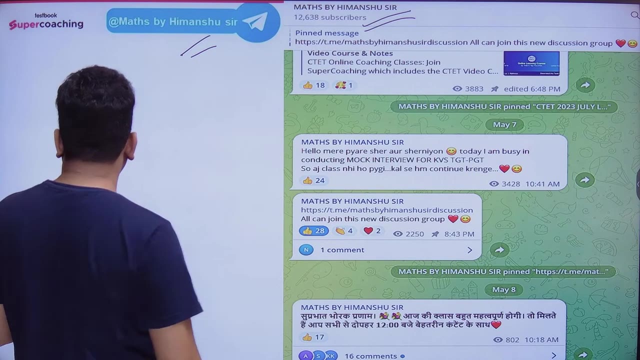 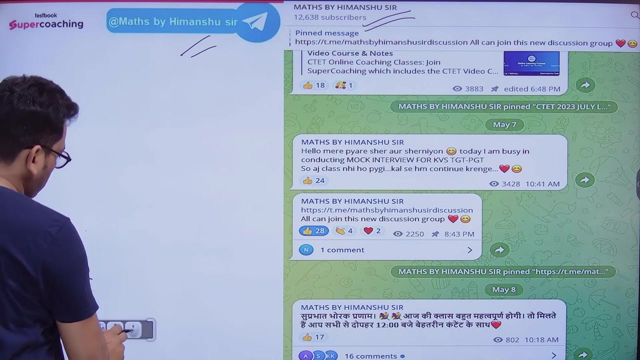 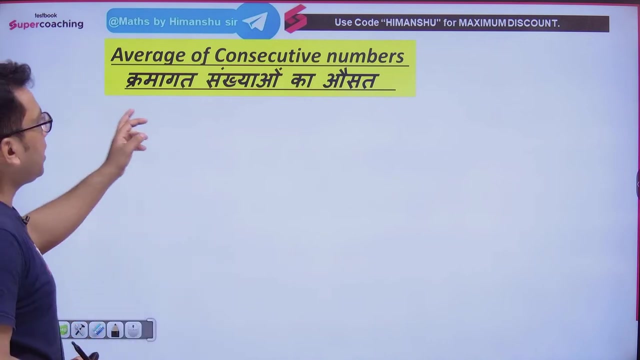 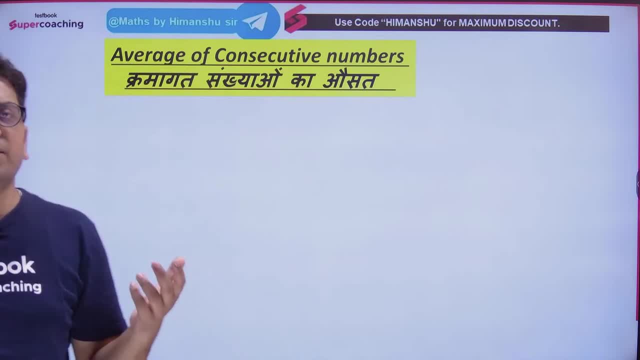 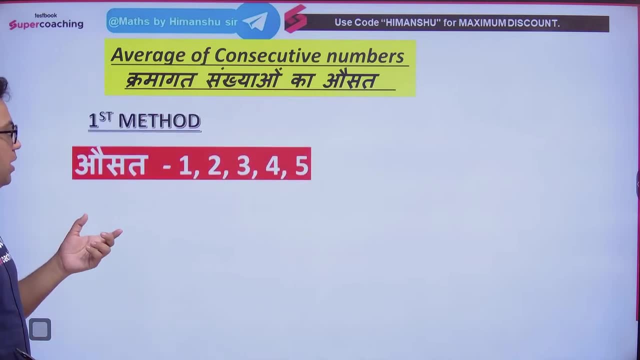 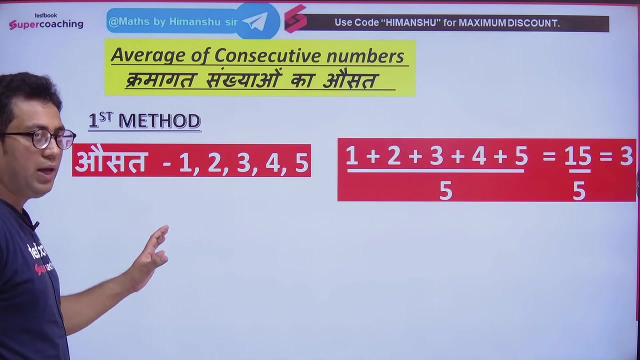 you must remember I told you in the last class that how do you calculate the average of consecutive numbers? suppose you have these numbers 1,2,3,4,5, so how will you calculate the average of these numbers? the first method is that we will join all of them. 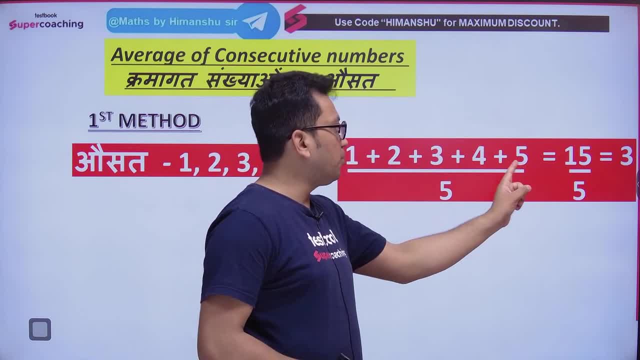 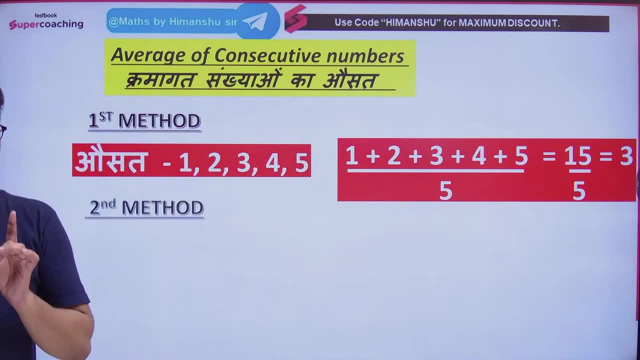 and we will separate the numbers from those numbers. so 15 divided by 5 is 3. that is the first method. the first method is to calculate the average. what was the second method? the second method was: when we calculate the average, the middle number, the middle number. 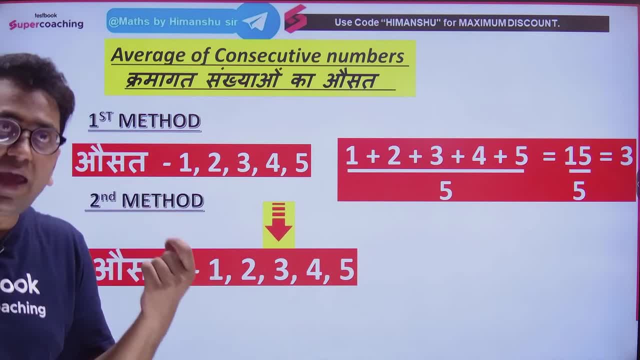 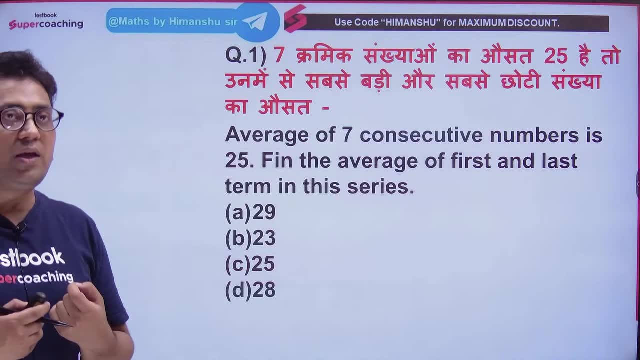 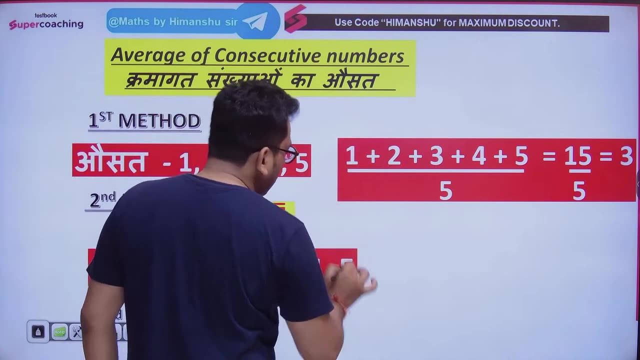 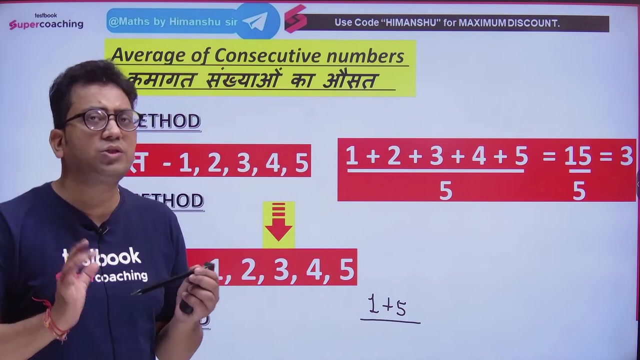 will be the average. it will be the average. the middle number will be the average. there is a third method. let me explain you. the third method says that if you join the first number, ie 1, and the last number, ie 5, what did I say? 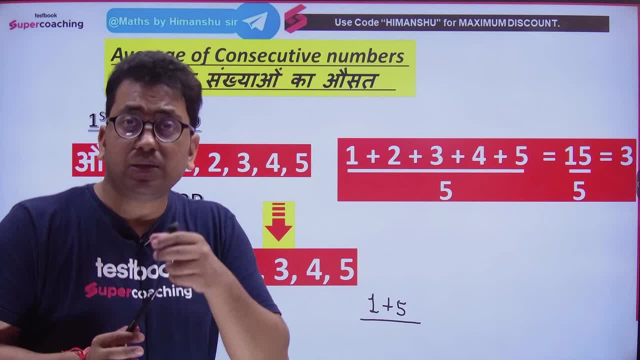 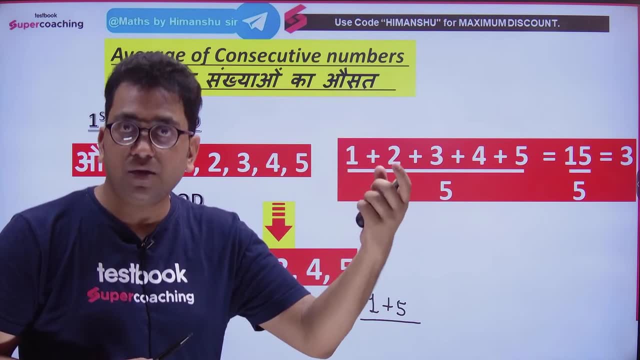 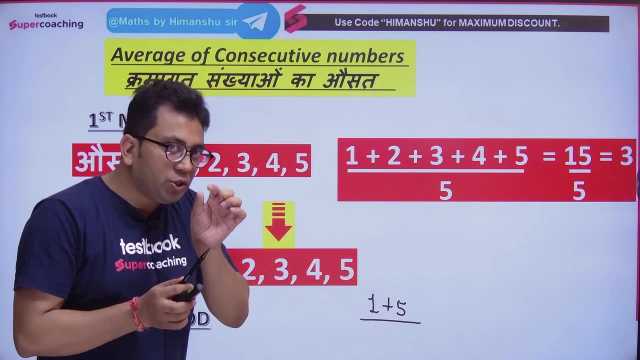 first number and last number here. the first number is the smallest, the last number will be the largest, ie the largest number. so what we are doing, we are joining the smallest number and the largest number. we are joining the smallest number and the largest number and we are separating it from 2. 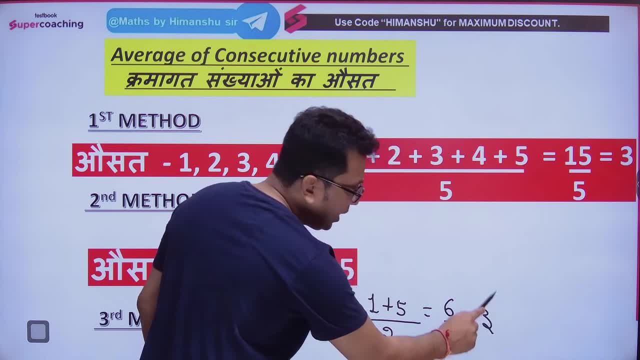 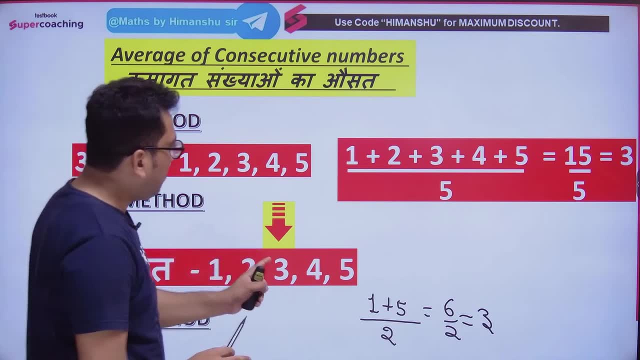 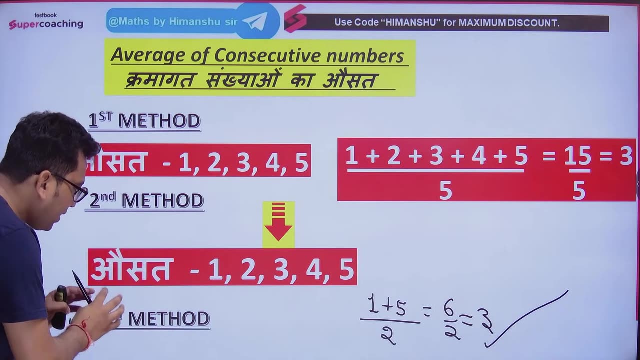 ie 6 divided by 2. so our answer will be 3, ie 3 will be the right answer. are you able to understand? so, in this way, what did we do? see? 3 only came and 3 was our middle. this is the third method. 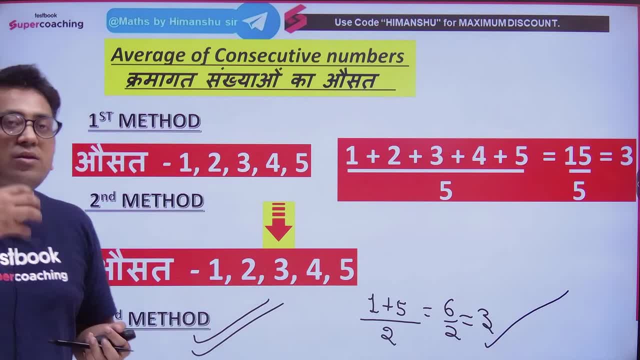 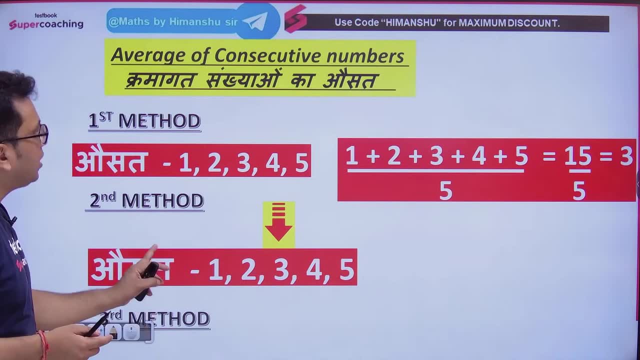 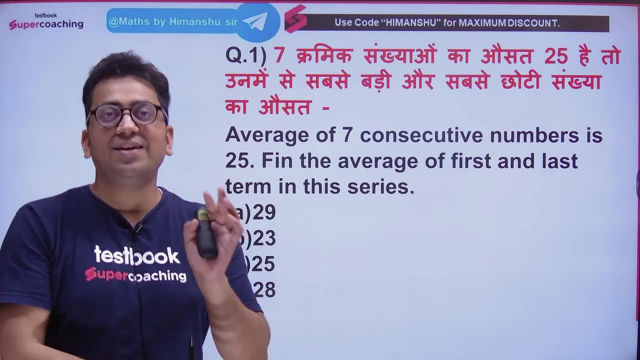 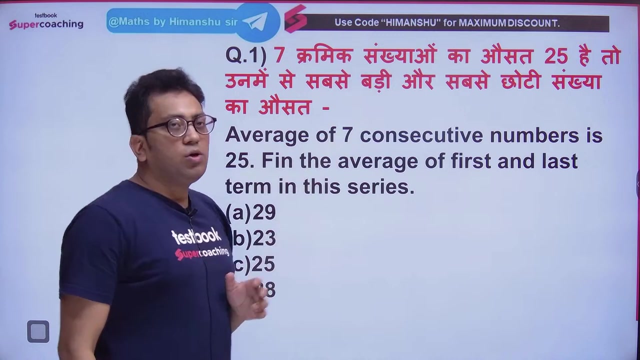 and now, based on this third method in our exam, how can we ask questions? we are going to think, so let's start the first, the last and the second, the next question. the first question of today's session is based on this concept: is based on this concept. 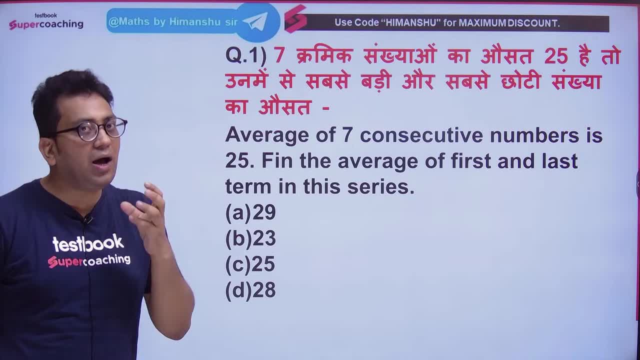 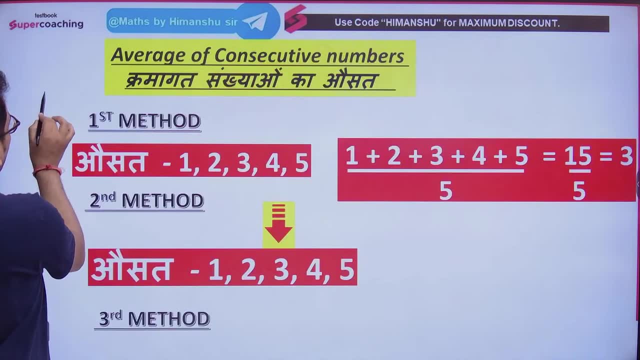 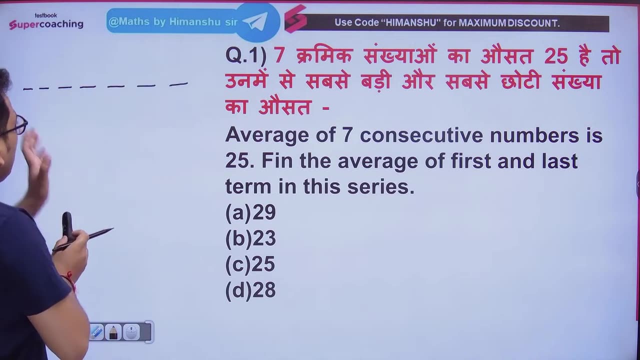 the average number of 7 is 25. so what will be the average of the largest and the smallest number of them? you said 1. you said in this way, 1,2,3,4,5,6,7, sir, if these are the regular numbers. 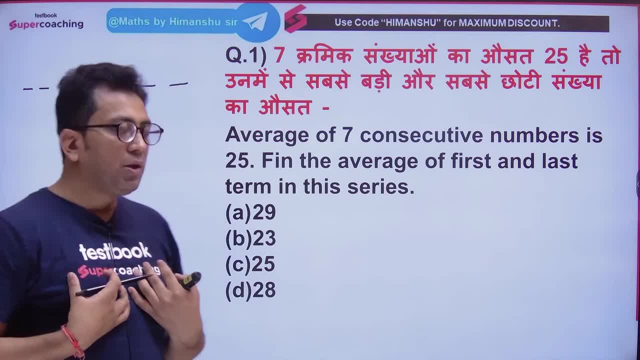 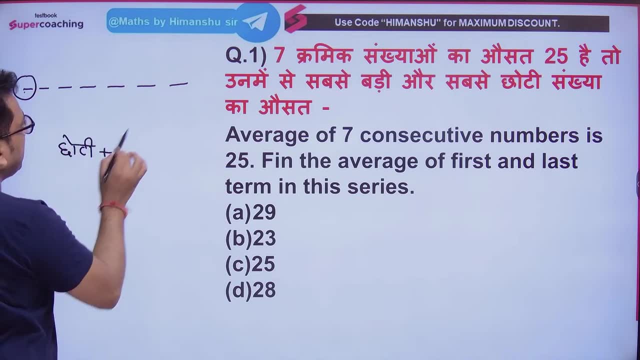 then we know the way to find the average. we will do the first number, ie the smallest number in the sum. the last number, ie the largest number, we will join both and separate it from 2, so we will get the average how much he has given. 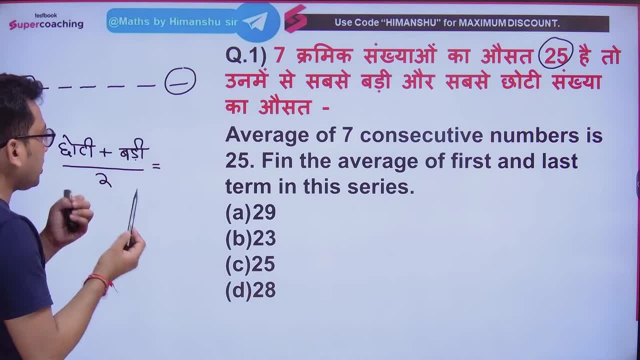 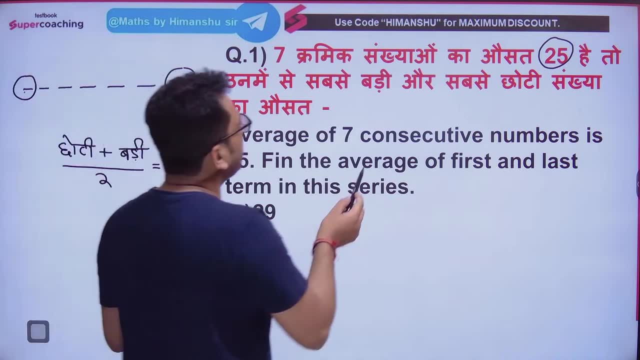 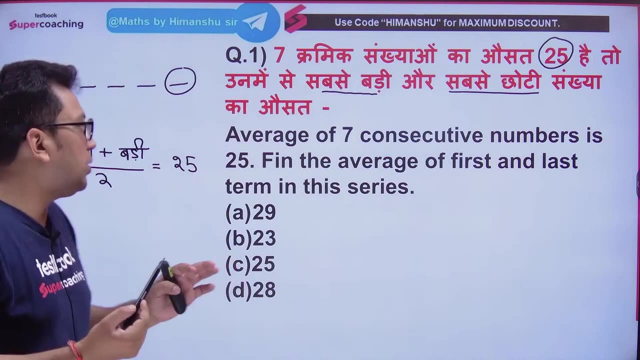 he has given 25. ie, if I solve it, how much will it be? it will be 25. we can find the average, he asked us. he said: tell me the average of the largest and the smallest. tell me, if we have to find the average. 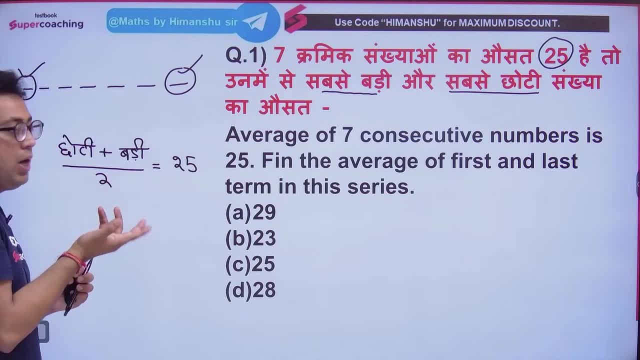 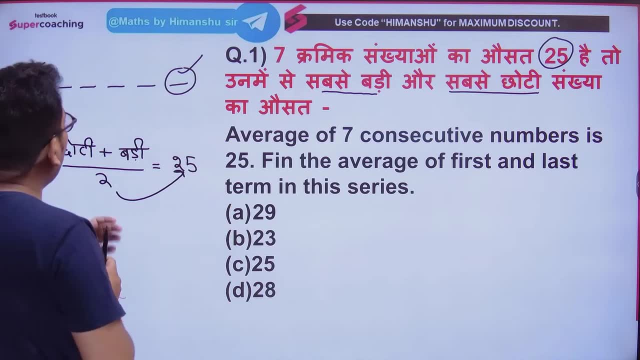 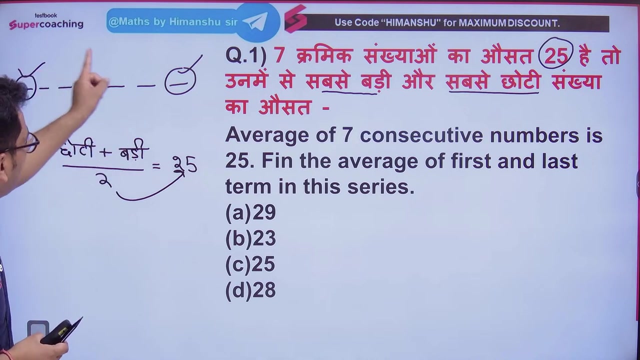 of two numbers. how will you find it, sir? it will be equal to 25. yes, so now? the concept is that, sir, if we have a formula, a series of consecutive numbers, a formula, then our average of that formula will be equal to the average of the smallest. 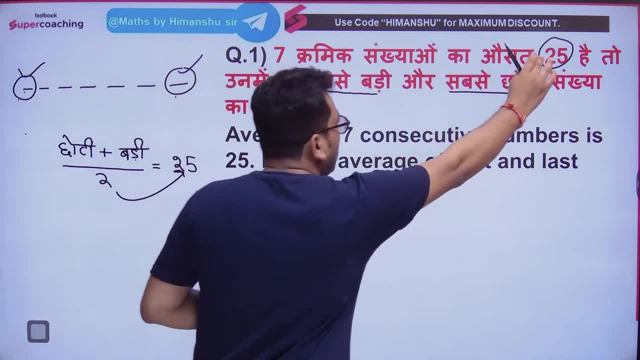 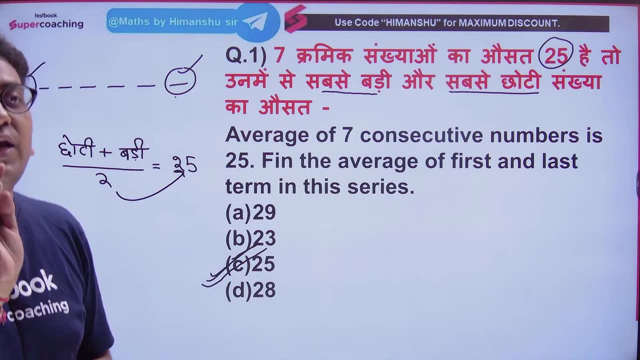 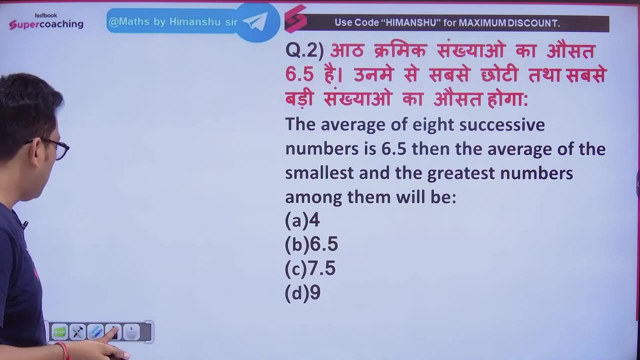 and the largest number. so if the average in the question is 25, then what will we get? the answer: we don't have to solve. we don't have to solve. do you understand? if you don't understand, then why are you worried? next question, question no.2. 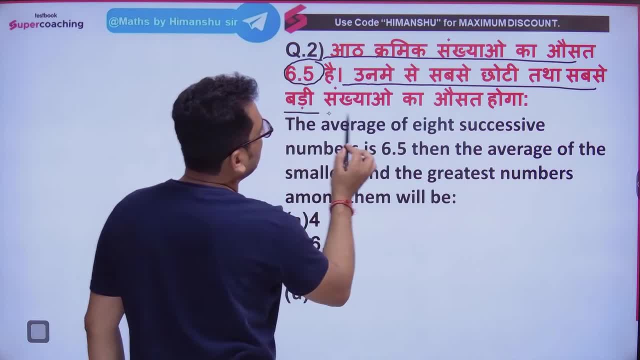 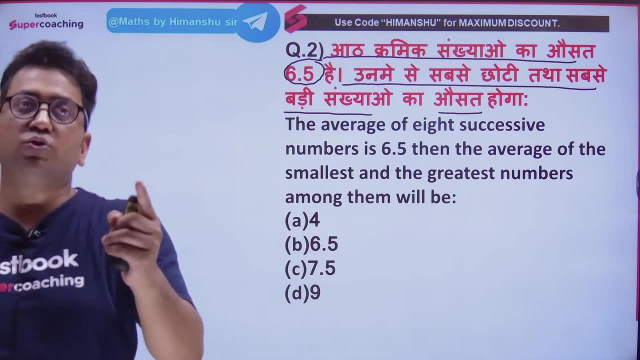 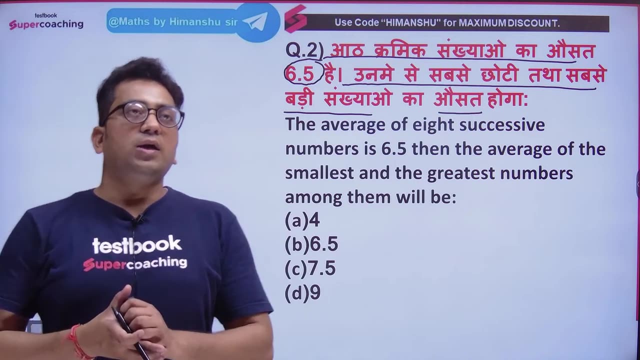 the average of 8 consecutive numbers is 6.5. so what will be the average of the smallest and the largest? you have to tell. I would like every child who is watching this session to answer this question. here I can see SinkiSumanAnjali. 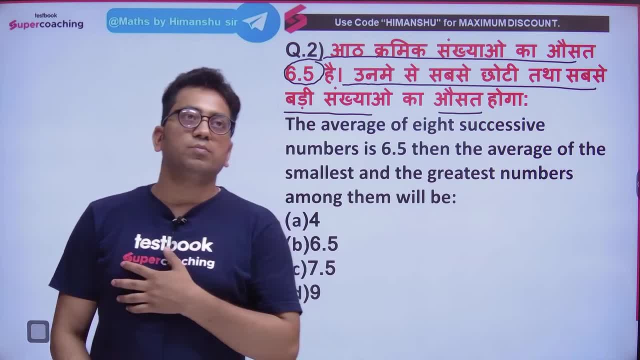 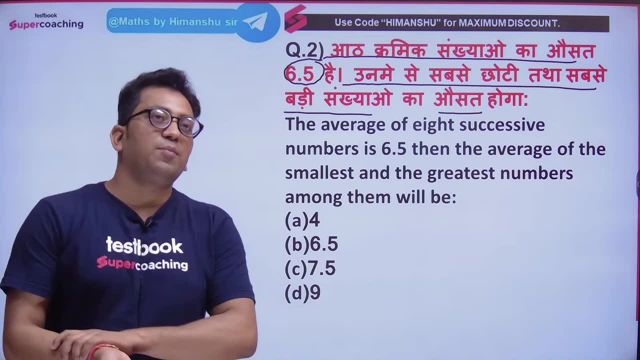 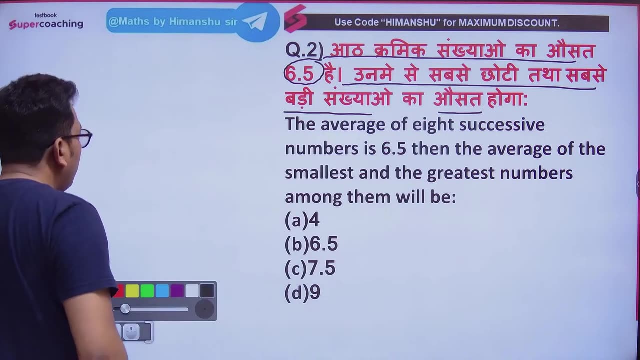 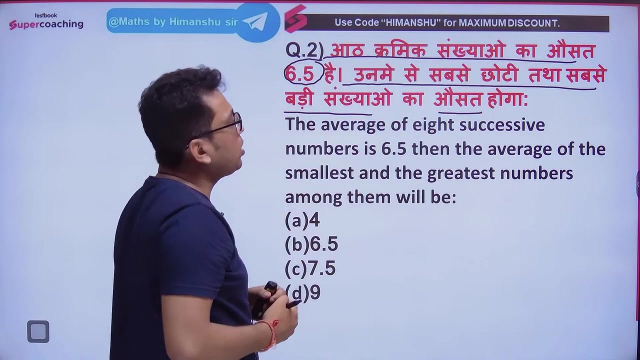 AkanshaBabita Shubham. very well, everyone, Nahid, while setting the reminder, like it. thank you very much. let's answer all 6.5. answer very simple: 8 consecutive numbers. then the ratio of the smallest and the largest number in it will be the ratio of the same. 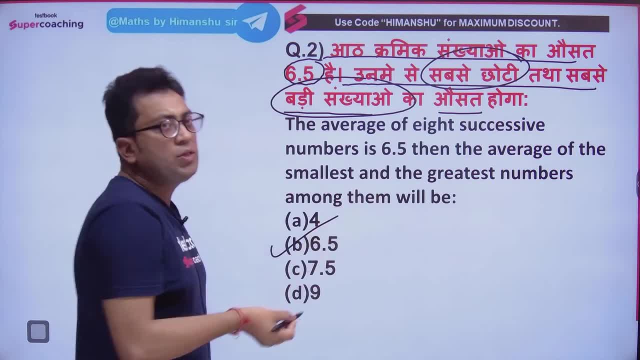 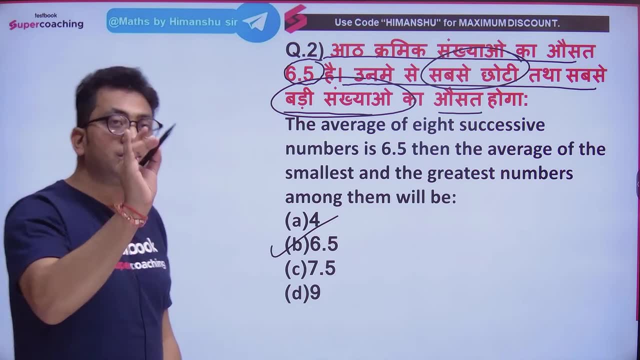 number. That is, if it is six and a half, then it will also be six and a half, Right, There is no solution. Mark 6.5 answers. Understand the concept of the questions and answer them. The next question is coming in front of you. 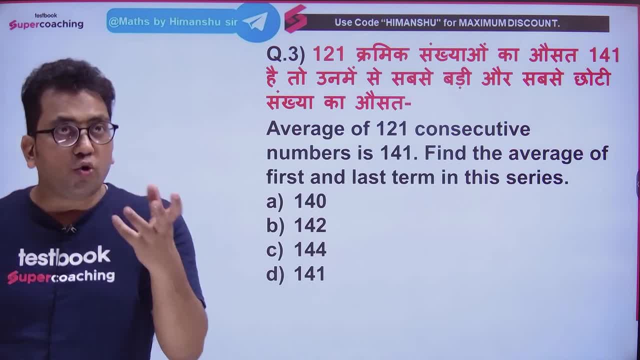 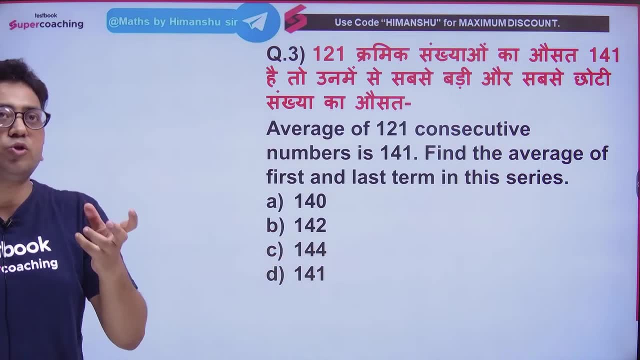 Here is the next question. Answer it quickly. Understand the question. The ratio of the number 121 is 141.. So tell me what will be the ratio of the largest and smallest number. Okay, let's see how many children are able to answer. 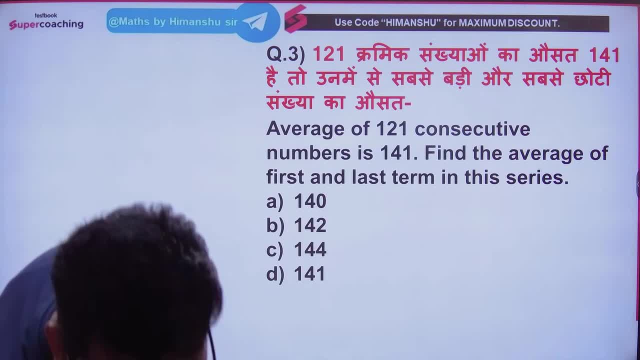 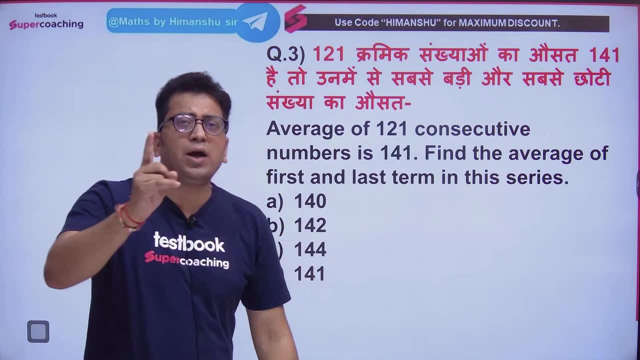 Answer all of them. Come on, son, with speed, with speed. Today I have brought a very amazing concept for you. I will teach in this way. I guarantee that no one has ever taught you in this way. Okay, there are other things to come. 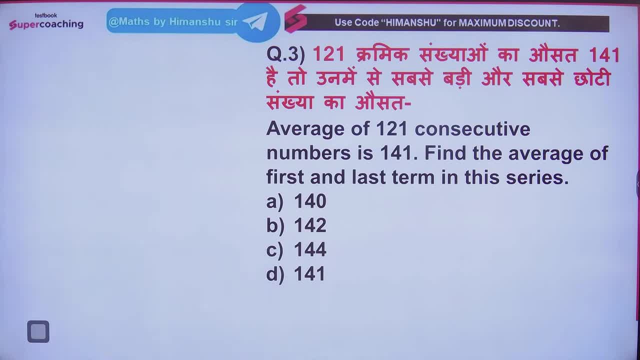 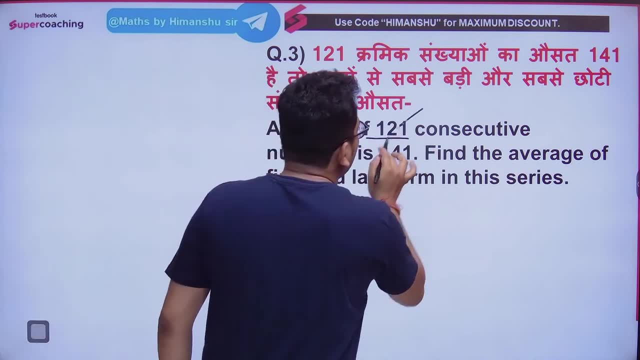 These are very nice things, son. Come on son, Very good, 141.. So you are answering 141.. Sir, how manyAB numbers are there? 121.. What does this mean? Does not mean anything, Sir. we do not mean any numbers. 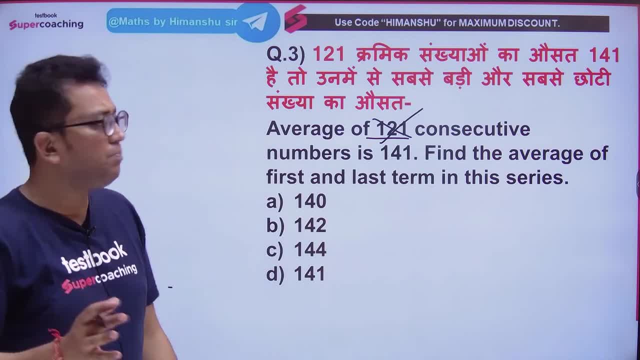 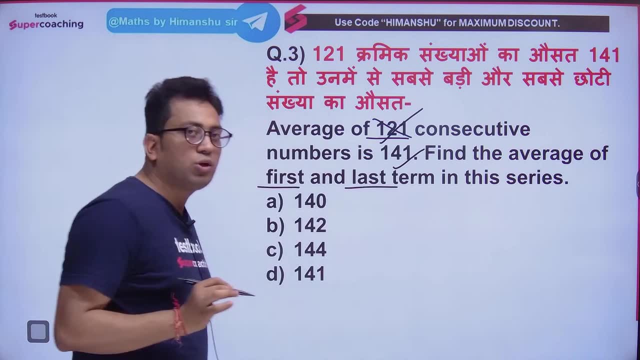 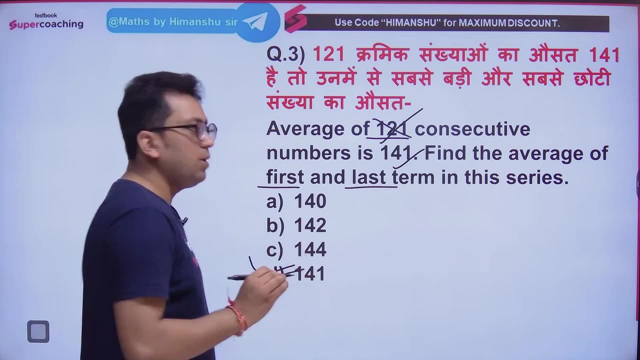 We are just concerned with the ratio. How much is the ratio 141.. And if this is a series of consecutive numbers, then the ratio of the first and last number will also be the same. That is, our answer of 141 is going to be D will be the right answer. 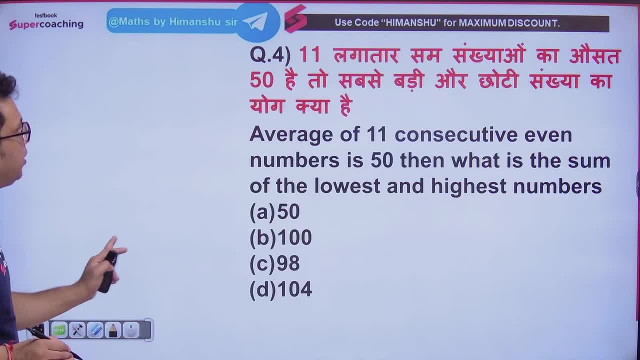 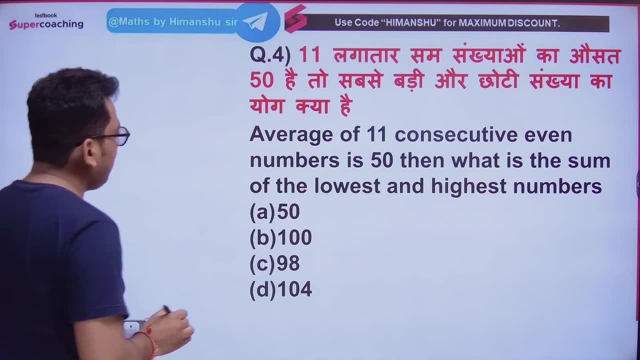 Next question. The next question is coming in front of you, question number 4, quickly, carefully, understand it easily. tell me what the answer will be. the question is in front of you. let's set the timer for all of you here, just 20 seconds. come on, tell me quickly what the answer will be. 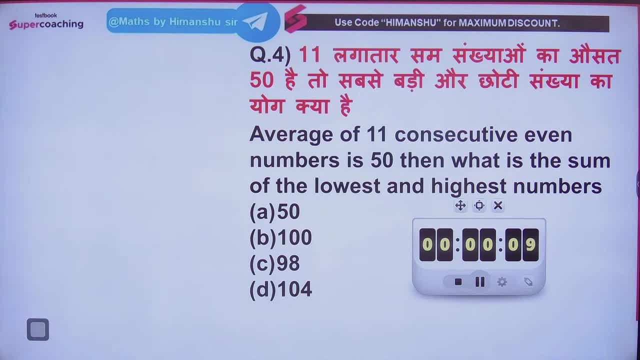 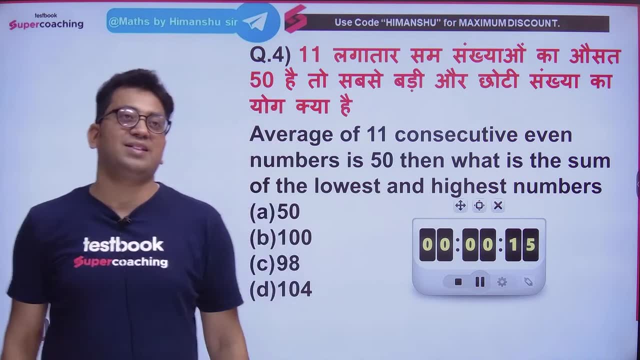 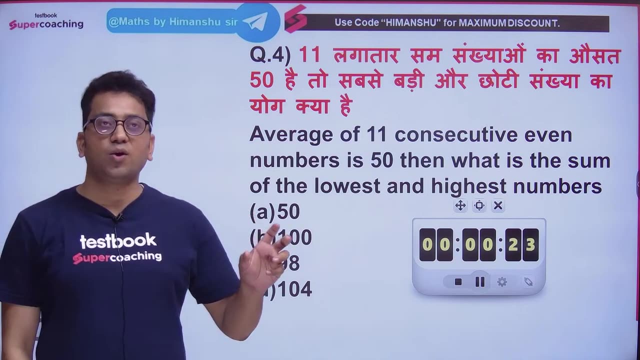 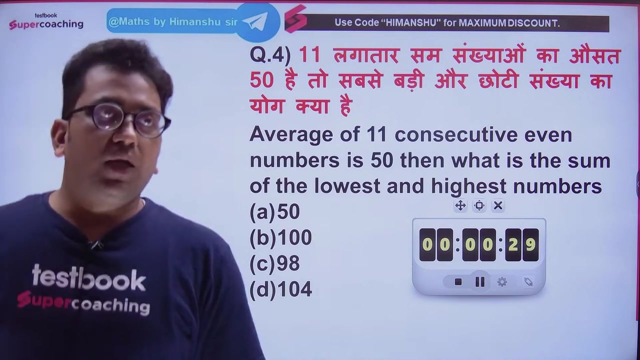 A child is saying he is preparing for SSC. maybe he is saying, sir, he can work in SSC, son, he can work anywhere. he can work anywhere we are teaching you in this way. you are giving any exam of India. he will work everywhere. okay, why won't he work, son? come on, fly the question. tell me quickly what the answer will be very good, very great. now look at this. 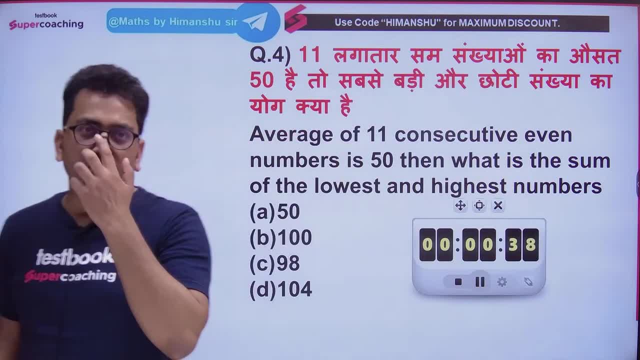 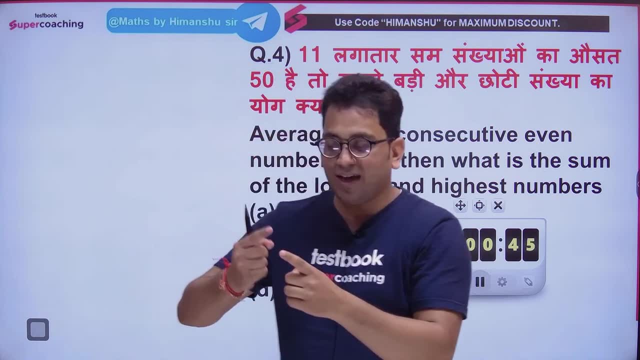 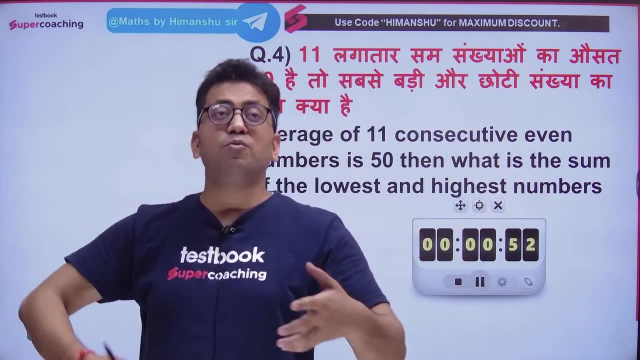 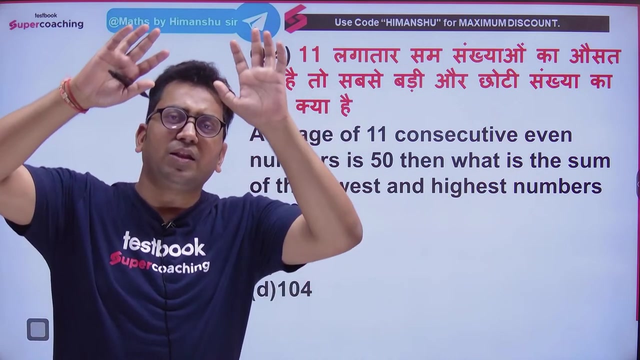 childhood. we used to play games. son, we used to play games in childhood. the bird flew. we were young, we were young. so, brother, brother, no, no, yes, the bird flew. the pigeon flew, the buffalo flew. I used to do it in my childhood, but we haven't changed yet, we haven't changed our mistakes yet, son, and we just flow in emotions. brother, the bird flew, the pigeon flew, the buffalo flew. the buffalo also flew, hubby, he flew in my environment. we have spread in emotions. we have gone there. we have not remained here. we have gone to六 religion, alayka thang. we have become a strange Robin. everyone has taken his Muse. we have removed all powers. we have quiet. radicals have taken our delusions. 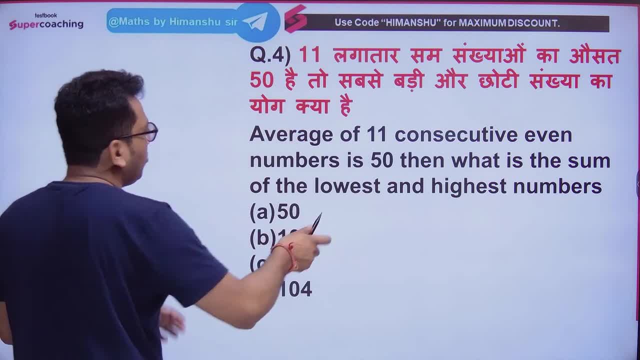 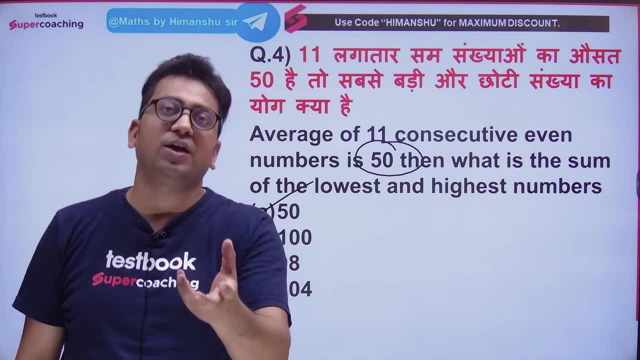 Sir, he said that the value is 50, so he looked here and there and answered that the value is 50.. Son, look at it and ask what it is, otherwise there will be an accident. there will be an accident. Sir, understand what he is saying. he is saying that the value of 11 continuous odd numbers is 50.. 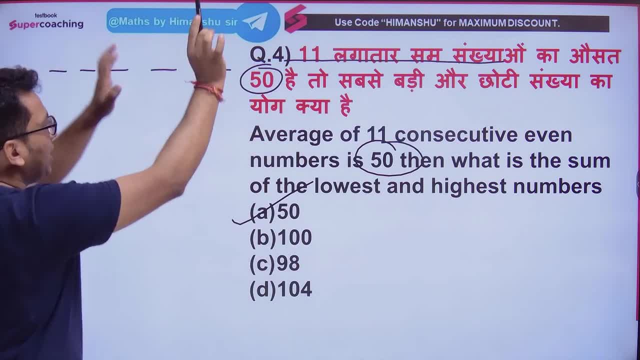 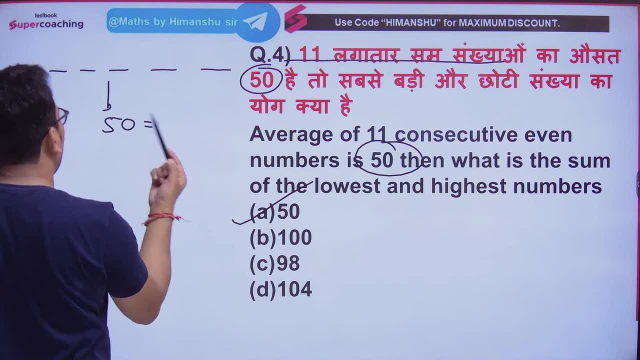 Okay, there are 11 continuous odd numbers. there are continuous odd numbers, so the value is 50. only, Sir, who will be equal to 50?? The same thing, sir. do the sum of the smallest and the largest and run away from 2.. 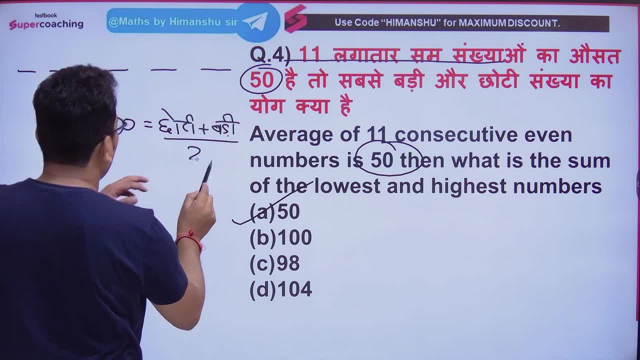 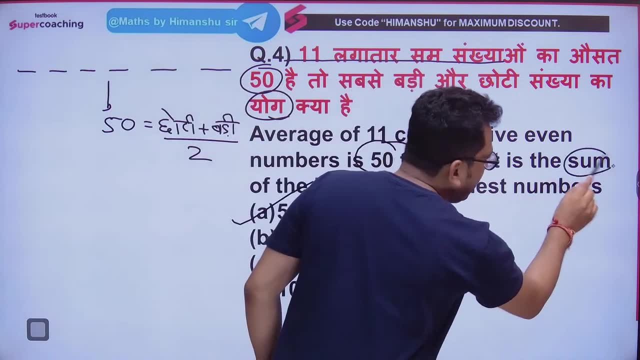 Absolutely right, sir. So it will be equal to this. Did he ask you the value this time? No, brother, he asked the sum of the largest and smallest. So, my son, you will get the sum of the largest and smallest, right. 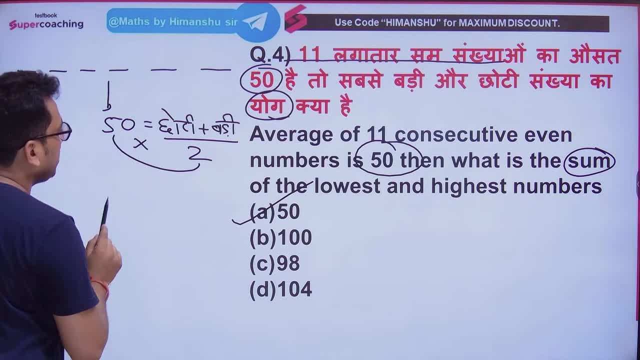 So, brother, multiply 50 by 2,, that is, 2 will be multiplied here. so the answer will be 100.. Do you understand? If you are understanding something, then my son, it will not be 50,. what will be the answer? 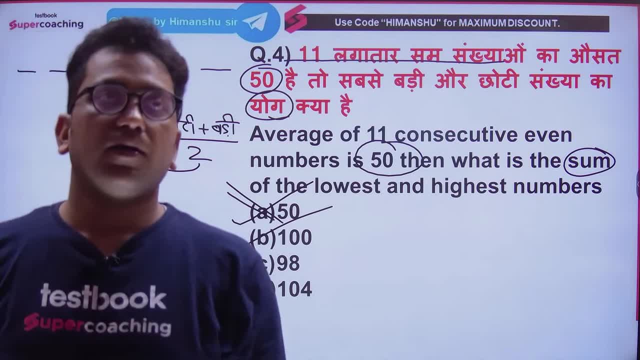 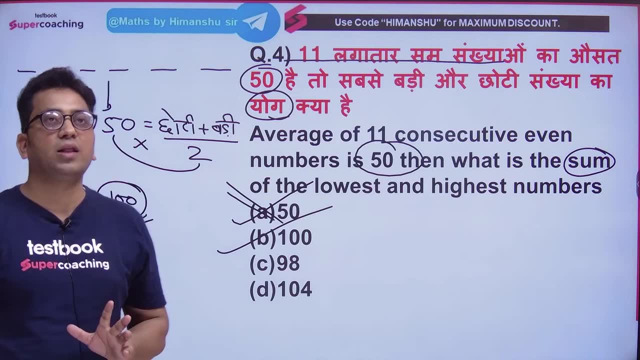 100, that is, 100 is our answer. Tell me, Chamka, are you understanding? So the answer based on what is asked. you do not have to multiply things. keep multiplying. Yes, this is how the work is done. 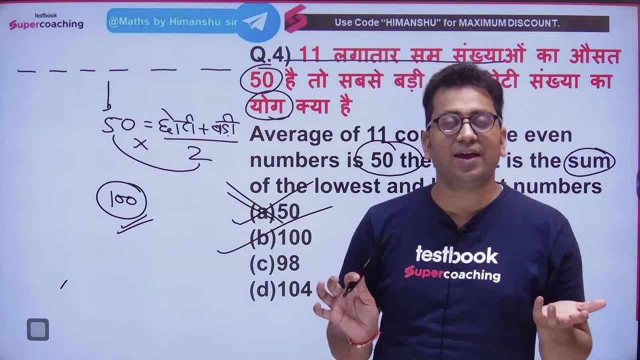 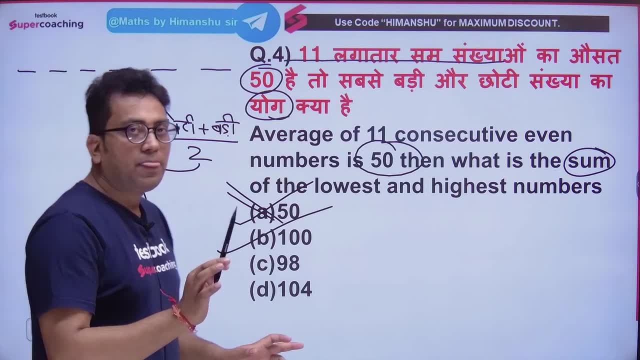 Hey, is it multiplied in math and mathematics? It is understood and the questions are answered by understanding. right? That is the concept. from here is Chamka, that if, If you ask the value, then the value you have given above will be the value of the largest and smallest. 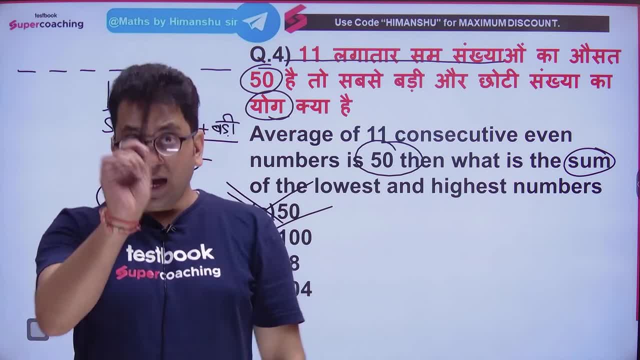 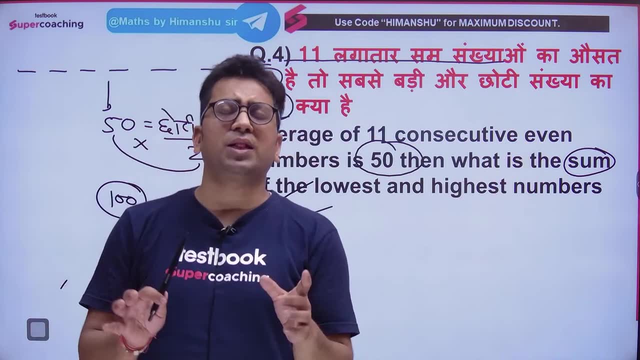 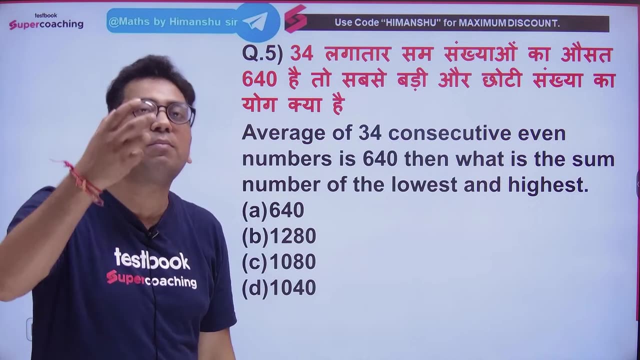 But if you ask the appropriate result, then we will double it. if it is consecutive, that is consecutive, Then whether it is even or odd, whatever it is, we do not care about it. it should be continuous. There should be a sequence where the differences between the columns are equal. the difference is the same. 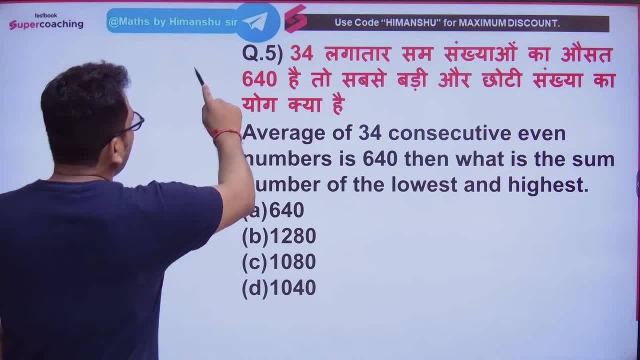 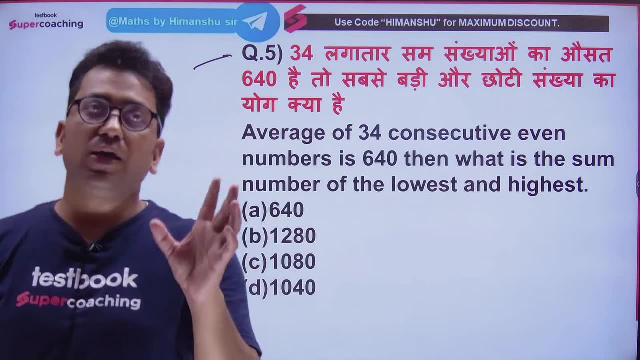 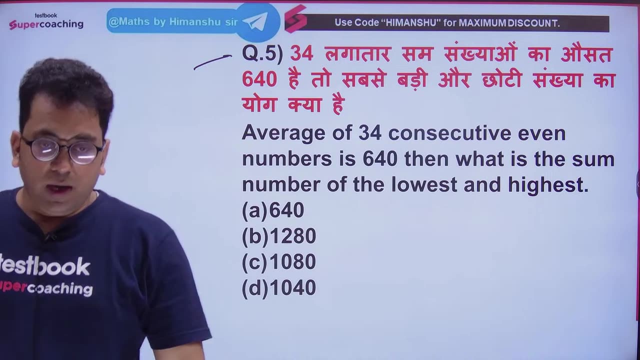 Next question, Question number 5.. Question number 5.. We have come to the fifth question. If the average of all numbers is 644 continuously, then what will be the appropriate result of the largest and smallest? Come on, Yes, son, answer quickly, with speed. 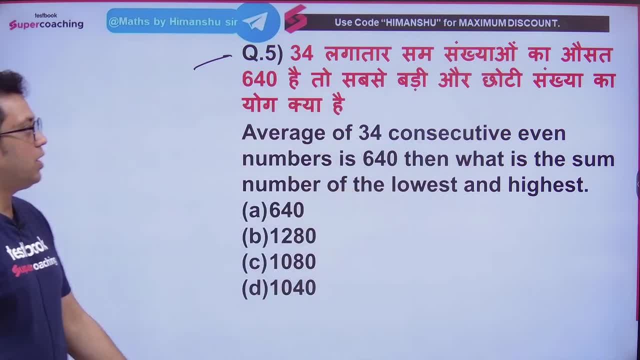 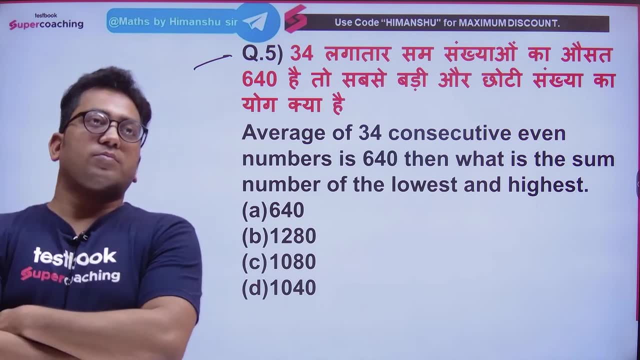 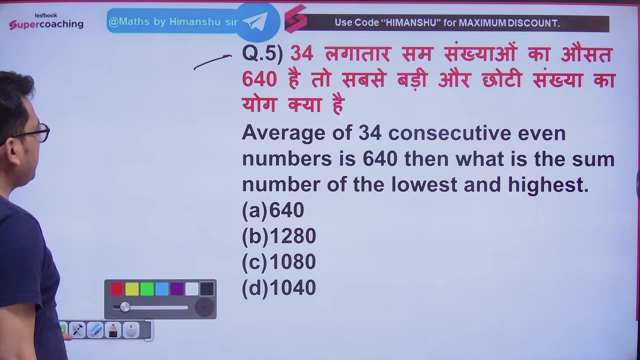 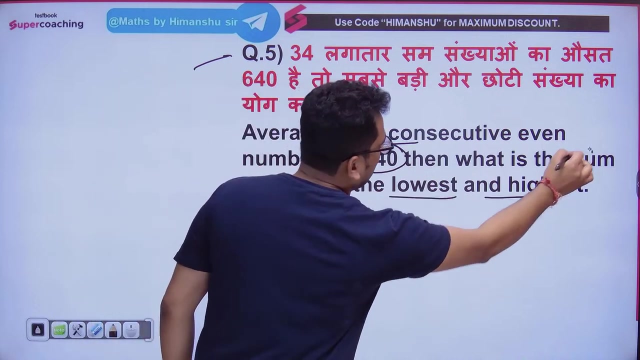 If the average of all numbers is 644 continuously, then what will be the appropriate result of the largest and smallest? Look, we are telling you that the average of all numbers is 644.. We are telling you that the appropriate result of the largest and smallest is asked. 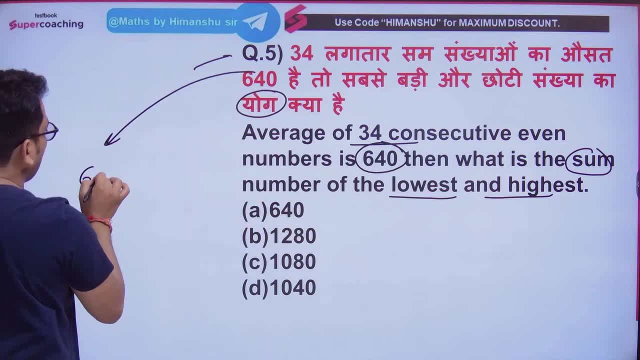 What is the appropriate result? So our child will directly pick up 640 and beat it by multiplying it by 2 and will say that your answer is 1280.. Is it or not? So B is our answer, brother. There is no need to think. 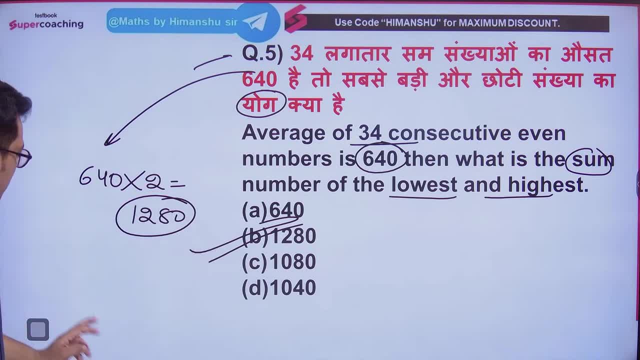 There is no need to think So our answer will be 1280.. Very good, Very good, Okay. Next question, Question number 6, is in front of you. Shine quickly, Tell me what the answer will be. Answer with speed. 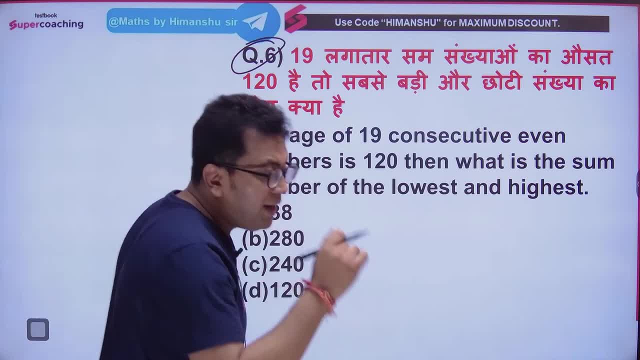 Okay, Son, this is a very important part of elementary math. From here, the question can be asked in your exam. Tell me quickly what the answer will be. All of you, Let's fly, Let's shine, Let's fly. 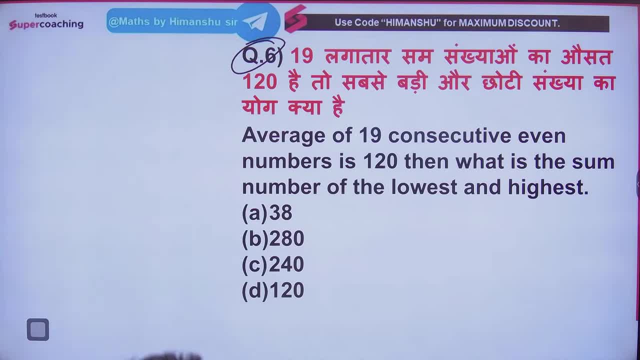 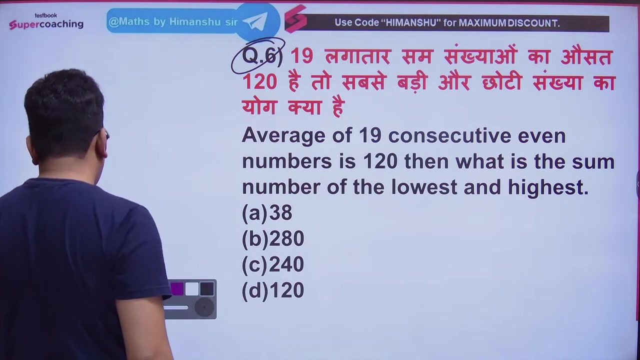 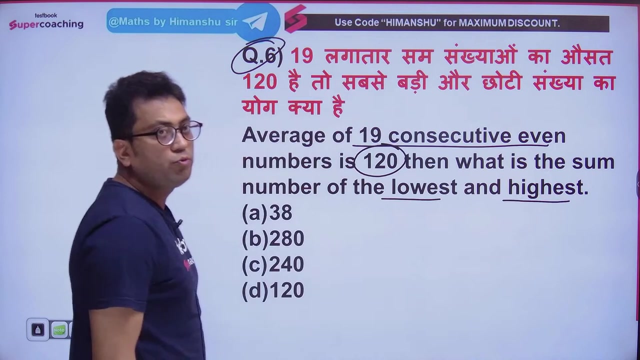 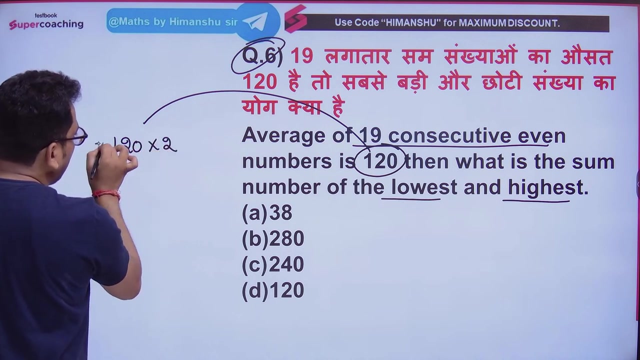 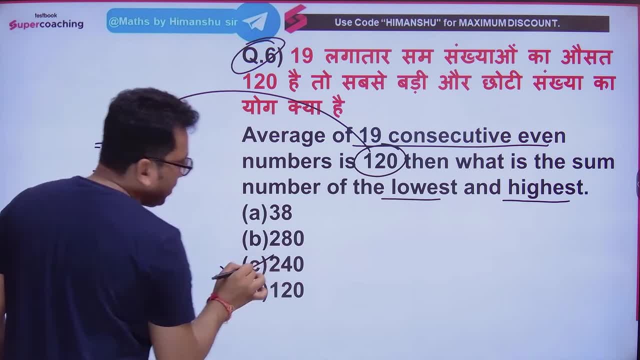 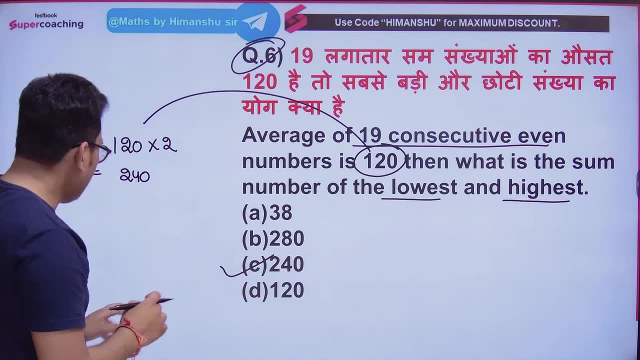 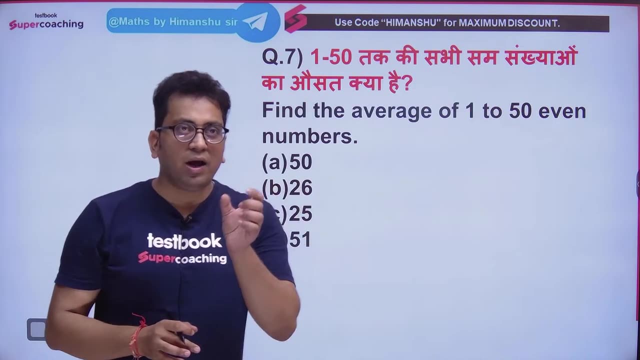 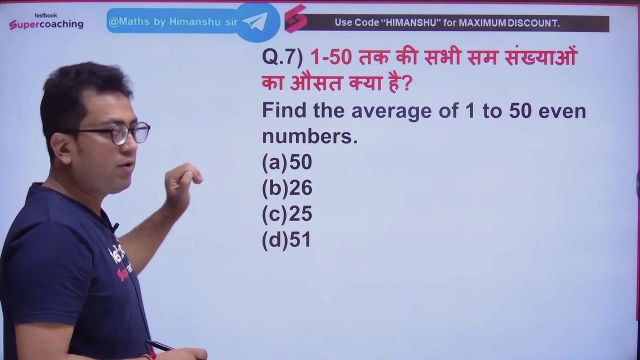 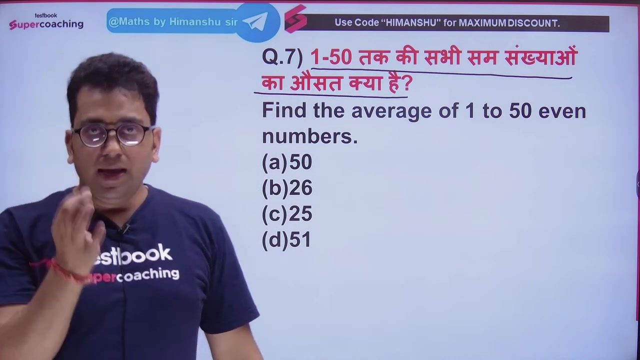 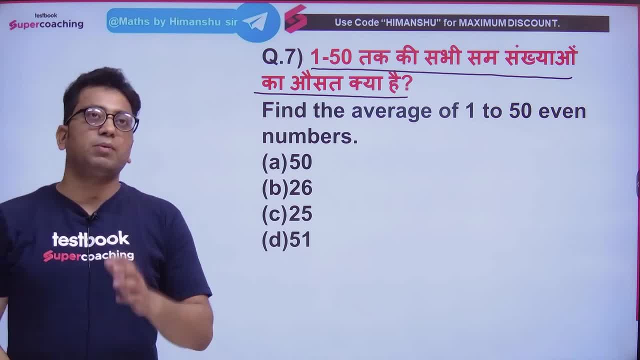 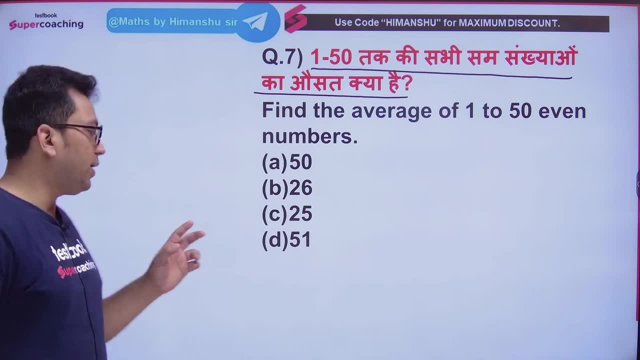 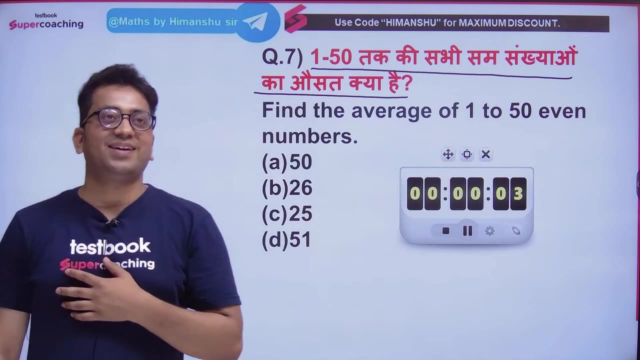 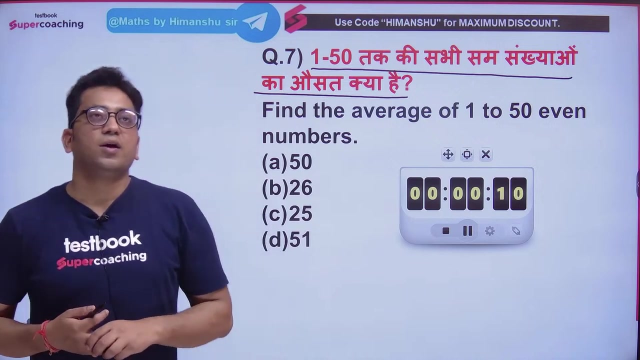 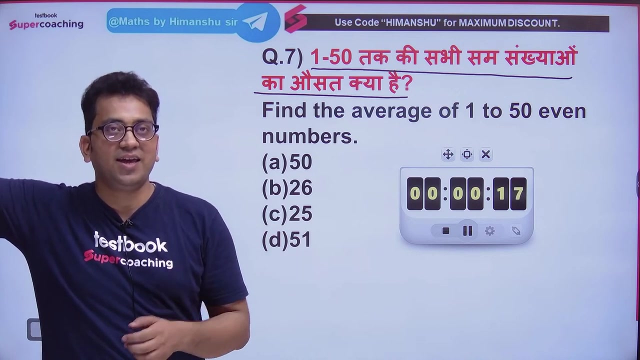 what will be the ratio of all natural numbers from 1 to 50,? what will be the ratio of all natural numbers from 1 to 50, cheek, Why won't he ask? We have written big on the rail. he will ask, and where will he ask? 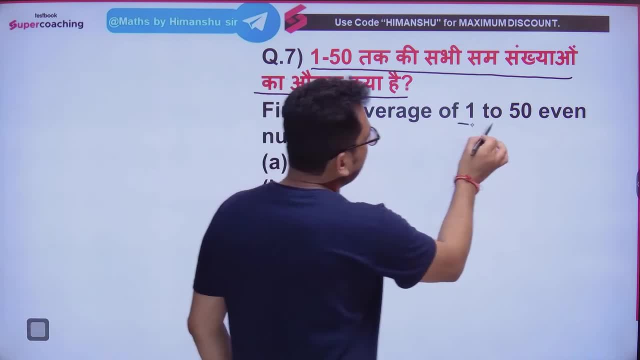 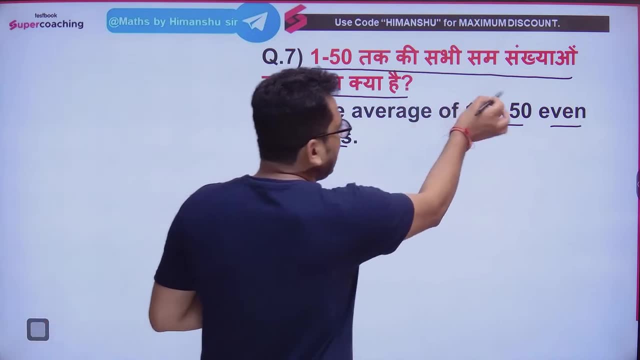 Come on, see what he is saying to you. We have to tell the ratio of all numbers from 1 to 50. Now tell me what are these all numbers in 1 to 50? And what is the difference in all numbers? 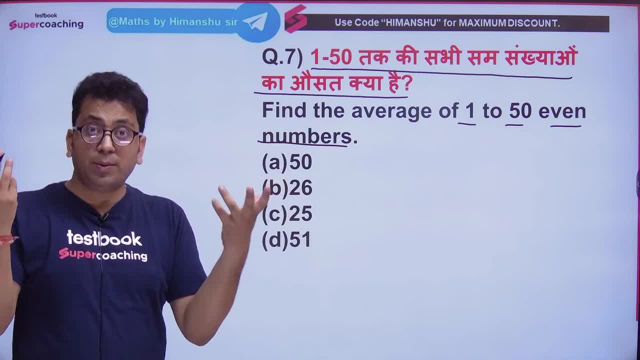 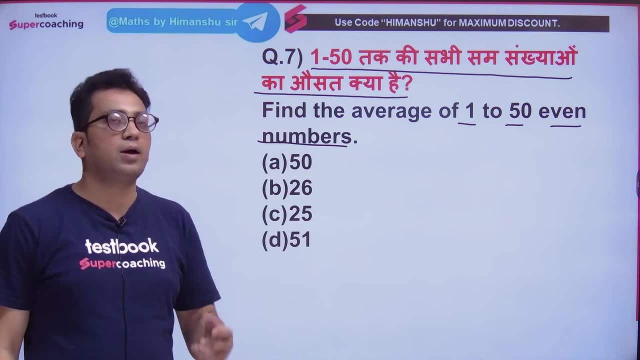 There is a difference of 2: 2.. If the difference in all numbers is equal, then the concept will remain the same. We will divide the smallest and the largest by 2.. Sir, what will be the smallest number here? 2.. 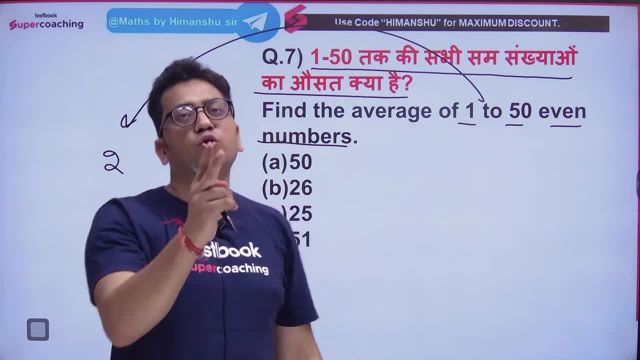 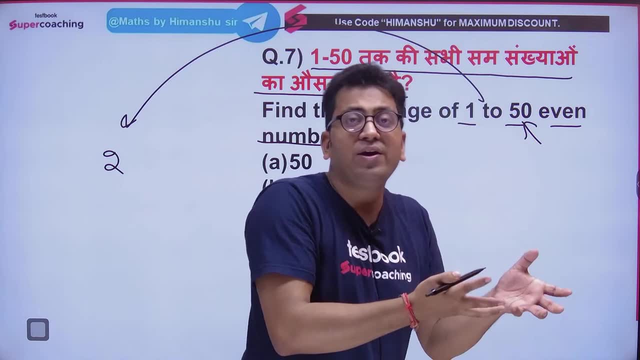 It is starting from 1,, so the first one will be 2.. The last one will be 50.. Because in 1 to 50, 50 is even. It is the last even number, So the last one will be 50.. 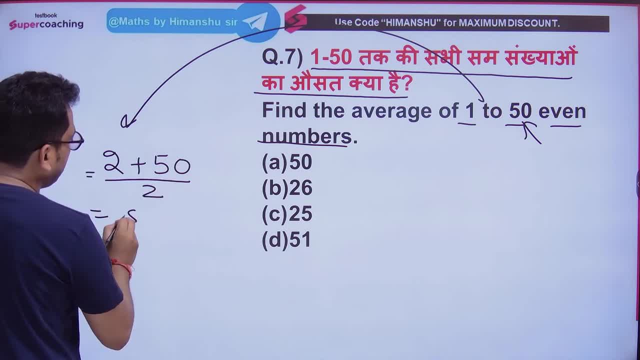 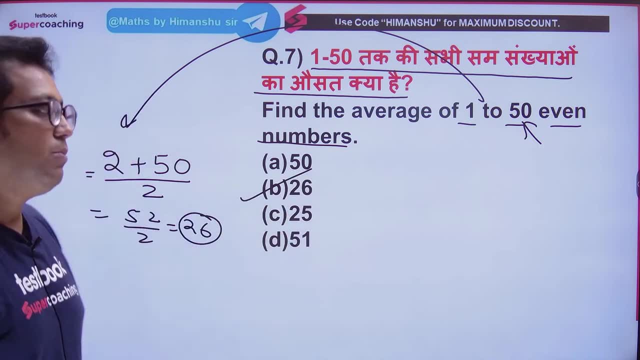 We will add both and divide by 2.. The ratio of 52 to 50.. 26 will be our answer. Say yes, 26 will be the right answer. Is it clear? Is it shining or not shining? 26 will be our answer. 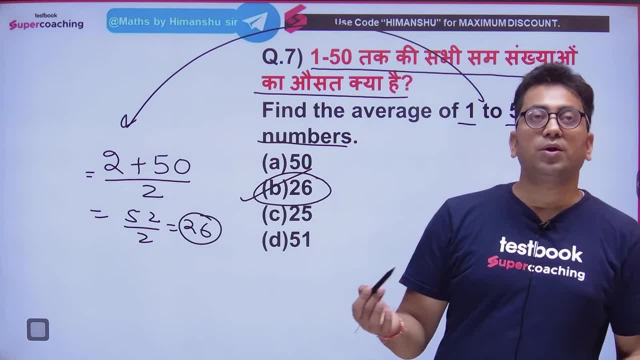 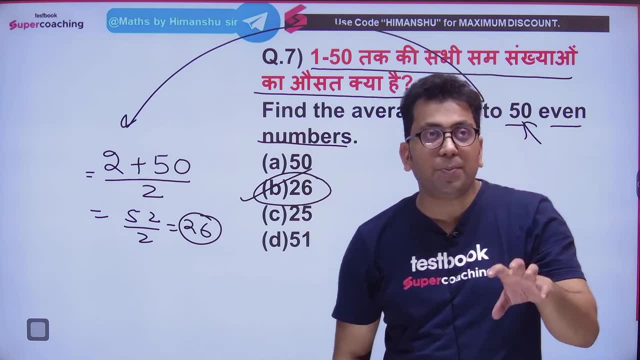 Okay, There is no retina Answer with the concept. What I say is that you will always keep the concept in mind in the exam And the ways I tell you to shine are based on the concept. The next question is coming in front of you. 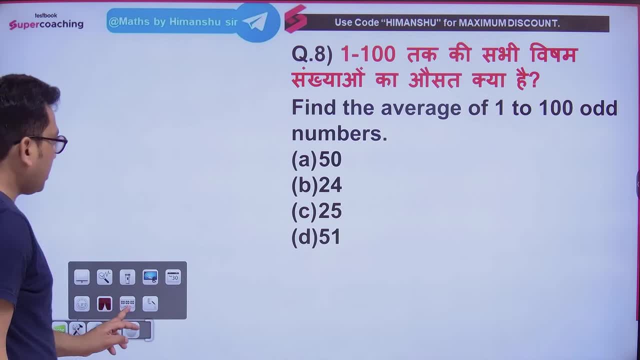 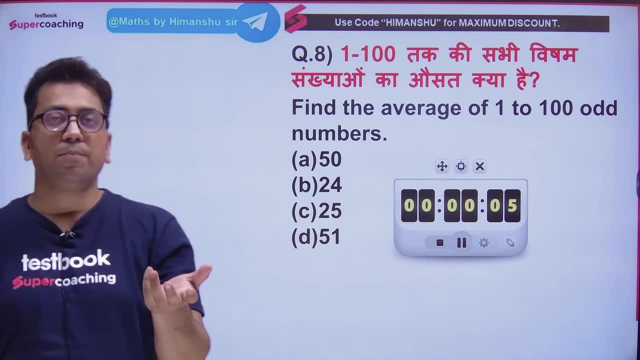 Tell me quickly what will be the answer. Question number 8.. Try it: 1 to 100.. All This time I did not say sum, This time I said retina. That will be the concept, Because there is a difference of 2 in the retina. 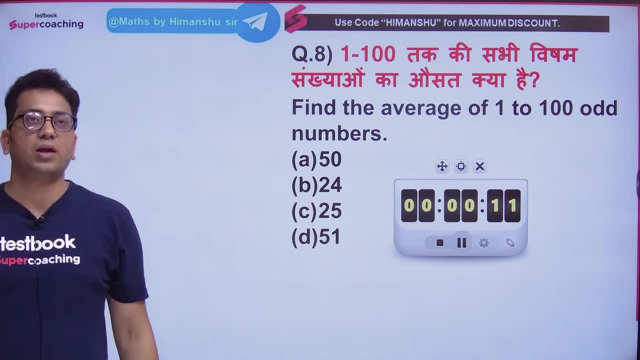 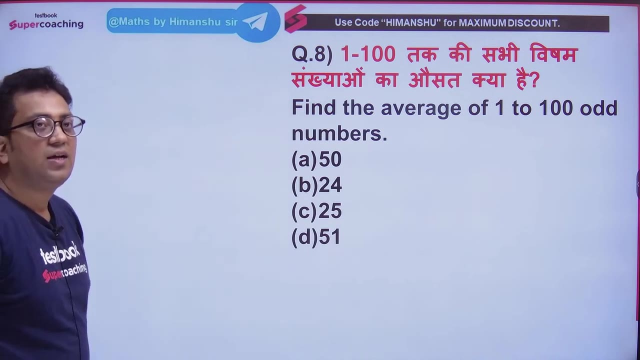 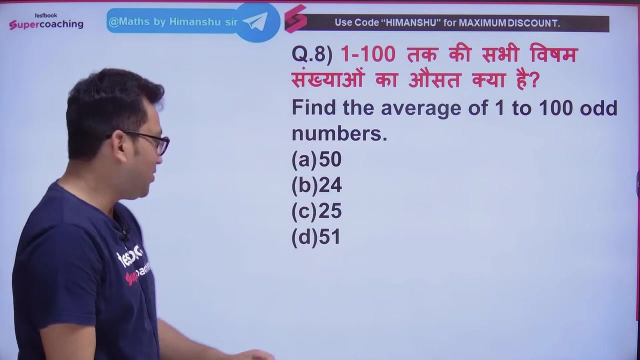 There is a part where the difference is equal. Tell me quickly what will be the answer. Yes, What are you saying, kid? If there is an odd number, Then give the odd number. Why do you get worried? There is no little patience. 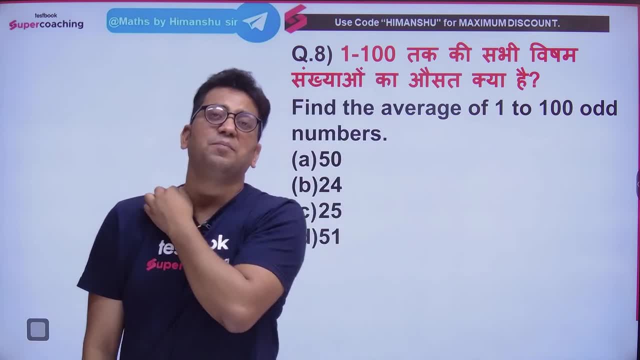 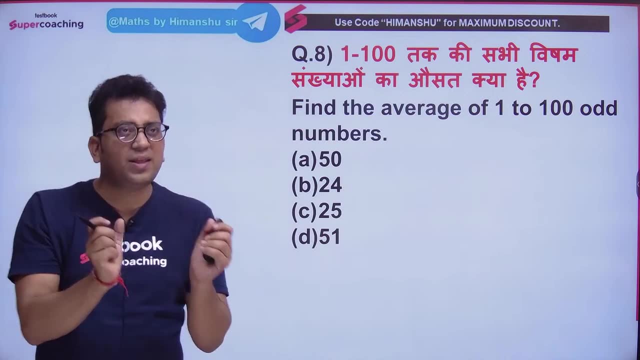 Nowadays, there is no such thing as patience in today's world. You gave the question of one even and gave the next odd. Then you are not understanding the concept. You are paying attention to the even odd, Don't pay attention to the even odd. 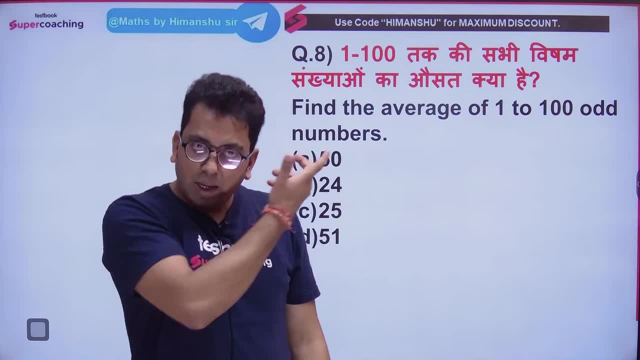 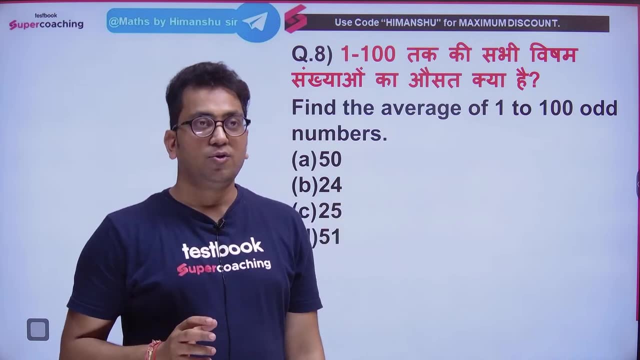 Pay attention to the concept. There should be a difference. Now, this can also happen. There may not be an even odd, There may be something else, But if there is a difference between the lines, then this concept will remain. Keep it slow, son. 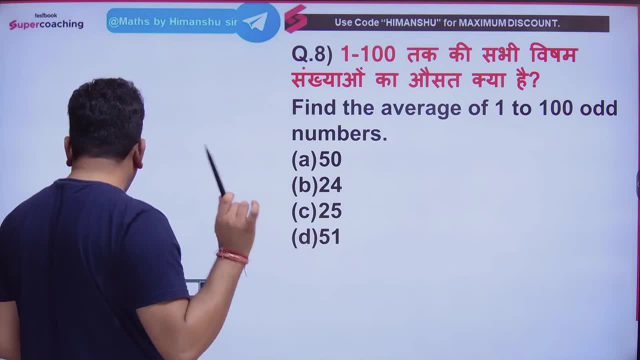 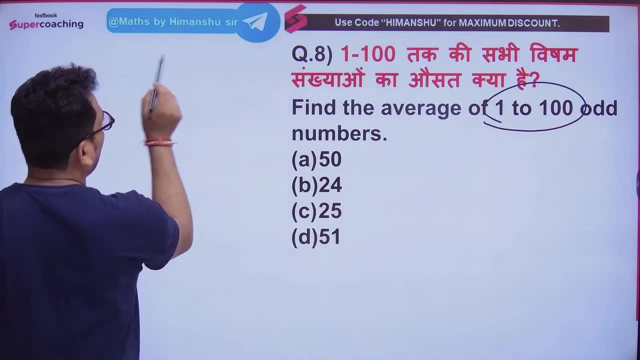 Isn't it? Tell Dheeraj? Call Dheeraj at home by phone. Tell him that we have less. You also come. So we are talking about 1 to 100.. So tell me What will be the smallest number. 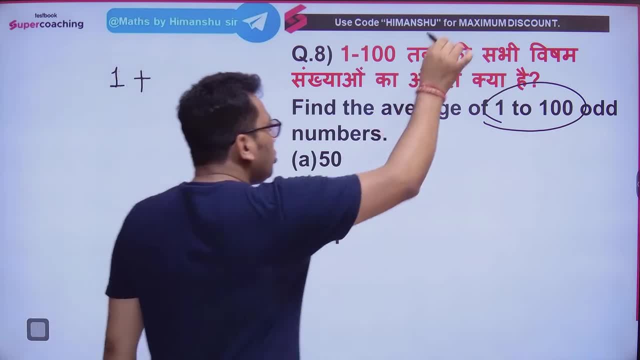 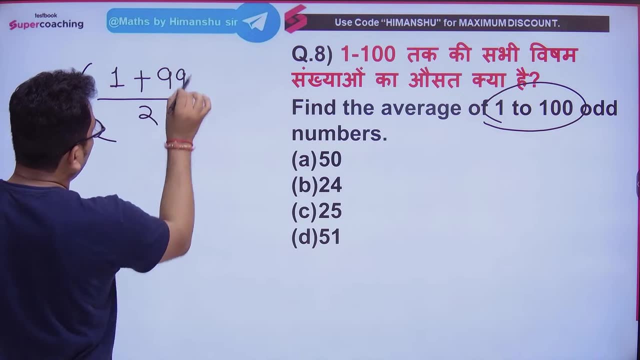 It will be 1., Which is not divided by 2.. And in 100, the last number is going to be 99. So we will add both, We will divide by 2.. Our answer will come: 100 divided by 2.. 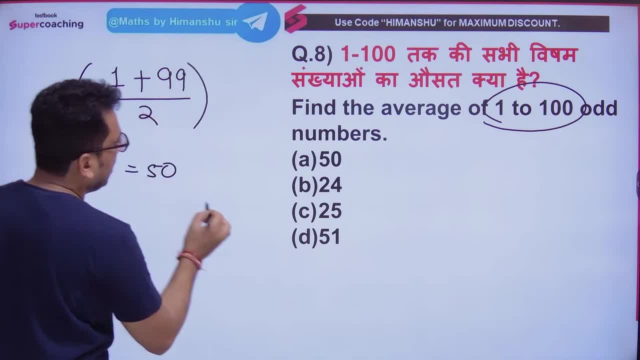 That is 50.. Our answer will come. 50 will be the right answer. Tell me Chamka, Every child will have a right answer. Yes, Our answer will be 50.. Do you understand the child? 50 will be our answer. 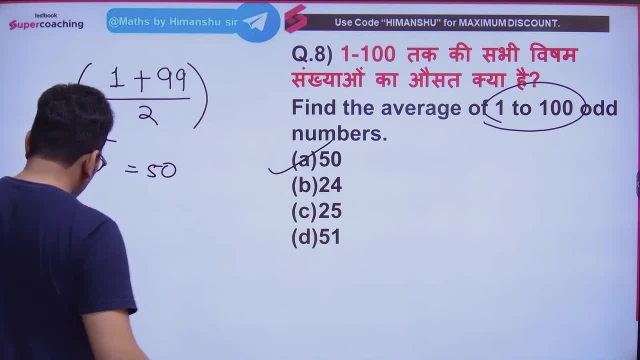 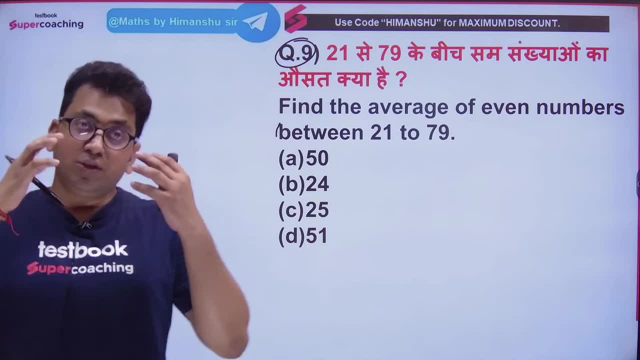 Come on, Let's come to the question number eight, son, Sorry, let's come to 9.. Next question, Question 9.. The child is saying that, sir, you teach math very well. Son, I teach math very well. 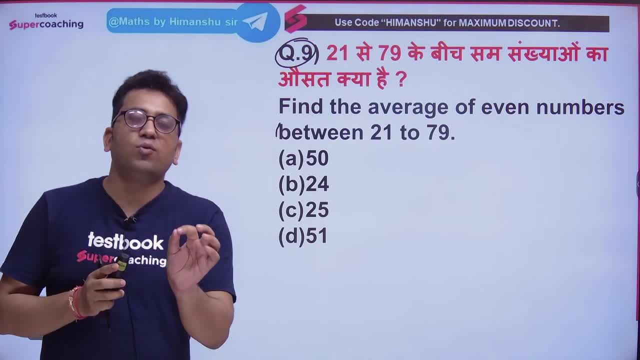 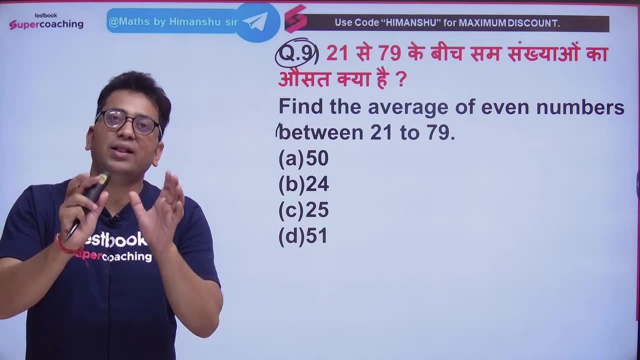 What I mean to say is that whatever subject I will teach you, I will teach it from the heart, I will teach it with determination, And if I teach it with heart and determination, then it will definitely reach your heart and mind. Okay, 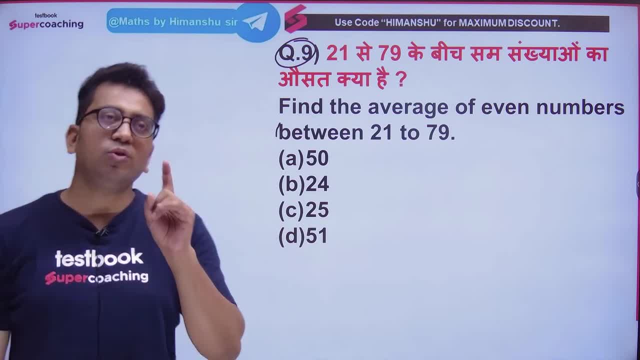 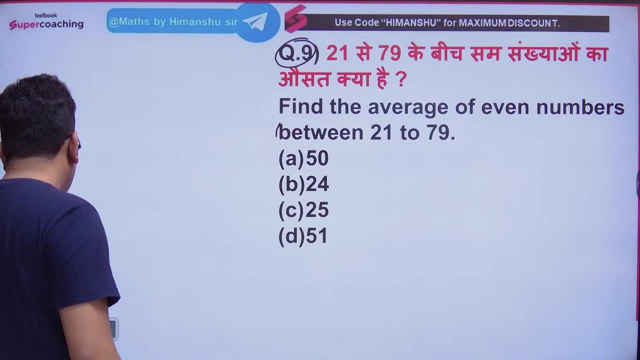 Whatever the subject may be, Any subject and any teacher, if he teaches from the heart, then your heart and mind will reach. Next question is in front of you: From 21 to 21,. it is starting and going to 79.. 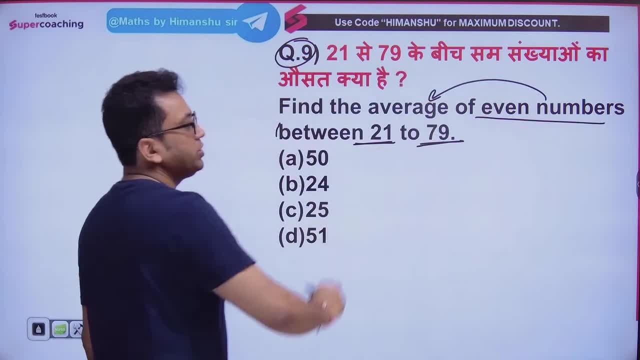 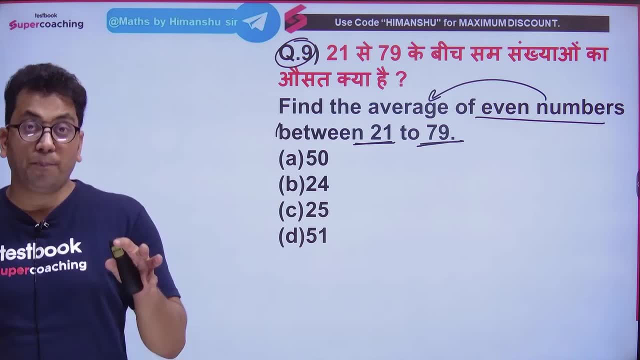 And here you have to find the average of even numbers, Find the average of all the numbers. Tell me what will be the answer Now, it has not been picked up from one, it has been picked up from the middle. Tell me, If you know the concept, then there is no question for you. 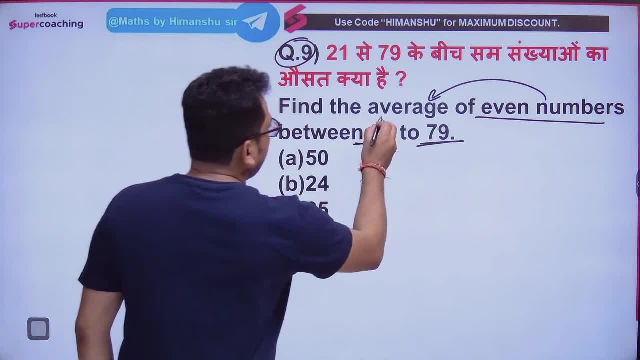 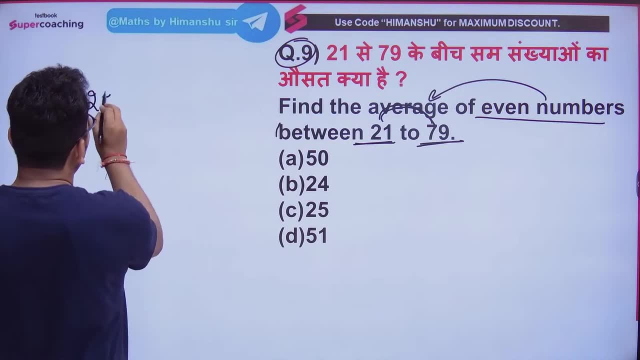 Come on, See my dear, It is starting from 21.. Now tell me, is your even number 21?? After 21, your even number is 22.. So I got the smallest 22.. In this range, in this range, I got the smallest 22.. 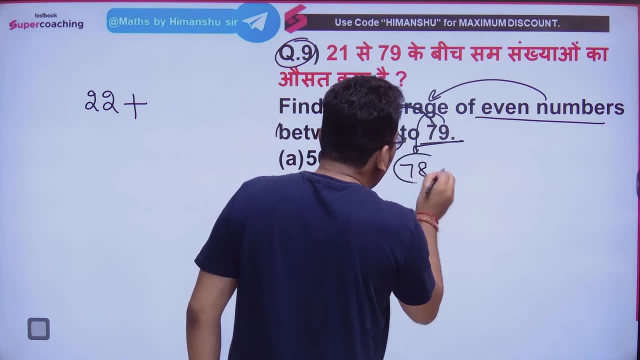 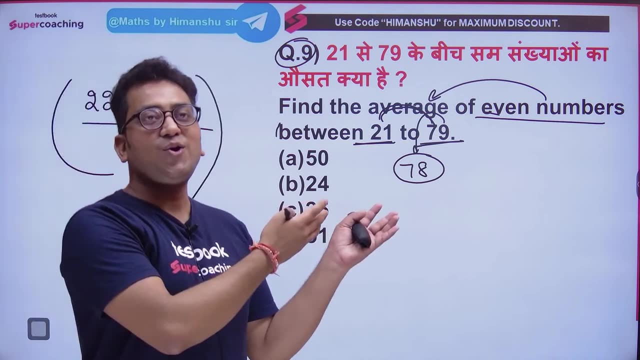 What will be the last Before 79.. I will get 28 because I have to see even That means I got 78. We will add both and divide by 2.. 70,, 20,, 90 and 100.. 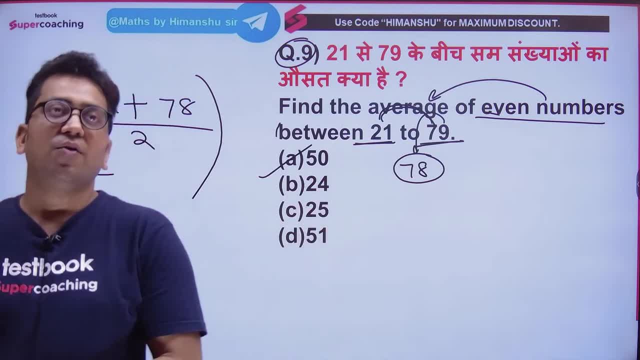 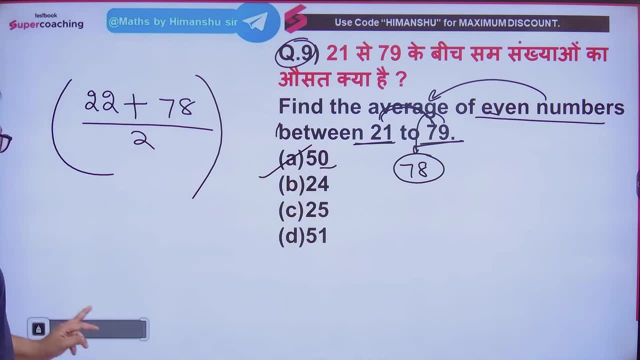 100 divided by 2. That means we will get 50 answers. 50 is the right answer. All the children are giving A answers. They are answering A. They are answering 50. Their answer is absolutely correct. Come on, let's move on. 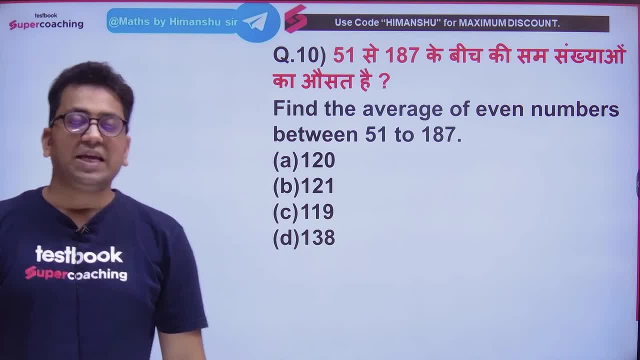 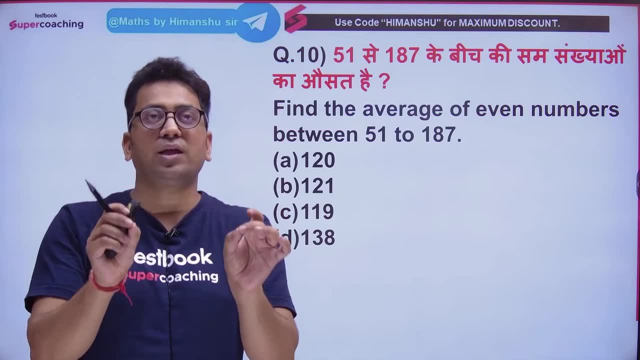 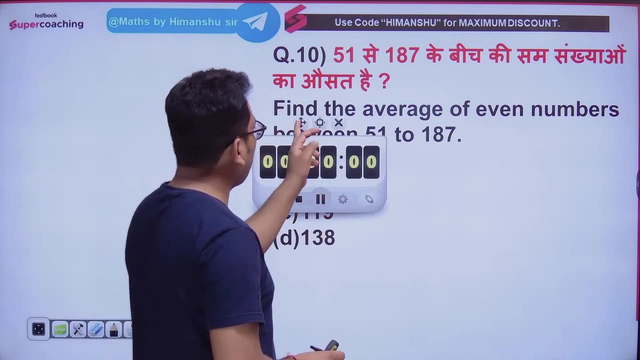 Why the next question? 10th question, Between 51 to 187.. Whatever the sum numbers are, You have to remember the number of them. Come on, let's see how many children are answering. The timer is set to 20 seconds. 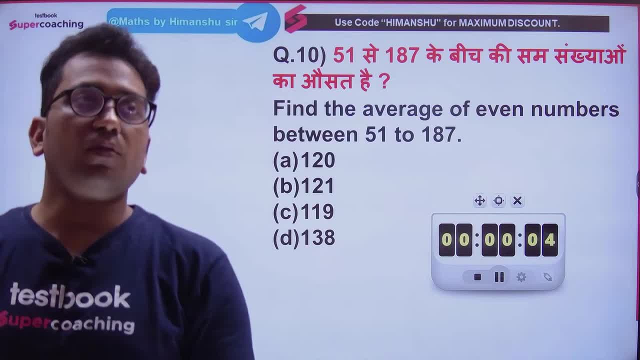 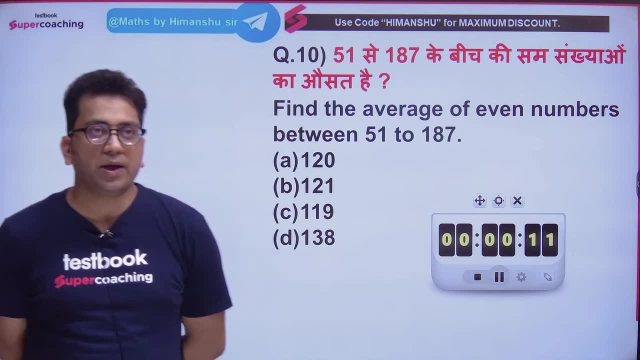 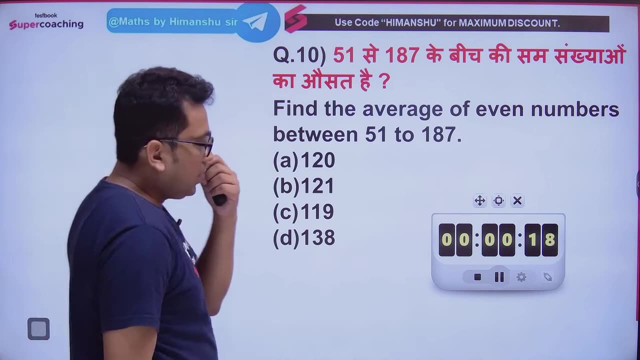 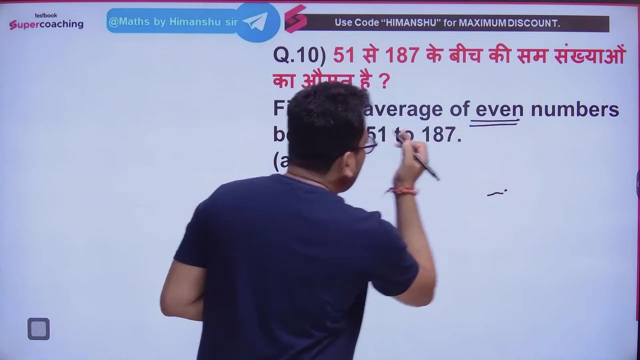 Answer all of them. Very good, very good. See a little. Pay attention here, my dear. OK, Come on, They are telling you the sum numbers. Sir, is 51 the sum number? No, sir. It is not divided by 2.. 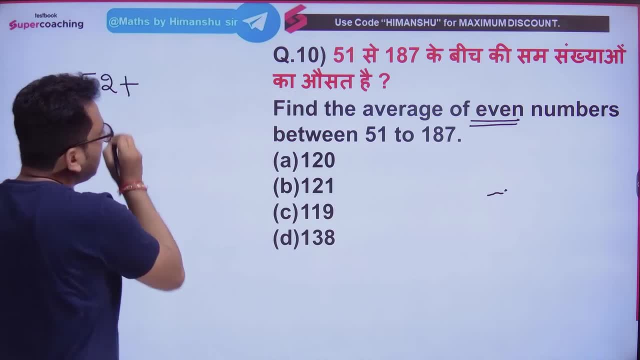 The next one is 52.. That means the smallest one is 52.. What will be the last one? 187 is not 187. It is the first one. That means 186.. We will add both and divide by 2.. 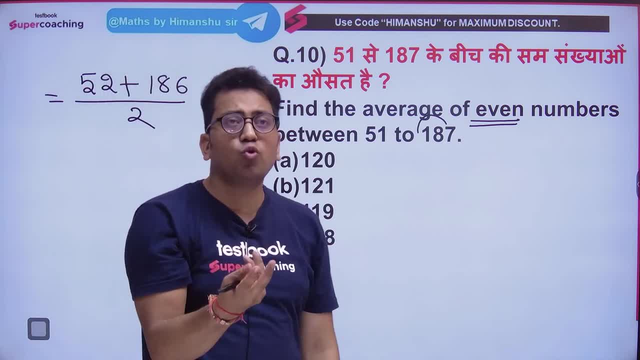 Why are we doing this? Because these are the sum numbers. There is an interval of 2 and 2.. There is an interval. We will add both. 2 and 6 is 8.. 8 and 5 is 13.. 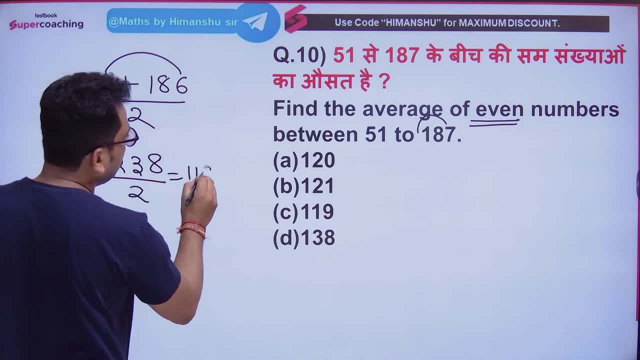 The result is 1. 238.. We will divide 238 by half, It is 119.. We got the random answer: 200 divided by half is 100.. 38 divided by half is 19.. That means 119.. 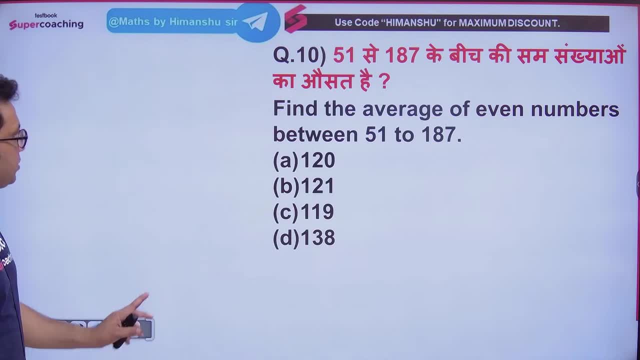 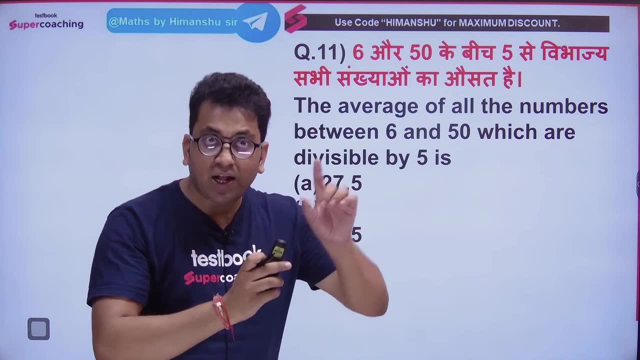 Very good, Very good. Let's move on to the next question, Question number 11.. Understand carefully, I am not making you do things. See, I am making changes in the question Slowly. What will happen with this? Your concept will become very strong. 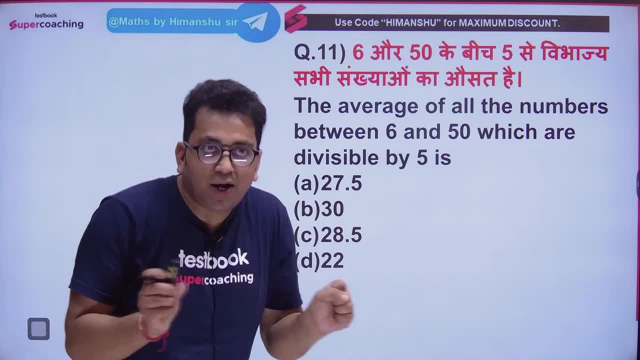 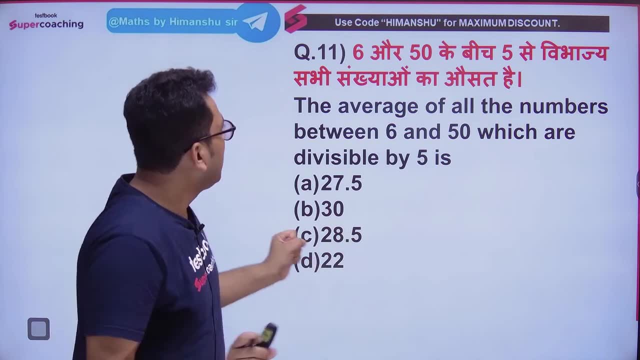 It will become very strong, No matter how much he is shaking in that question. He wants to shake you. See how he shakes. You do not be shaken. You will not get excited. Now see what he is saying here. There is no difference between 6 and 50.. 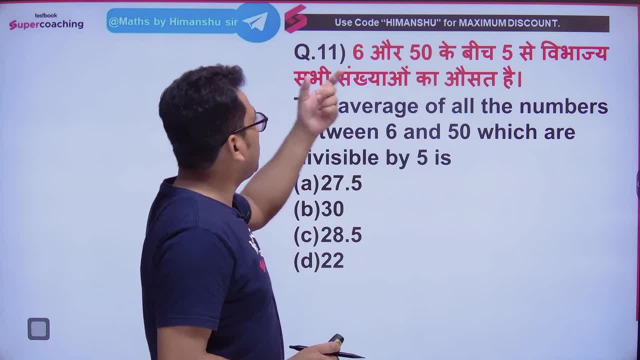 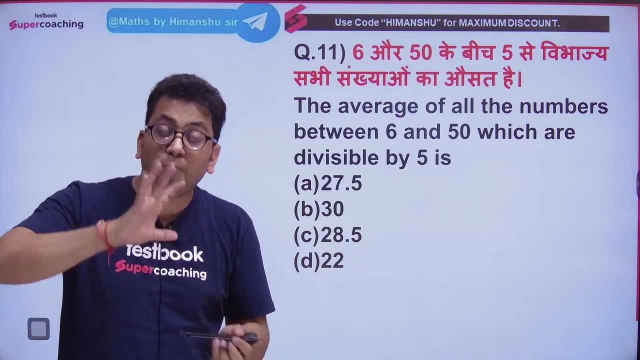 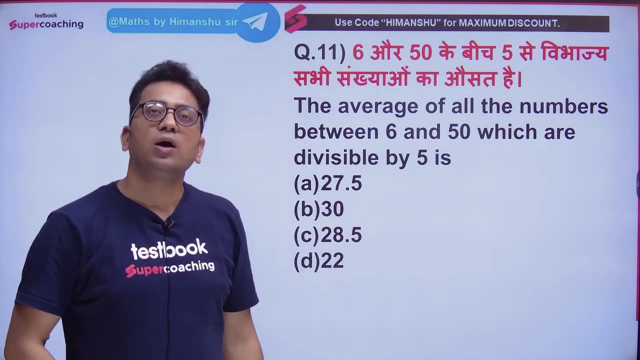 All the numbers which are divided by 5.. Now such a matrix where such numbers are divided by 5, then say how much is the difference between them? Will it be equal? It will be absolutely equal, Sir. read the five tower and see. 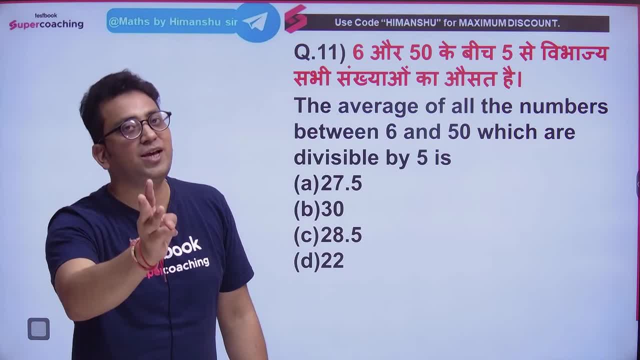 5 x 1 is equal to 5,. 5 x 2 is equal to 10,. 5 x 3 is equal to 15,. 5 x 4 is equal to 20,. 5 x 5 is equal to 25,. 5 x 6 is equal to 30. 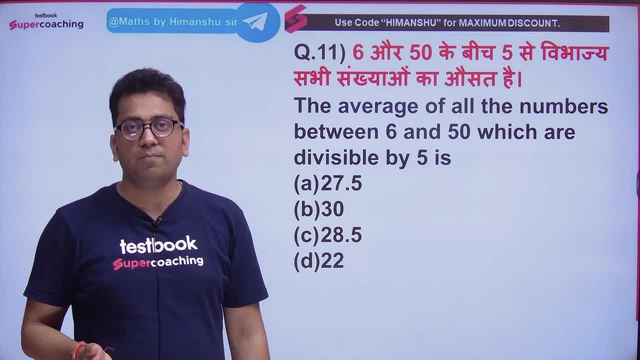 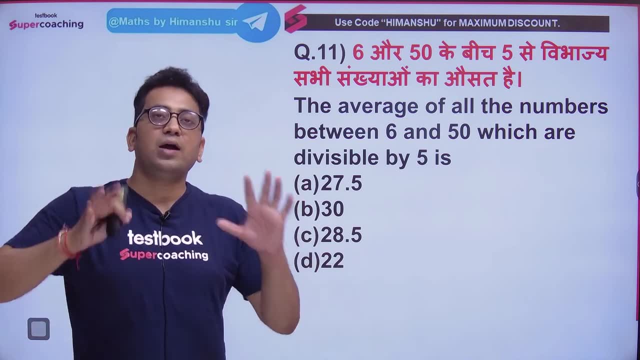 There is a 5 x 5 difference in all the numbers. If 5 is divided by 5, then there is a 5 x 5 difference. That is, there is a difference. To apply this concept, we need a difference between the columns. 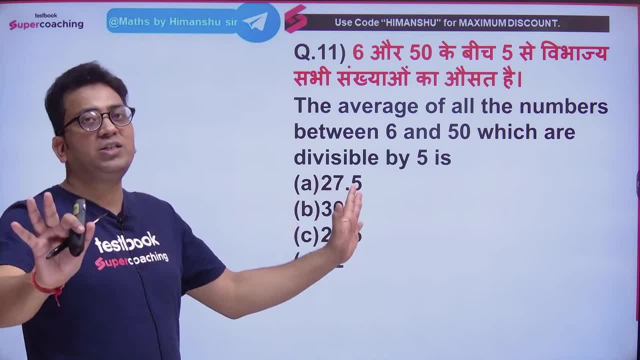 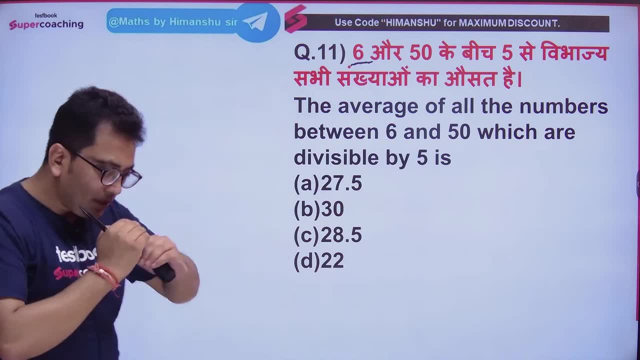 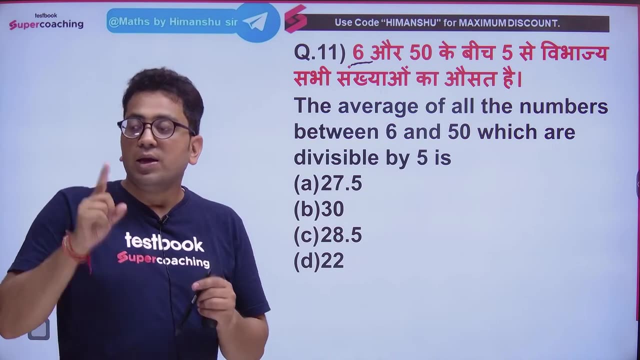 We are getting that here, So we are going to use the same formula again: The smallest and the largest number. Now tell me, After 6,, which number will be the first to be divided by 5?? Sir, 5 x 5 is equal to 5,. 5 x 2 is equal to 10.. 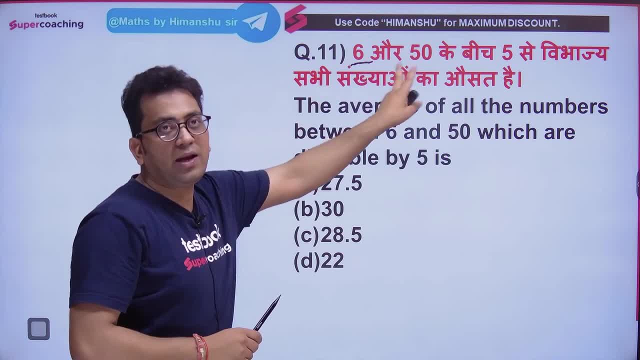 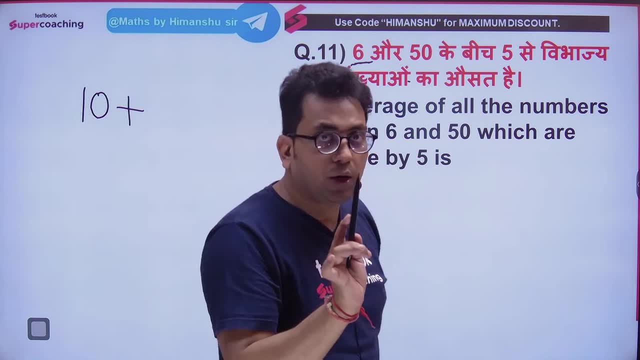 See 5 will not come. It is not coming. in this range, 5 x 2 is equal to 10.. The first number will be 10.. Are you able to understand? I am touching every aspect. What will be the last? 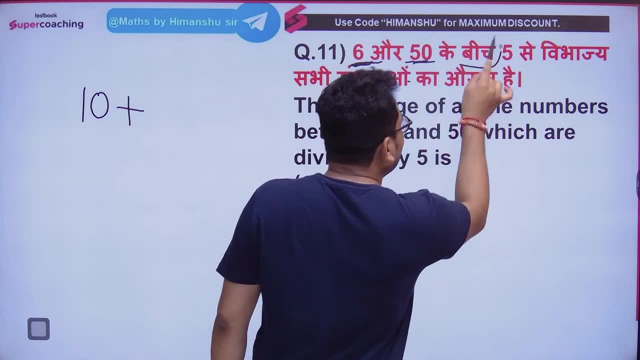 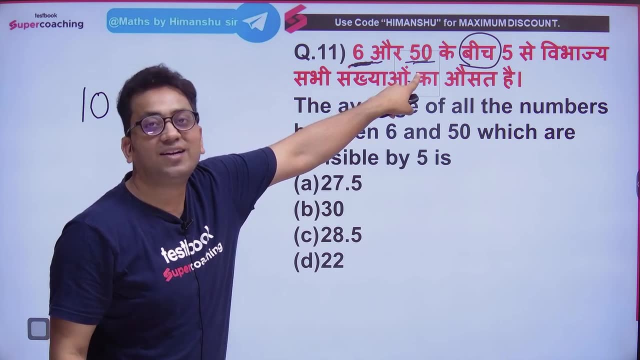 Sir, he is saying in between 6 and 50. In between, Yes, Don't take 50. The box will be rolled. No, Don't take 50, son. In between 50, 45. Brother, it will be less than 5.. 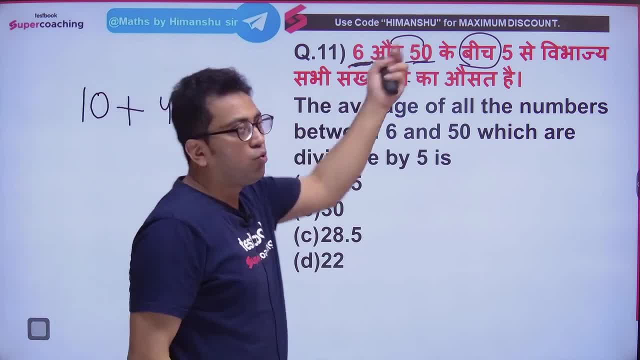 That is, it will be 45. We will not think Because it is 50, then it will be less than 5, then it will be 45. Don't take 50. Many children take 50. It gets messed up. 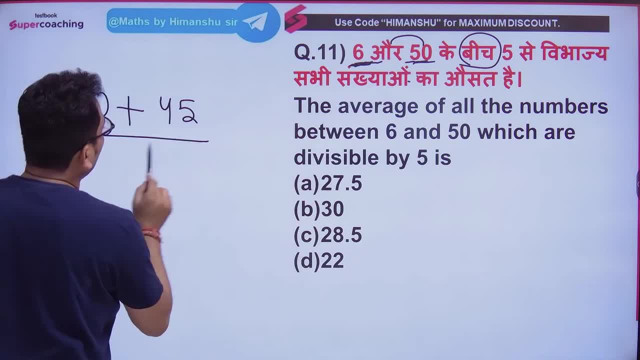 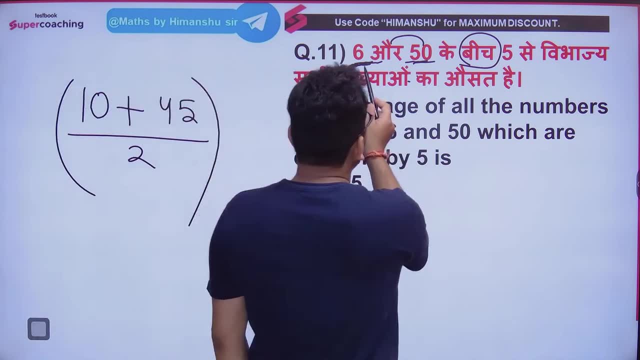 Don't take 50.. Isn't it? Take 45.. Now we will add it and divide it by 2.. The concept will remain the same. We will add the smallest and the largest and divide it by 2.. See, if he had said 6 to 50,, then I would have taken 50. 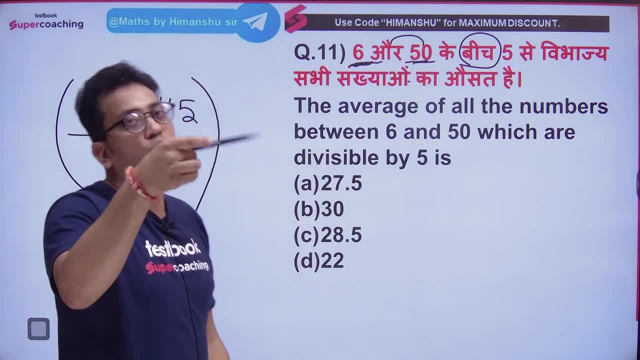 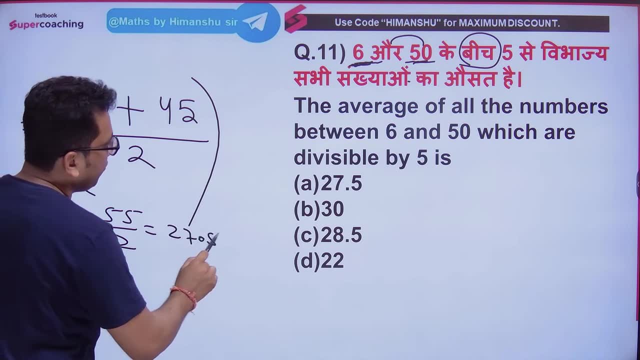 But he said between 6 and 50, then I will take 45. Let's add son 55. If we do half of 55, then how much will it be? It should be 27.5, which you can see in option A. 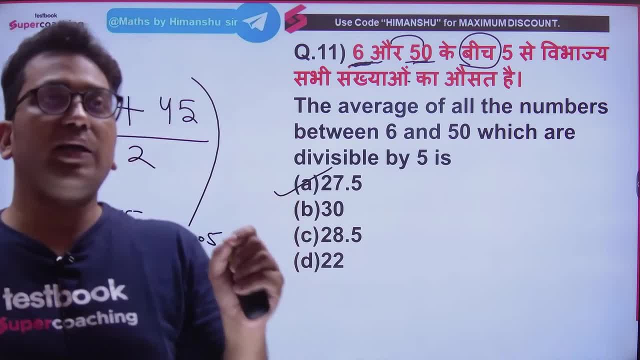 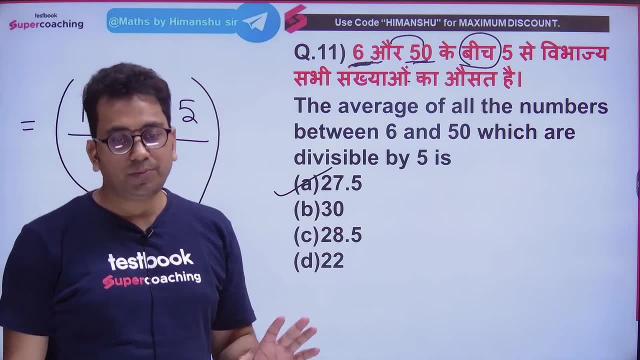 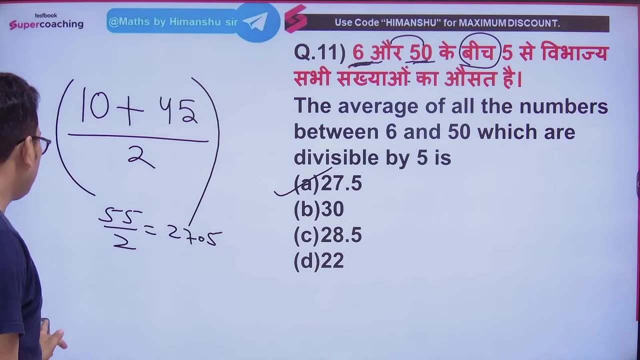 In my opinion, every child must have understood. 27.5 children are answering here. Okay, brother, Are you able to understand? Yes, Is it clear to all of you? There should be no problem. Let's move ahead. The next question is coming in front of you. 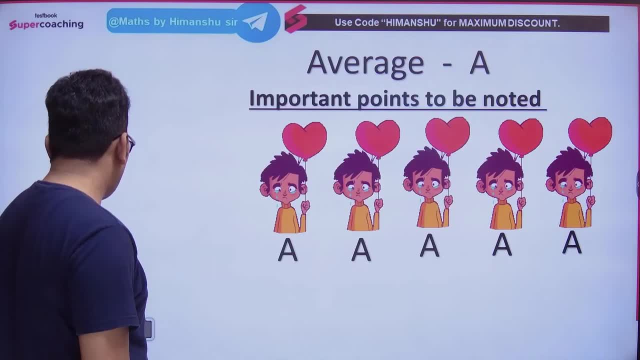 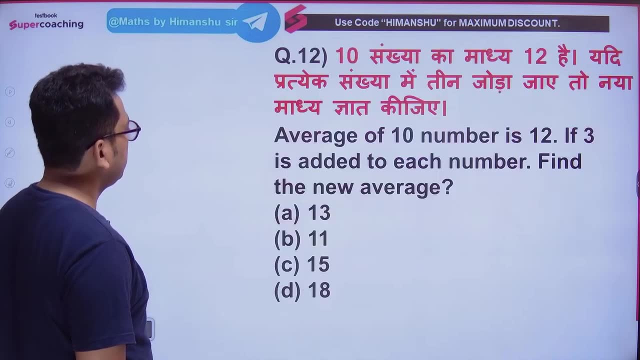 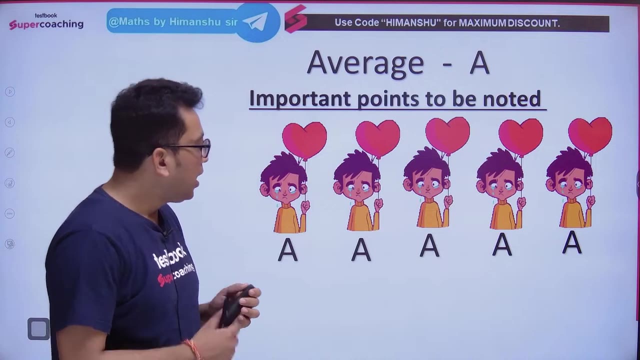 Not the next question, but the next concept. Okay, Now, look, we will explain this concept to you. Okay, Listen to me carefully. Okay, You have here 1,, 2,, 3,, 4, 5.. You can see 5 people. 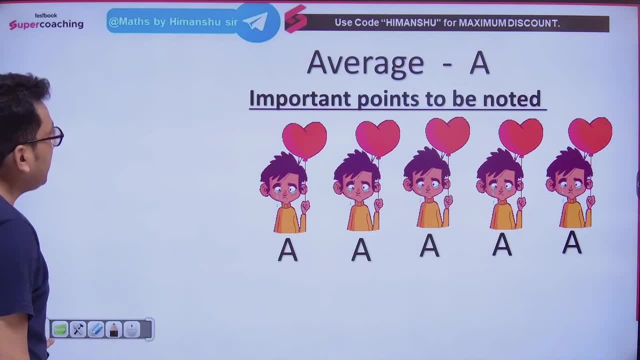 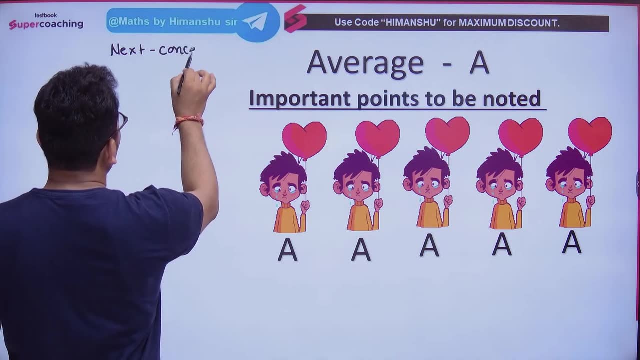 You must be seeing tears in their eyes. I am going to explain the next concept to you. This is the next concept. This is the next example. son, Just understand the concept Based on this, how questions are asked in your exam. 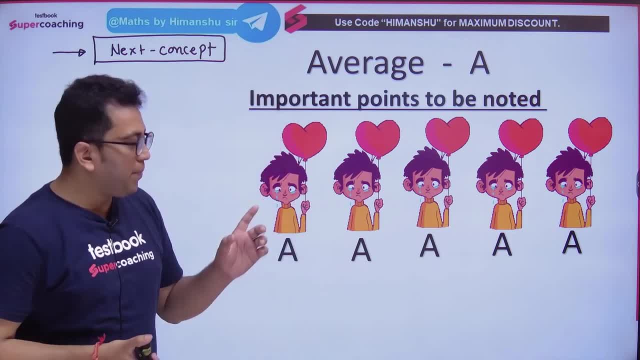 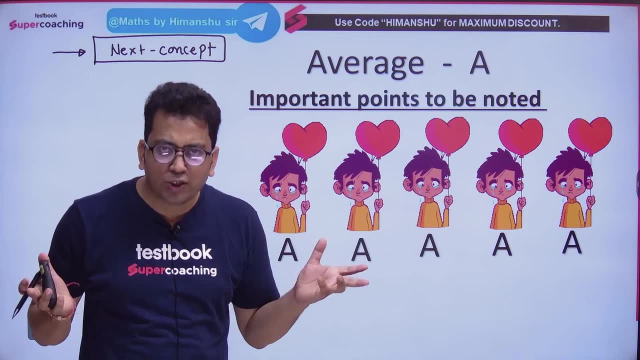 Okay, Listen to me carefully. You must be seeing 5 people here: 1,, 2,, 3,, 4, 5.. These 5 are combined. How Combined? Why is it combined? These 5 are combined because they have a group. 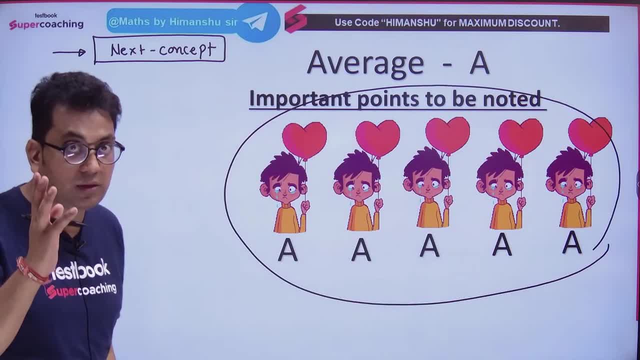 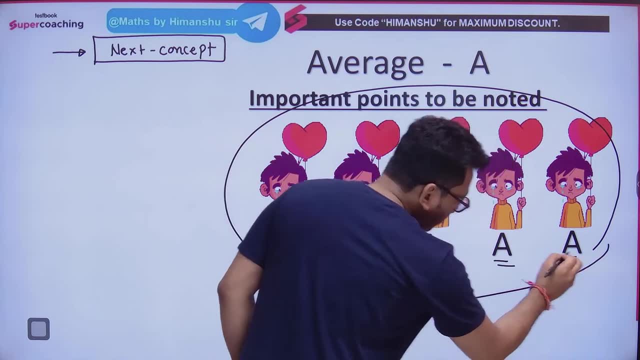 What is their group? They have a group. Listen to me carefully. They have a group And their average is A. All of them have A, A, A, A, A. Listen to me carefully, These are 5 people. 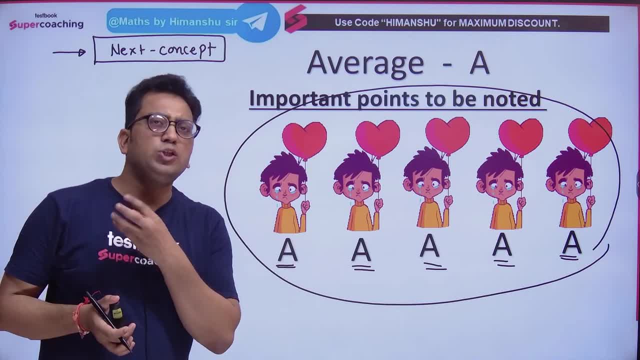 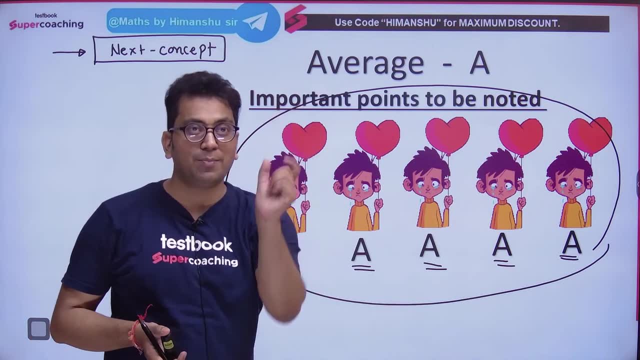 And these 5 are combined. You can assume that they are combined. Why are they combined? Because they are in a group And we have given them A, A, A. Now you must be seeing their hearts in their hands And you must be seeing tears in their eyes. 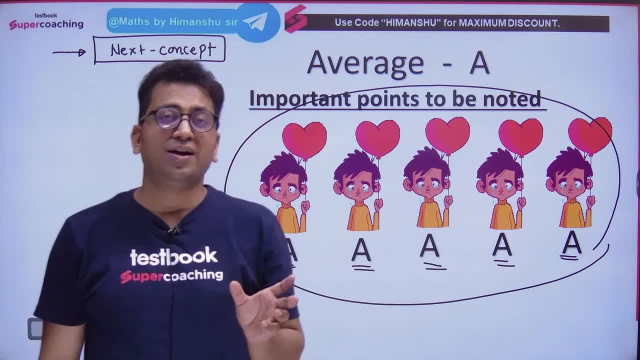 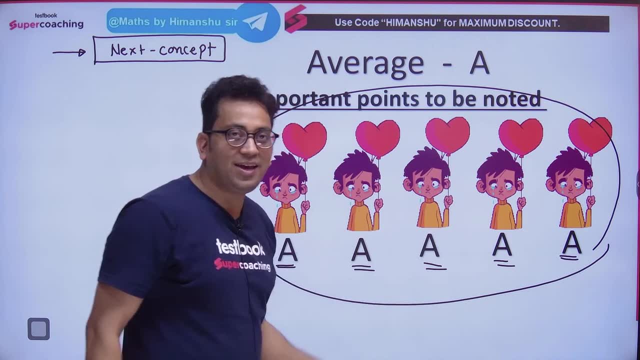 So you must be seeing their hearts and tears. You must have understood that someone has broken their hearts. They have turned towards destruction. This is the situation. So see what happened. You must have seen the movie. What happens in the relationship? It is the same with one. 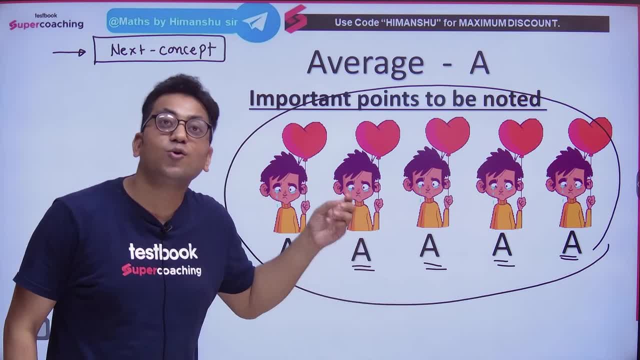 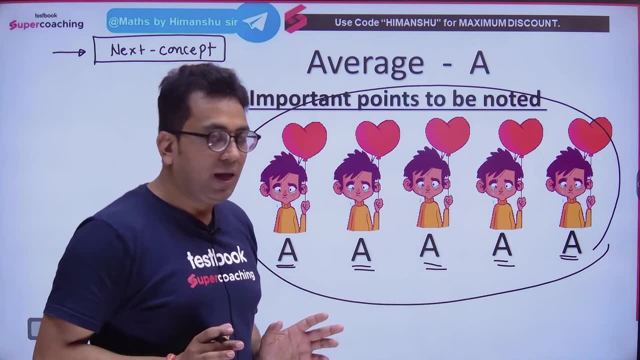 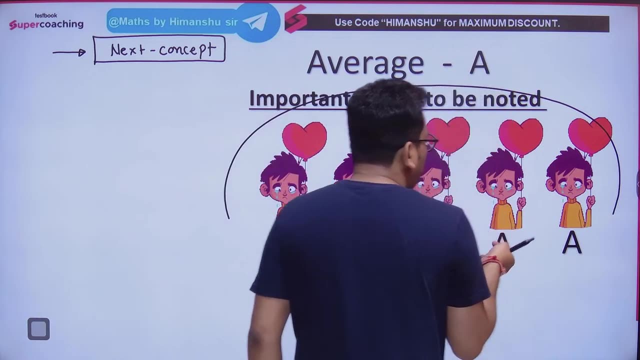 It is the same with the other. It is the same with them too. Brother, one's heart broke, Everyone's heart broke, Everyone's heart broke, Everyone's heart broke. Okay, What I mean to say is that they say that if you tease one of us, then the rest will tease themselves. 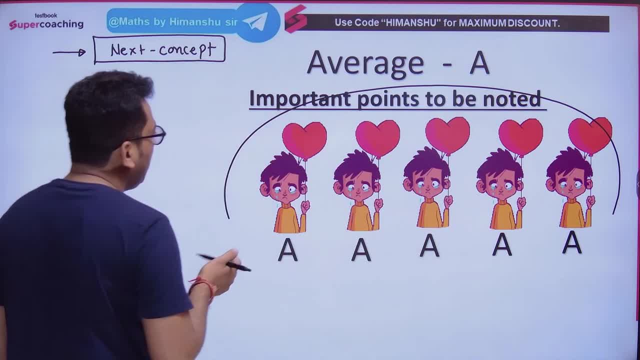 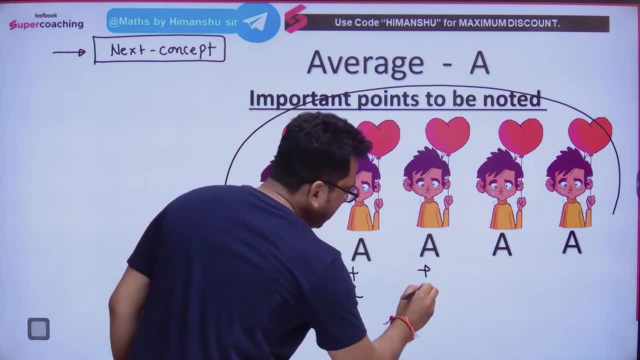 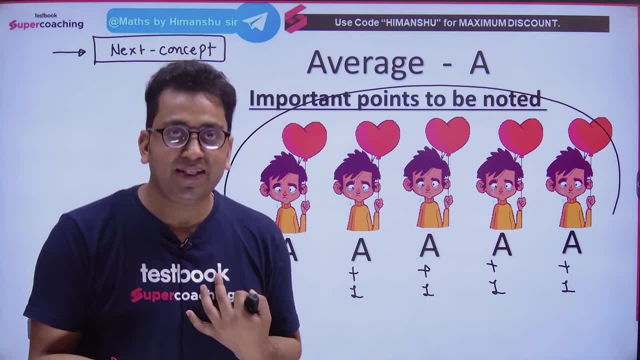 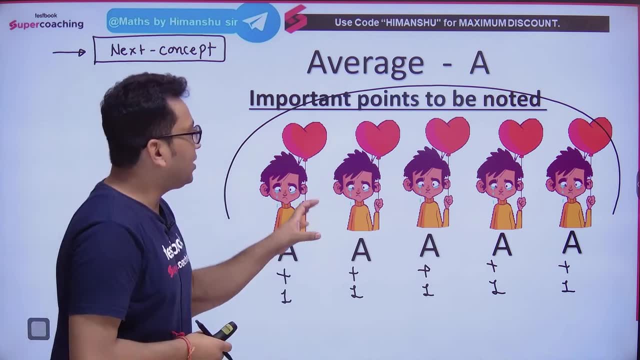 We will beat, beat, beat. We will beat, beat beat. We are math lecturers, We are math students. We are math students, we are Math. So we will divide the value of the standing and the lost. So, brother, if his heart broke, 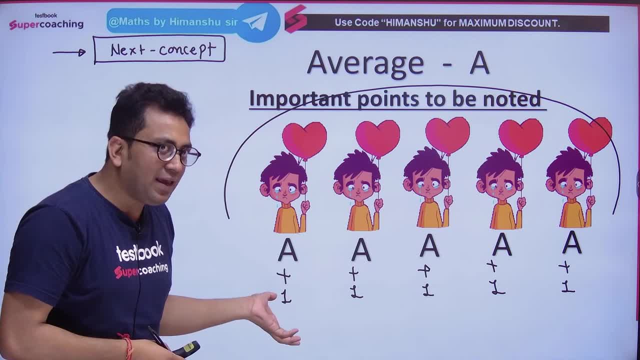 So the one who is joining will give it back. So we gave the one who is joining. So they all also say that we also have to join the heart. So we gave one to each of us. Assume that we all take down one of the parts, then they will say, brother, take it from us too. 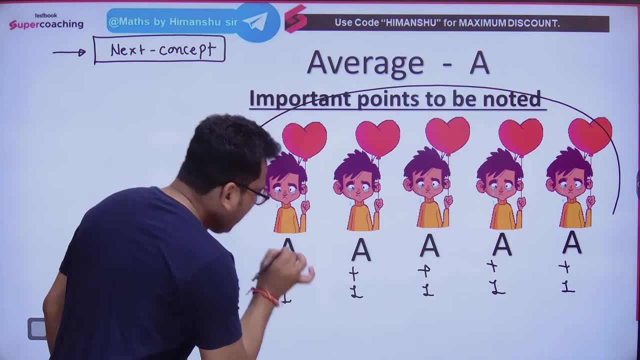 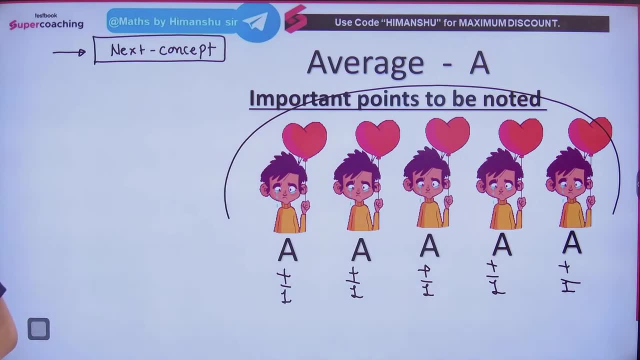 take it from us. take it from us, separate it from us too, isn't it, Sir? that's what we will do: Take it away. It means that if the heart of one is broken, then the heart of the rest will also be broken. 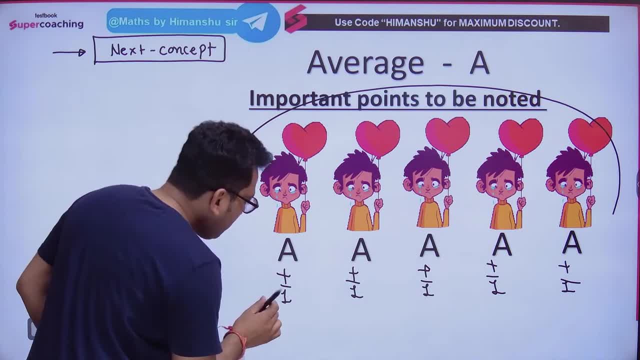 Do you understand One by one? it will be minus. If I am multiplying by one here. if I am multiplying by any number, then this will also be multiplied by this. this will also be multiplied by this, and this will also be multiplied by this. 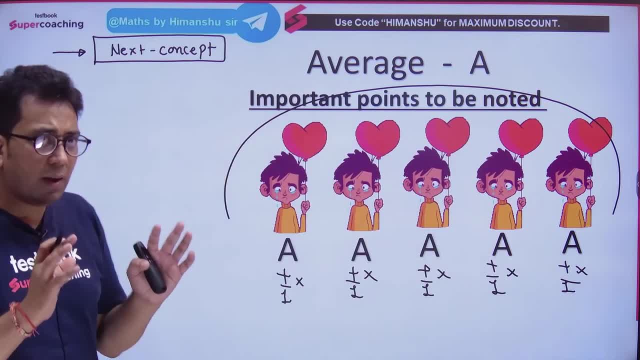 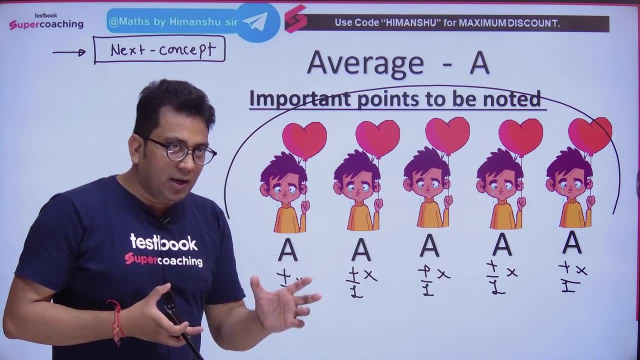 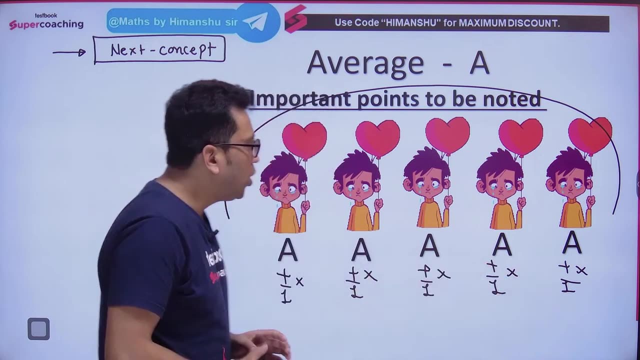 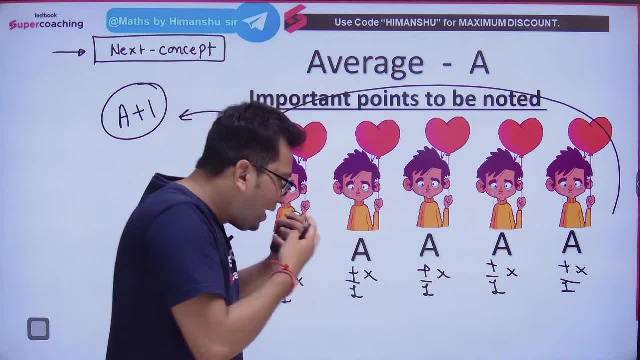 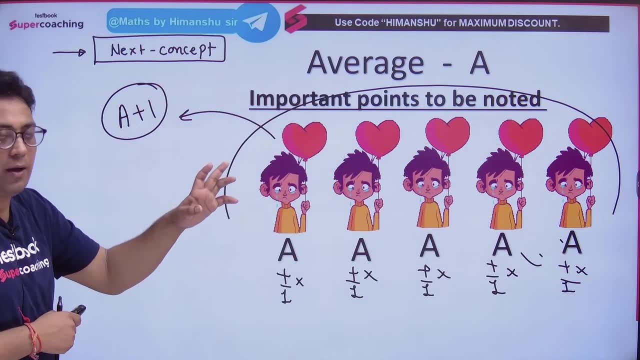 Why? Because the meaning of average is per head. That is what is happening with each other. If everything is happening the same, then the whole group will also be added to it. If everyone has one, If everything is happening minus minus one, then the average of the whole group will also be minus one. 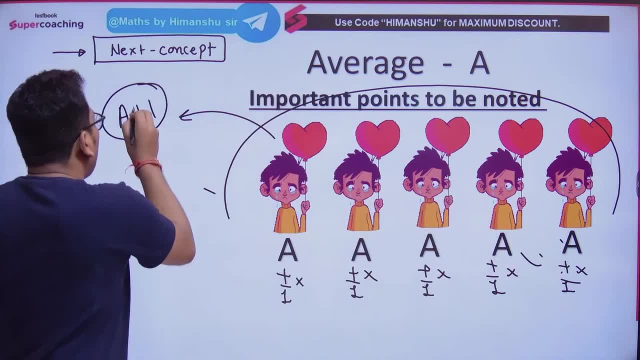 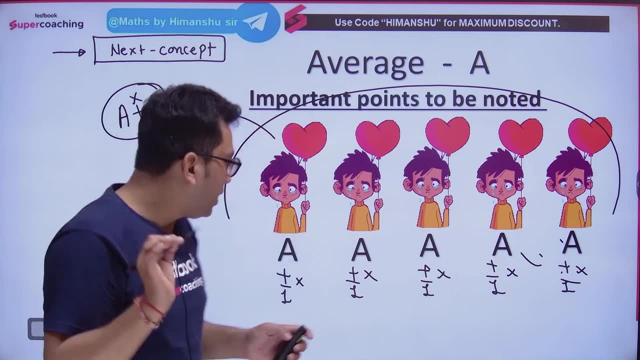 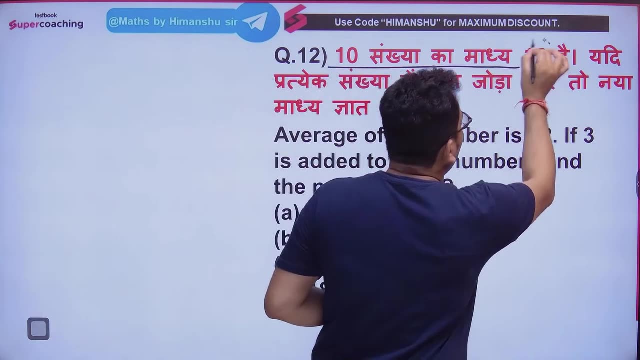 If everything is multiplying with each other, then the average of the whole group will also be multiplied, And in this way the concept of division will also follow From here. the question that comes to you directly from this concept is that if the number of 10 is 12, understand. 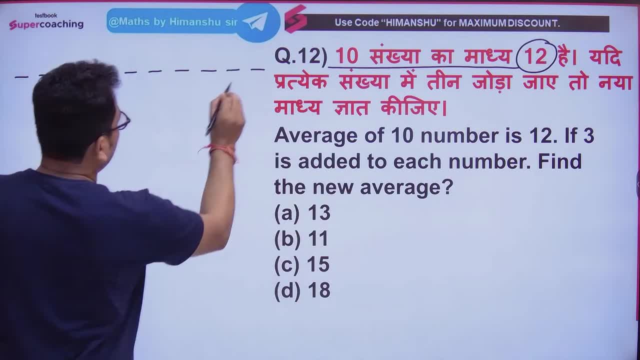 1,, 2,, 3,, 4,, 5,, 6,, 7,, 8,, 9, 10.. Imagine these 10 numbers. How much is their average? 12. They are all the same combination. 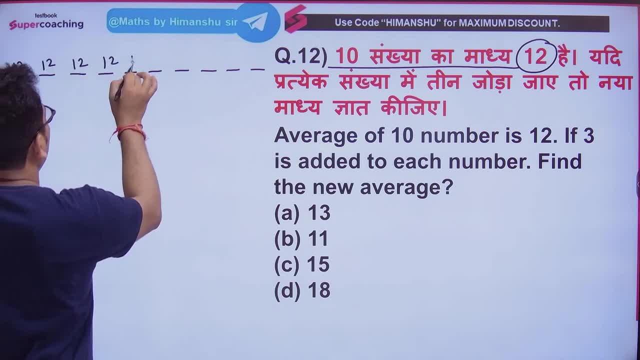 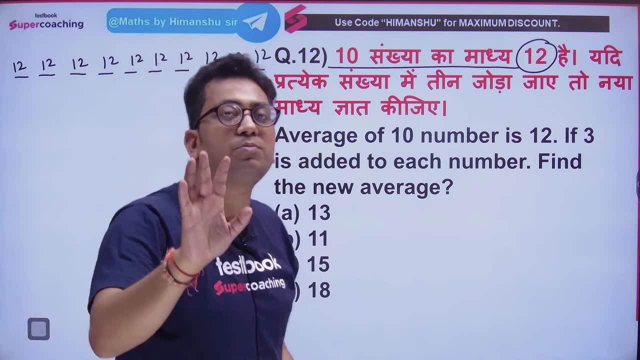 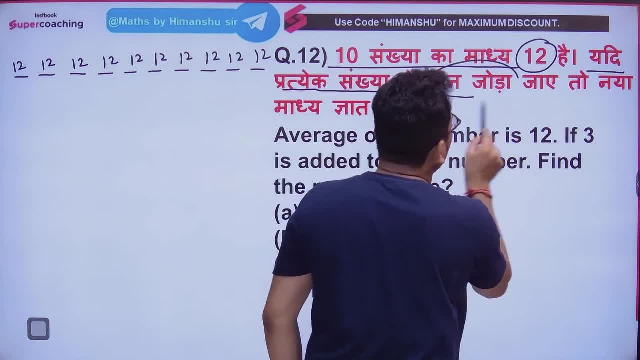 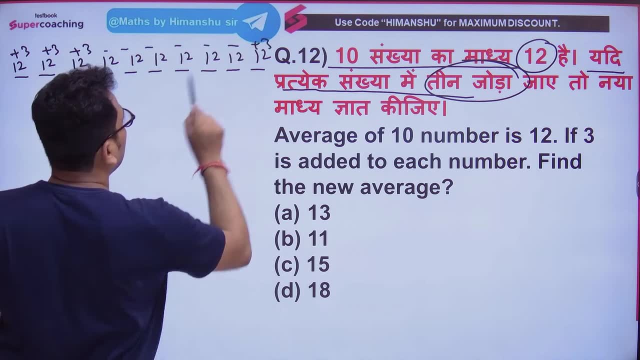 Now he is saying that if 3 are added to each number, 3 are added to each number. 3 are added here. 3 are added here. 3 are added here. 3 are added to everyone. So he is saying: tell me what will be the new average. 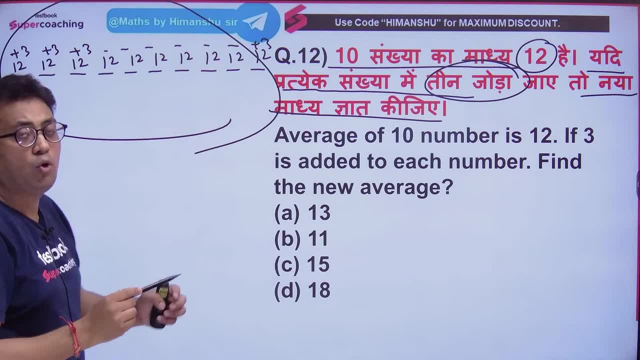 That is what will be the average of this whole group. Tell me, If you add 3 to each, then what is the average that everyone has? That is, 12 and 3, how much will the average be? It will be 15.. 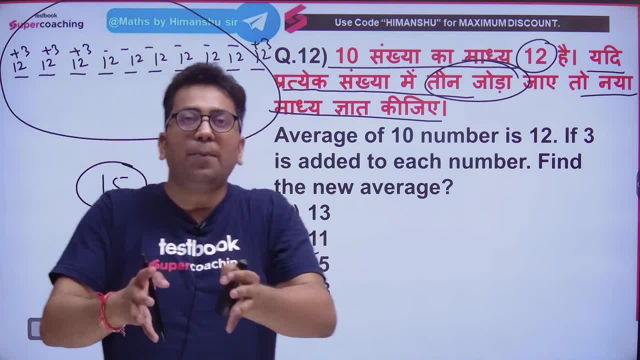 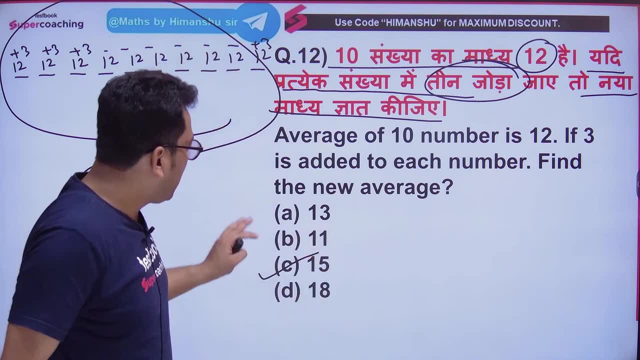 So here the concept says that what you are doing per head, that is, with each one, that will be your average. It is a simple funda. And here you are directly asked a question. See the next question in front of you. 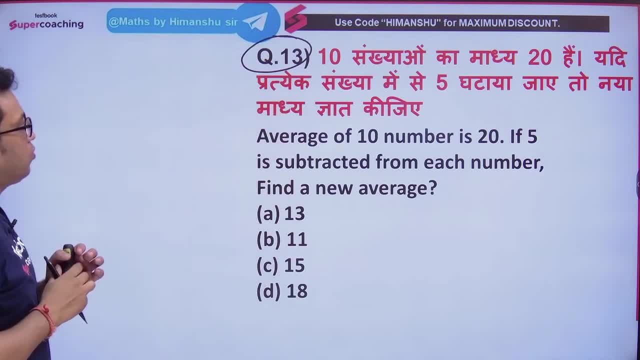 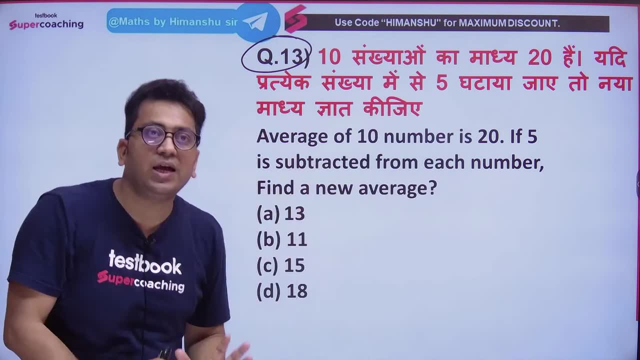 Here is the 13th question. Let's see how many children are able to answer the questions. The matter of 10 numbers has given you 20.. If 5 out of every number is reduced, if 5 out of every number is reduced, then what will be the new average? 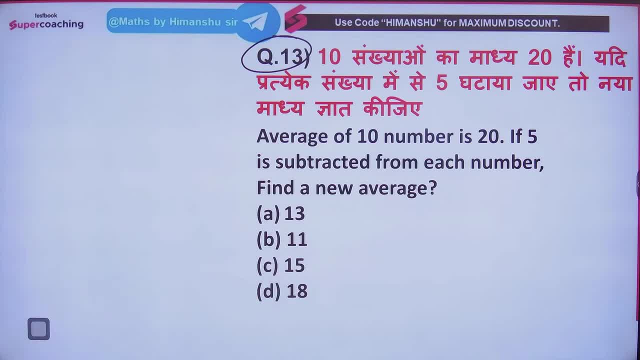 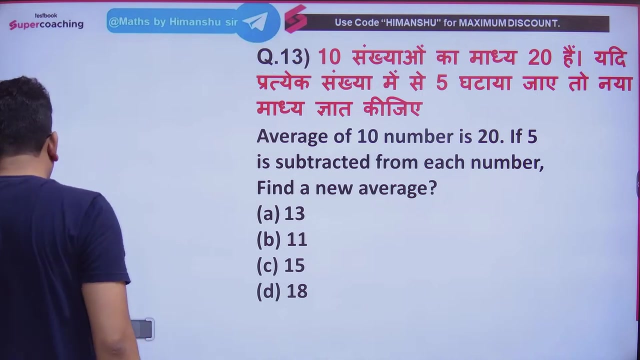 Answer quickly. Tell me what will be the answer. All of you answer with speed. Tell me my son. Hmm, I will tell you what will be the new average. Look carefully: 5 has been reduced. 5 out of every number has been reduced. 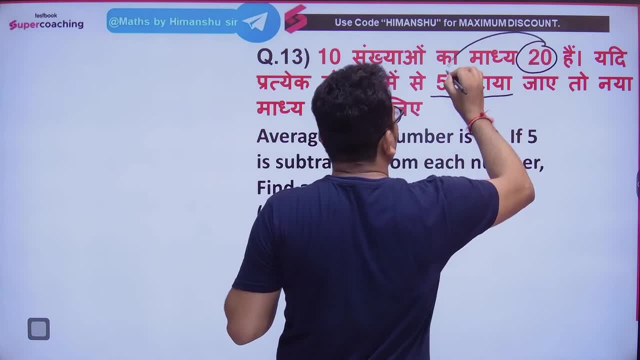 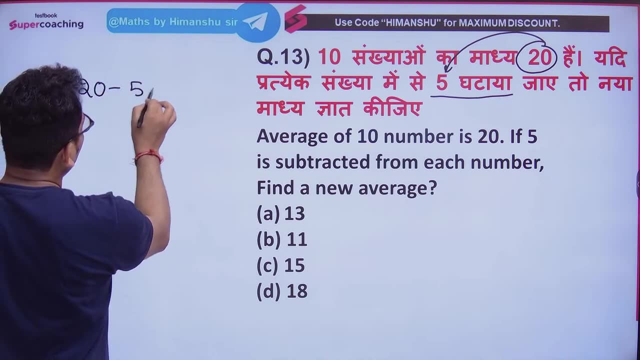 OK, What is the average? 20.. If I reduce 5 out of every number, then 20 will also be reduced out of the average. That is, 20 minus 5.. How much will it be? It will be 15.. 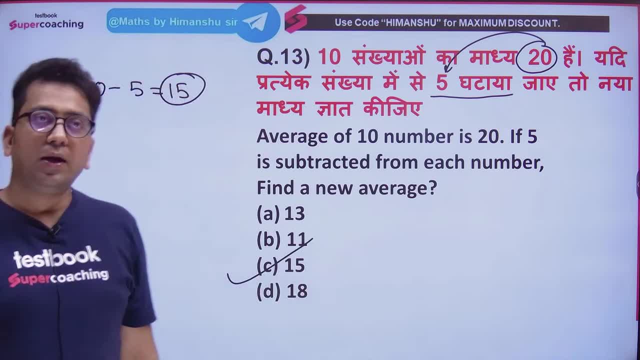 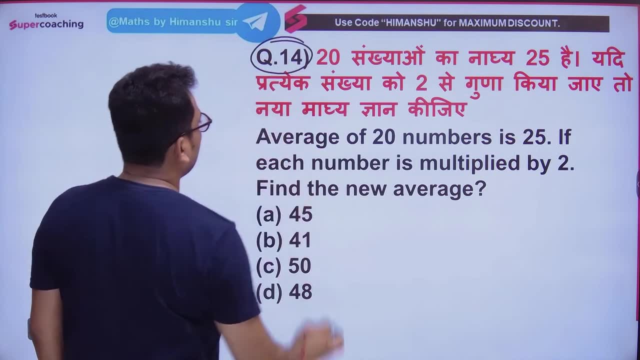 It will be 15.. That is, our answer will be C. OK, So 15 will be the right answer. Our answer will be 15.. Next question, Question number 14, is in front of you. The average of 20 numbers is 25.. 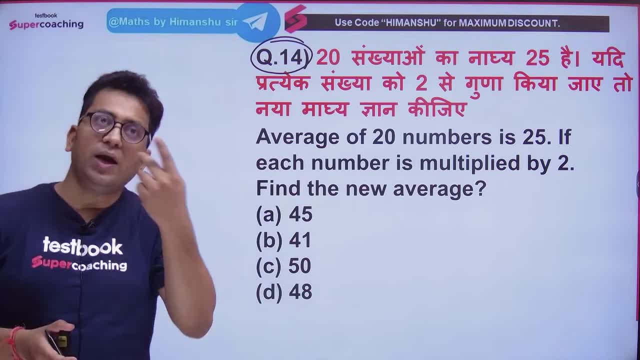 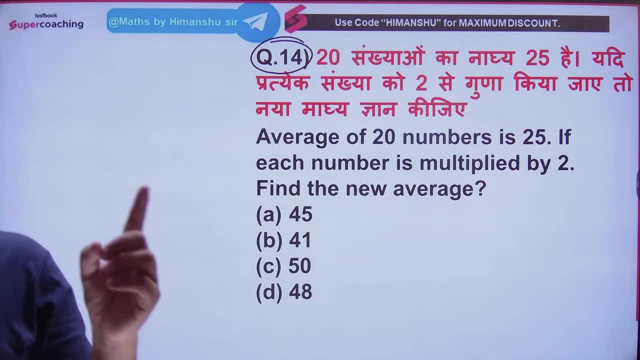 If each number is multiplied by 2,, then what will be the new average? Tell me quickly what will be the answer. Answer with speed. The average of 20 numbers is 25.. If each number is multiplied by 2,, then what will be the new average? 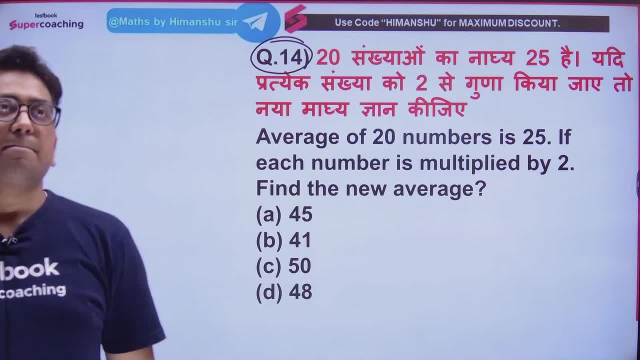 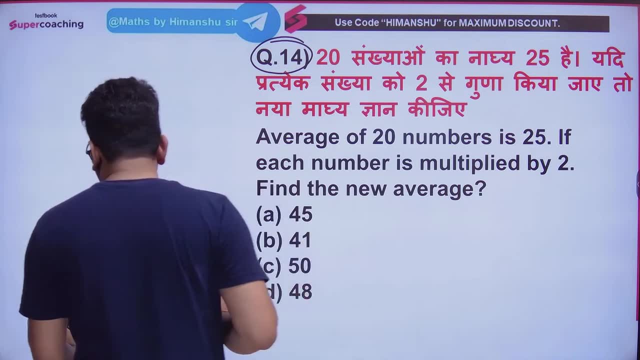 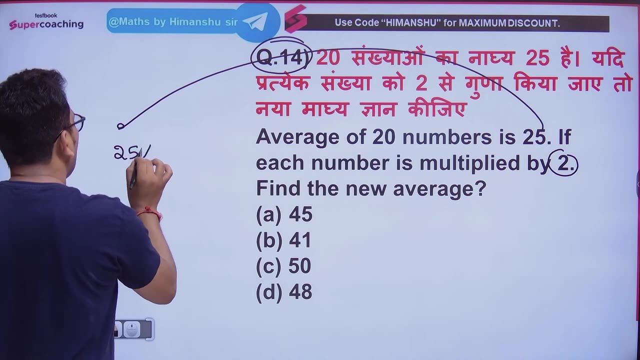 Let's see how many children can answer. Look, you are being told that each is multiplied by 2.. So what will we do, sir? We will raise the average, We will raise 25 and multiply it by 2.. That is 50, will be our answer. 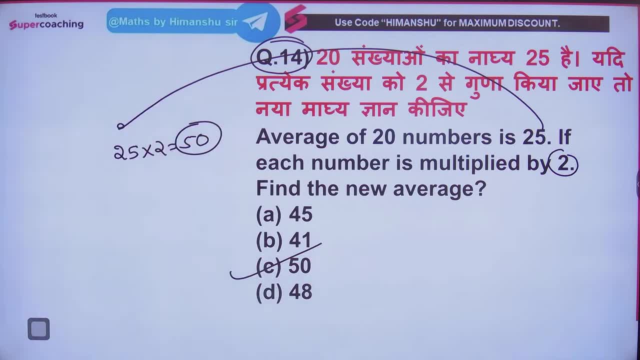 That is, 50 will be the right answer. OK, So 50 will be our answer. 50 will be our answer. The children who are answering C? their answer is absolutely correct. Now see, the question was asked in this pattern. 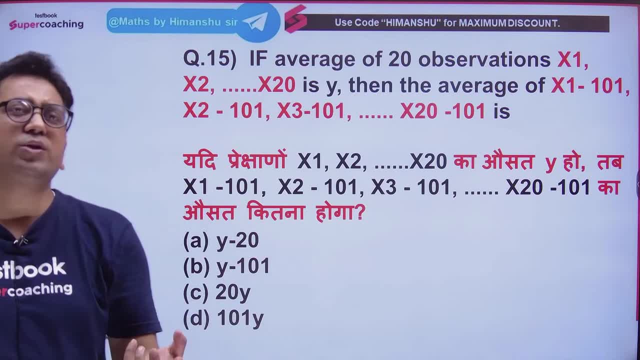 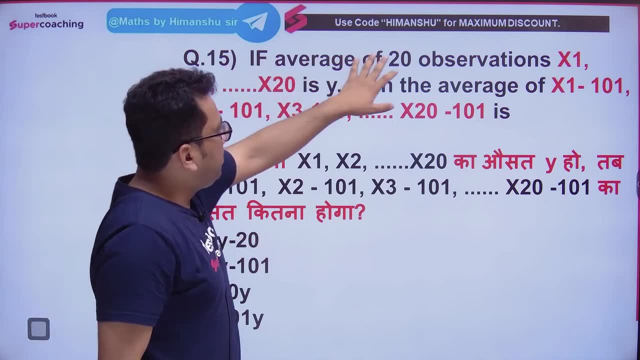 When such a question is asked, the child does not know what has been asked, But you know the concept. You will shine. He is telling you that if there are 20 fractions here, 20 fractions are given in this way. their average is given to you by Y. 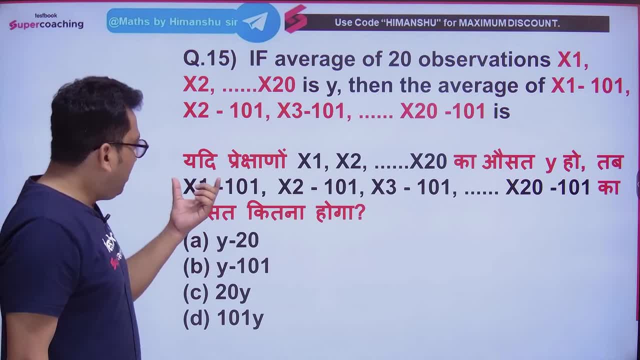 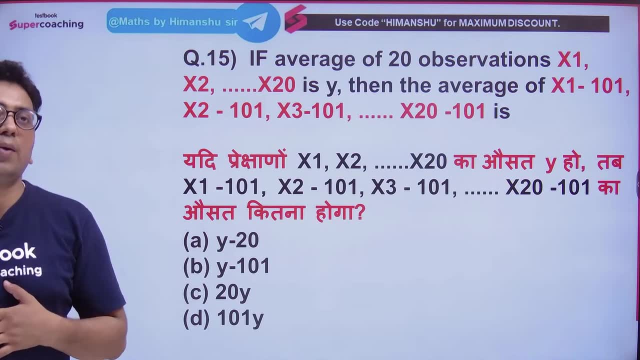 How much is the average Y? You see Now, if each fraction is divided by 2.. If each fraction is reduced by 101, then what will be their new subject? What will be the average? You have to tell this. The options are in front of you. 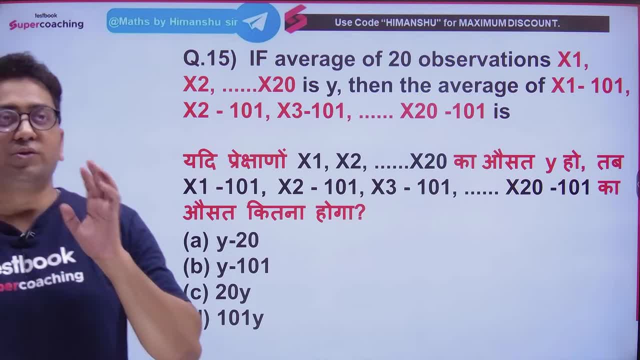 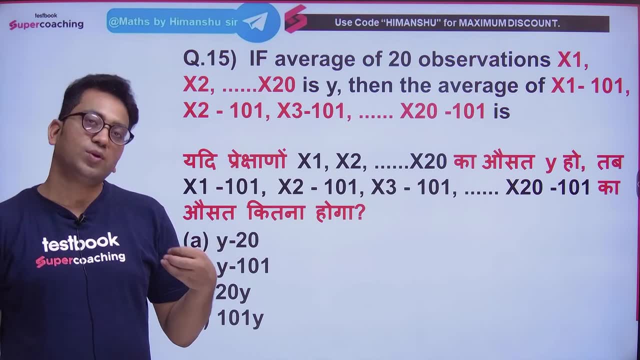 Answer with speed. A child is writing. I love super coaching. Thank you very much. See, this should come from your heart, Isn't it? It comes automatically from the heart. When the child understands, then interest develops. He feels that yes. 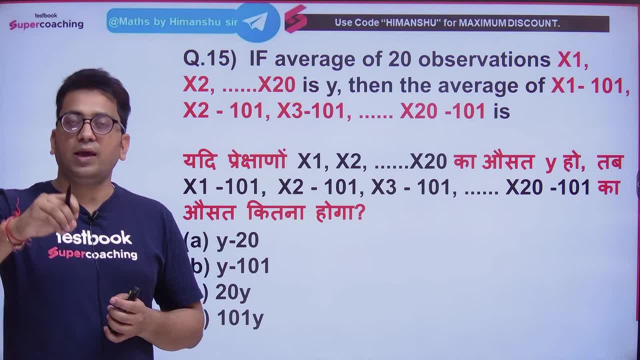 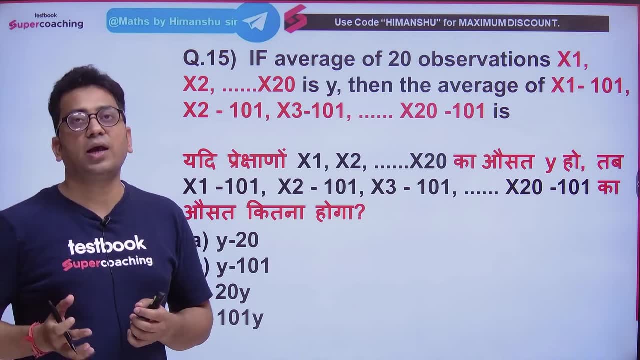 And in reality- let's assume that there is such a platform where you try to provide everything. Everything is being made available, Whether that is your paid batch or we teach you on YouTube. everywhere you are being taught from your heart and from your heart. 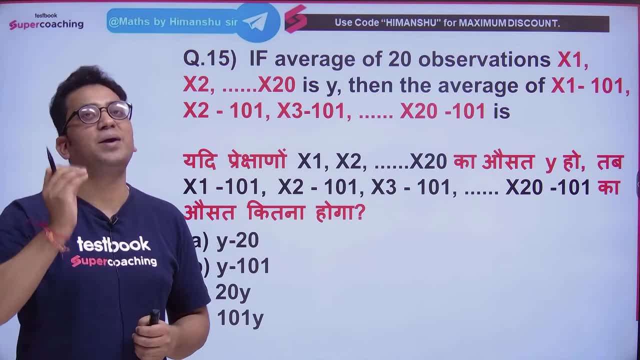 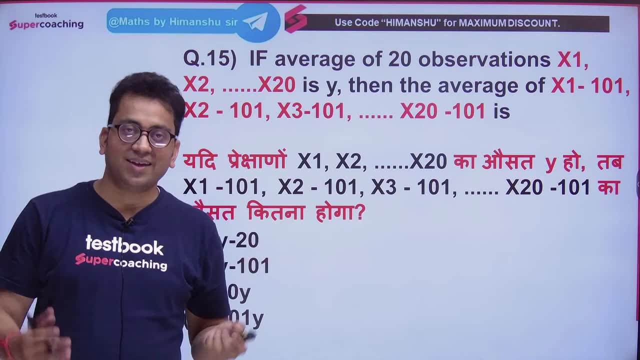 So your selection will be made. and when your selection is made, then how does the child give prayers? And it looks very nice. Who doesn't like all the prayers? Everyone is accepted. The next question is: brother, the children are answering here. 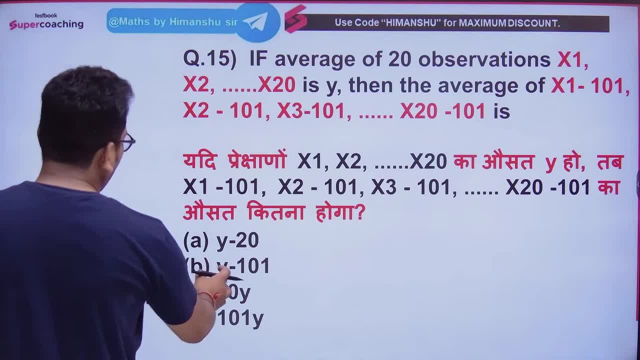 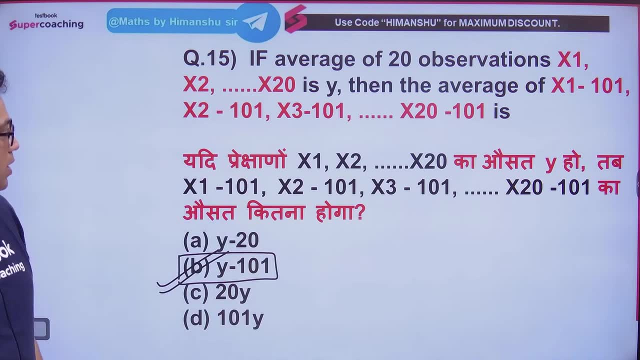 The options are going towards B. Very good, What will be the answer? option number B: Why my mother? Why my mother? Why my mother? y-101, because if 101 is decreasing from all, then 101 will also decrease from your average. 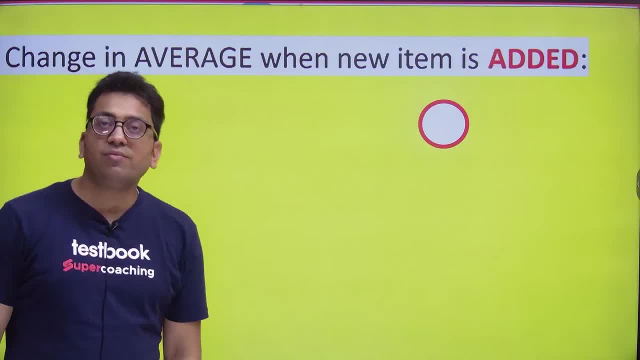 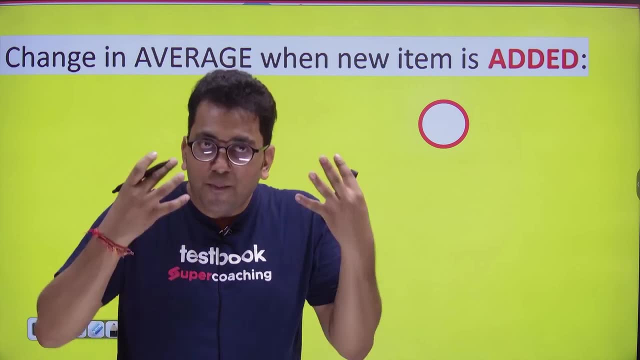 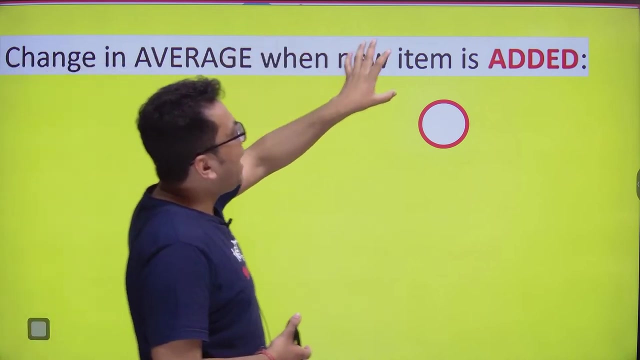 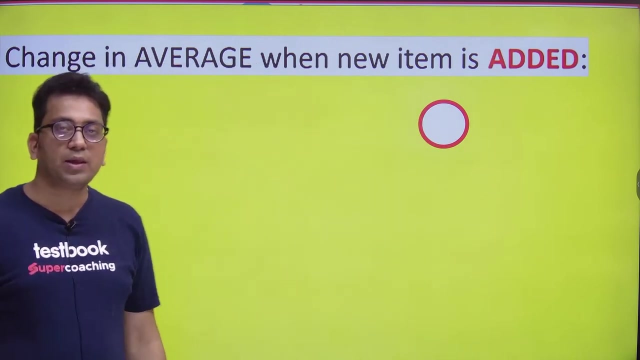 next question. next question is not. next is feeling. I will not even call it concept, I will call it feeling. you have to feel it. let's make you feel. come here. change in average when new item is added. item means any thing. if we add means if in a table. 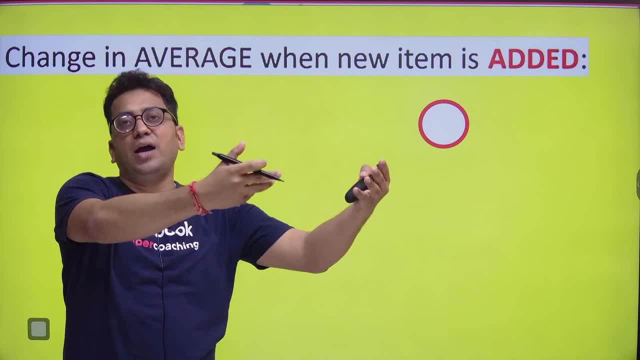 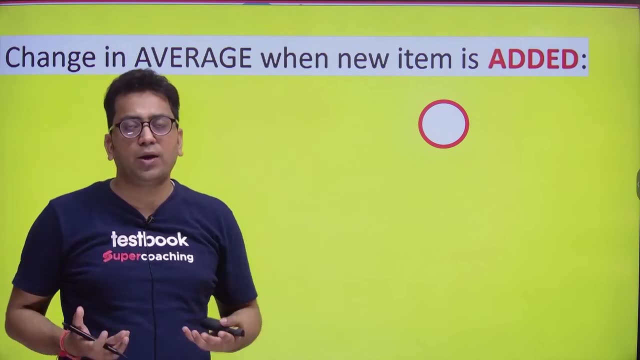 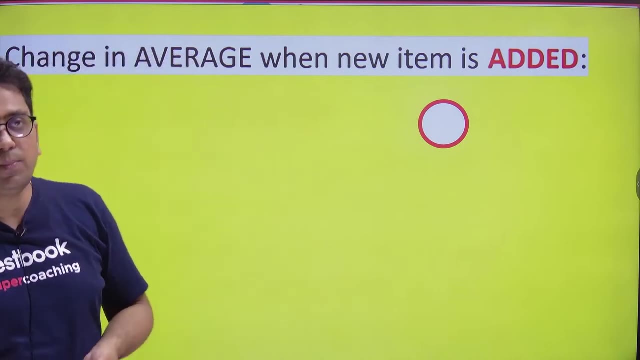 a more number comes for table, we will say number only. here we have said item. so if you add any other item, then what changes come in that? what can come, what changes can happen? that whole concept I want to discuss with you. are you all ready once comment. 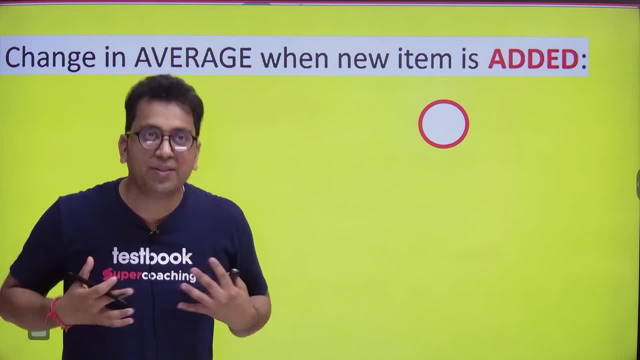 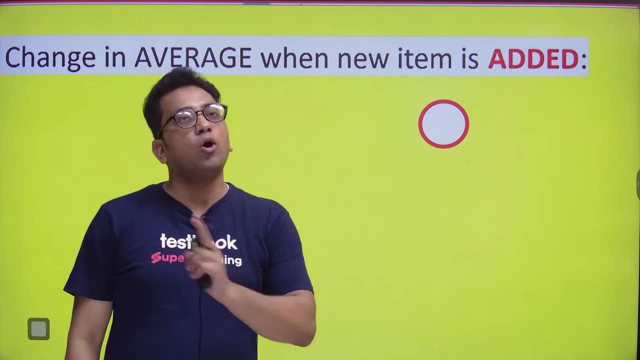 in comment section, all children will write: yes, sir, we are ready, we are ready now. if you understand this concept, then you will look at these questions and you will never make a mistake. once, quickly, in comment section, all will write with heart and smiley: yes sir, ready, ready, ready. 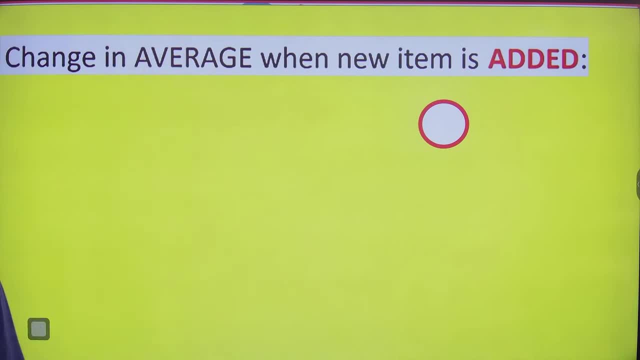 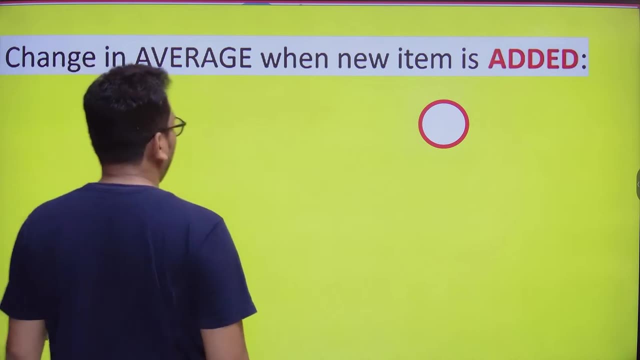 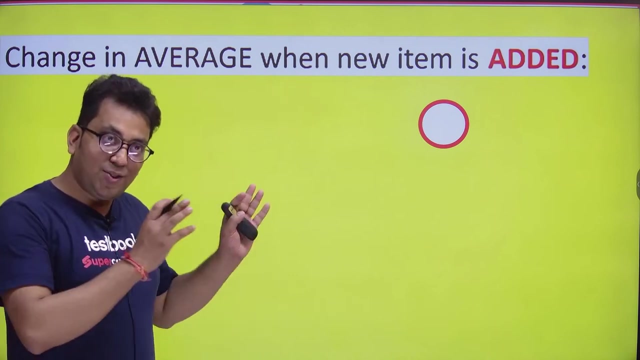 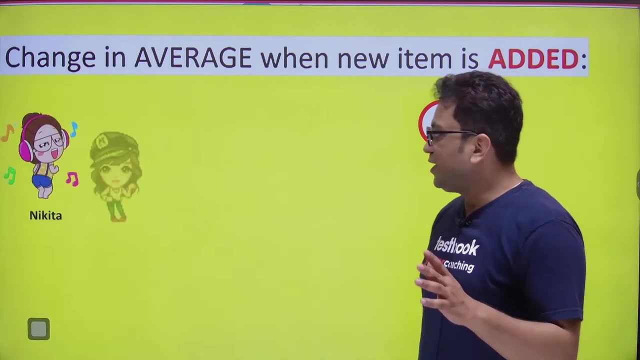 we are ready, completely ok. answer is: no one understands my feeling. don't let them understand. you understand yourself. that is enough. now you understand the math. ok, come here, all are ready. ok, so we have called lion here. see one, two, three and these four. we have called these four lions. 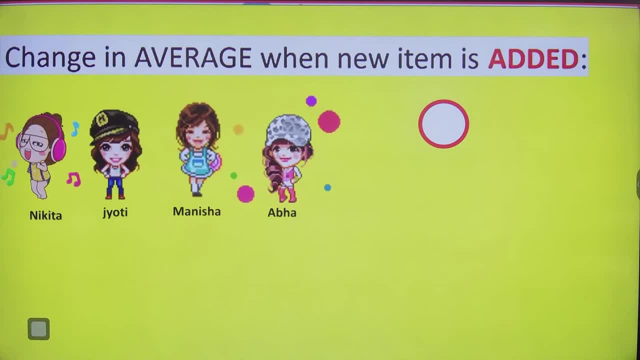 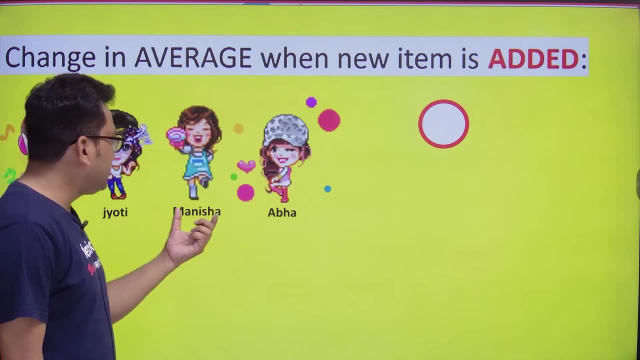 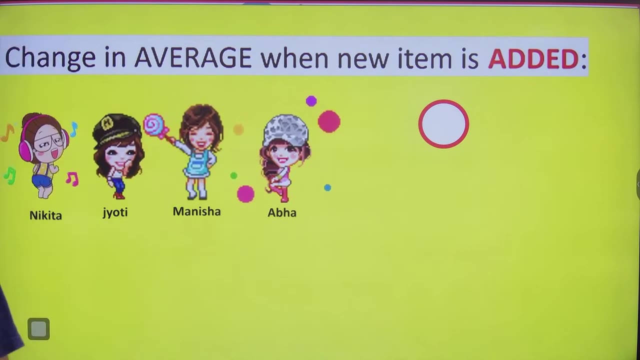 see the name of these four lions. see the name here. one is Nikita, who is dancing here, our lion is dancing. second is Jyoti. third is Manisha right and fourth is Abha. so we have called four lions here. we have assumed that all of them have some amount. 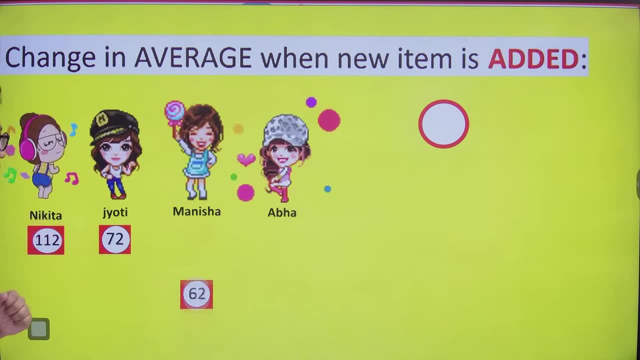 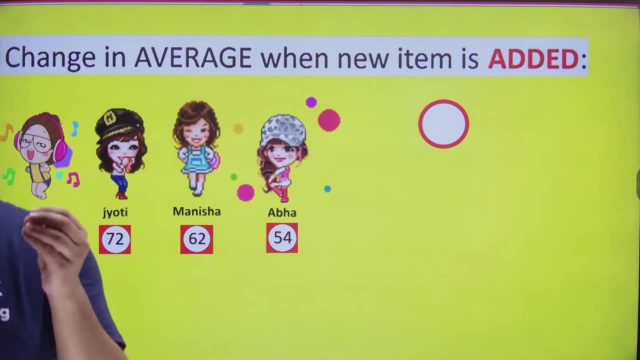 suppose they have 112 rupees, they have 72 rupees, they have 62 rupees, they have 54 rupees. now I want to know from you- I think every child can answer that- what will be their standard. tell me quickly what will be their standard. 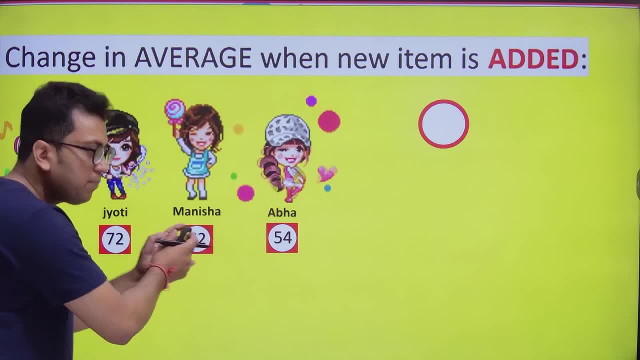 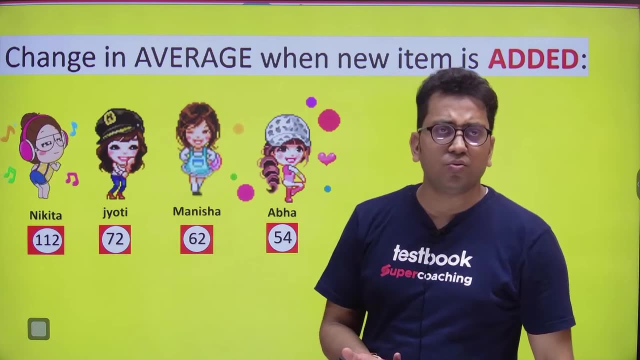 how will you find out their standard? all of them will join. all of them will join and they will divide the numbers. so there are four numbers. divide them into four. it is a simple thing, sir. so, brother, four, two, six, two, eight and two, ten, ten has zero. 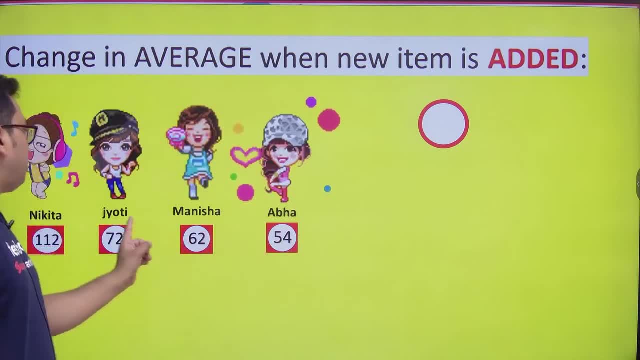 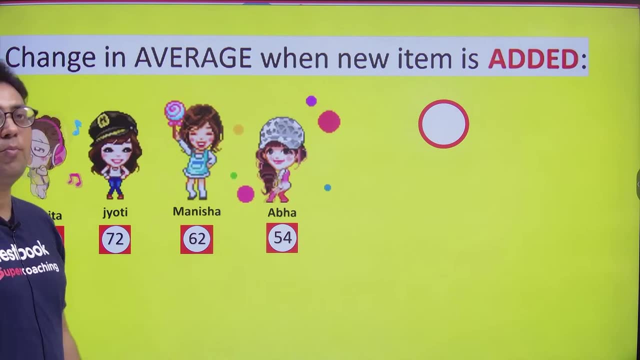 one is achieved, five, one, six, six, twelve, seven, nineteen and one, twenty. twenty has again zero. two is achieved, two is achieved, one has come three. so, brother, three hundred has come, and we will divide three hundred into four, we will divide three hundred into four. so how much will be the rate? 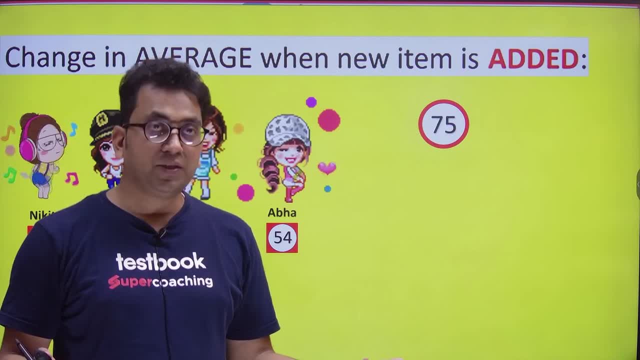 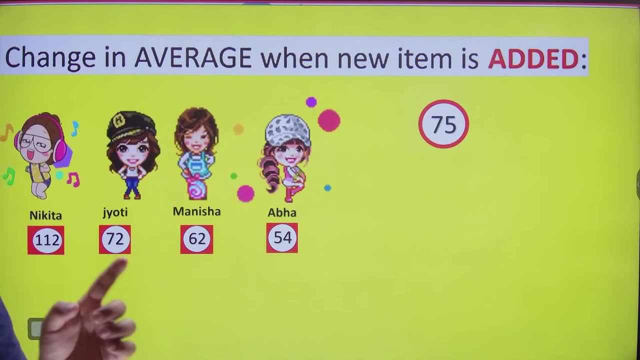 seventy-five. how much will it be? seventy-five, so how much is our rate? seventy-five has come. tell me quickly, are you able to understand all this? okay, Ashok is saying: we are not ready. sir son, come ready, come wear clothes. why did you come like this? 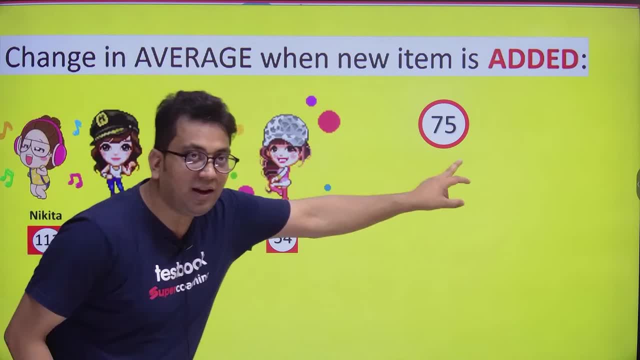 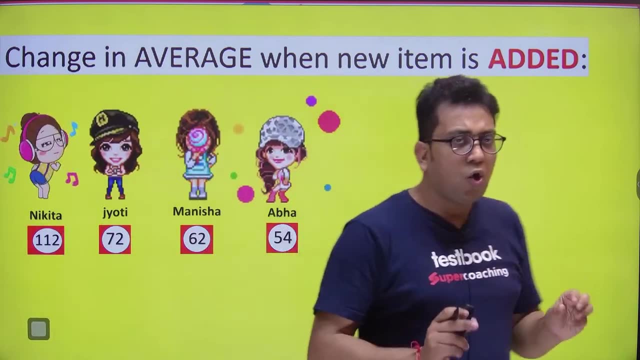 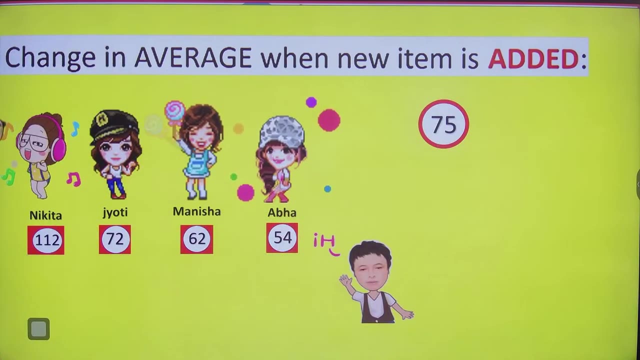 come till here, did you understand? so seventy-five, our rate has come. these four lionesses are very happy. they are very happy, they are playing games and the rate they get is seventy-five. now, brother, one of these lionesses has come. our lion, see, son, he is shaking his hand. 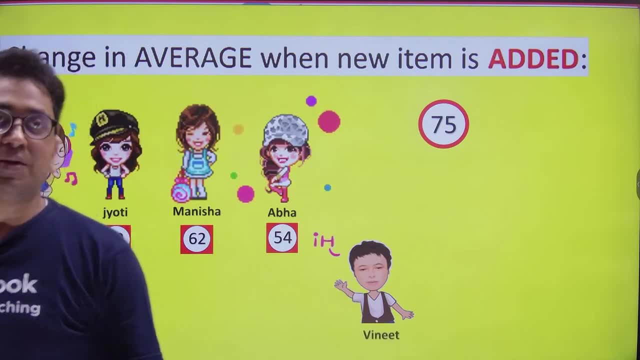 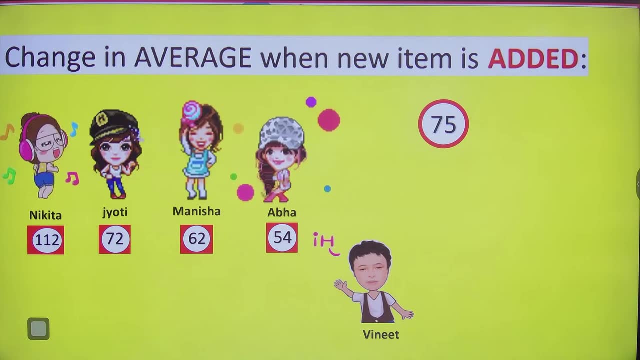 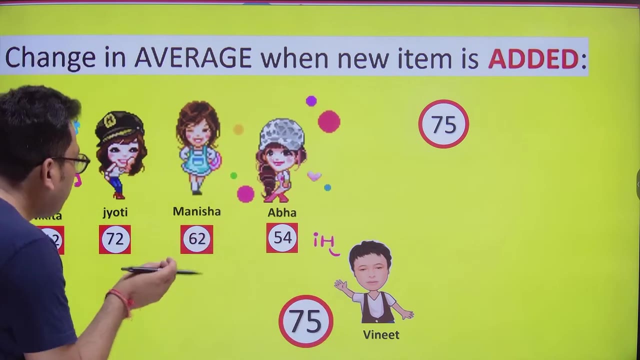 hi, handsome. hi, handsome has come and see the name of this handsome. what is this? Vinit, isn't it? what is the name of our handsome Vinit? now understand my thing carefully: Vinit has brought seventy-five rupees with him. pay attention to the thing: Vinit has brought seventy-five rupees with him. 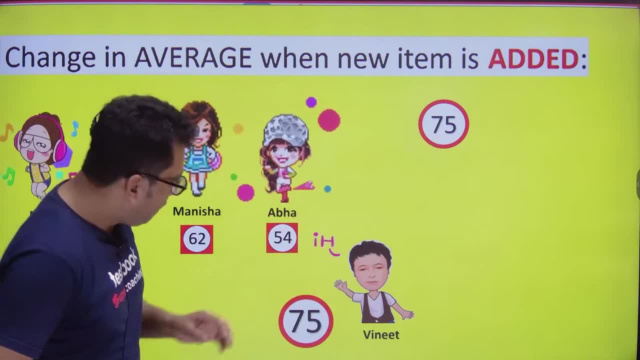 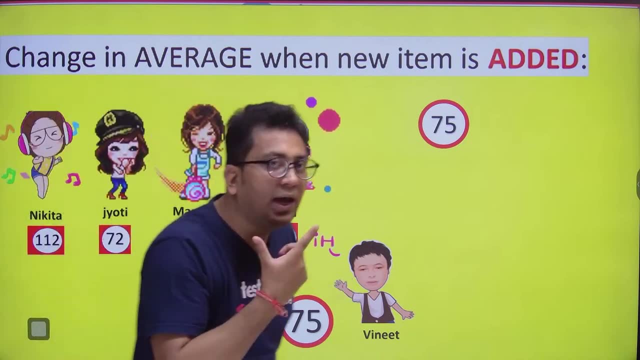 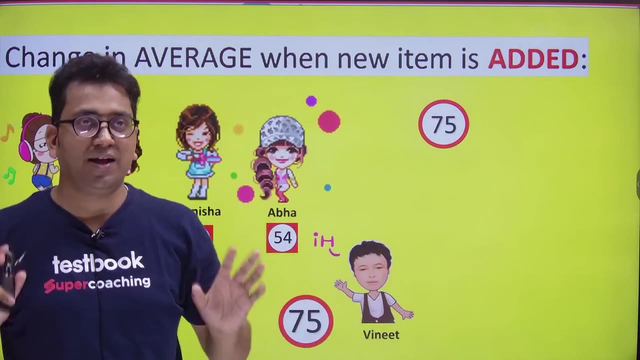 I am saying that the rate of all of them is seventy-five, and Vinit has brought seventy-five rupees. so you tell me that on their face, will you see happiness, will you see sorrow or any feeling or any reaction will you see? so do you know? 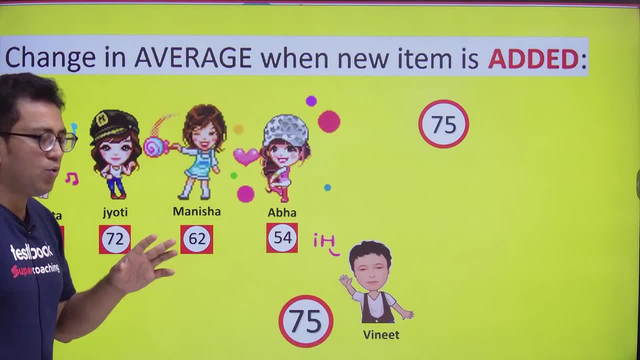 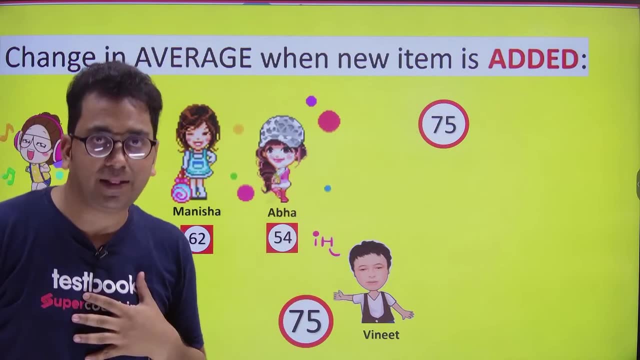 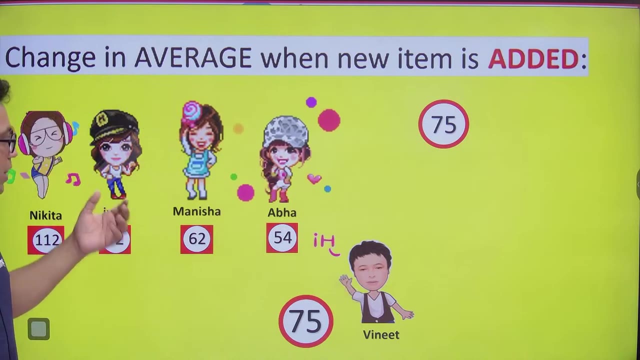 what you will say. you will say, sir, tell me one thing: all of them have seventy-five, seventy-five, seventy-five. what is the rate which is per head? we assume that all of them have seventy-five. in reality, some of them will have less, some of them will have more. 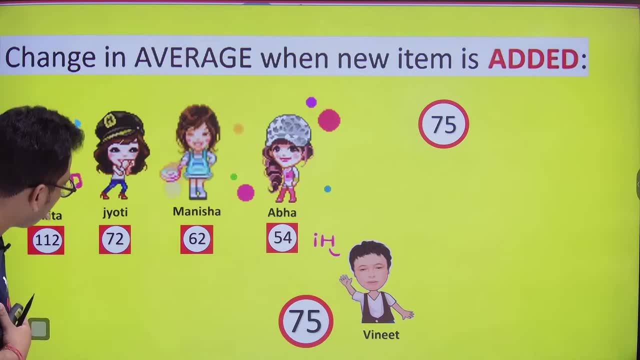 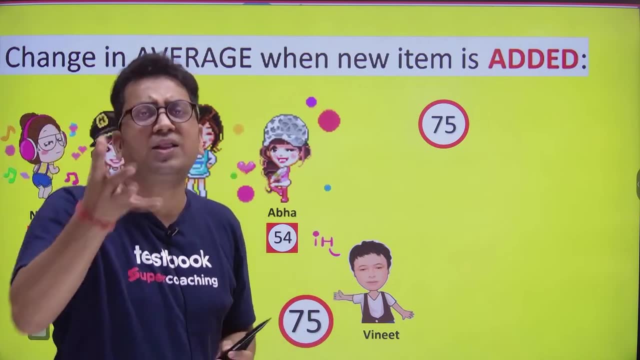 if the rate is seventy-five, then we are assuming that all of them have seventy-five, seventy-five. if Vinit also will bring seventy-five, then on their face will not even see a trace. do you know what they will say, brother, we have seventy-five, you have brought seventy-five. 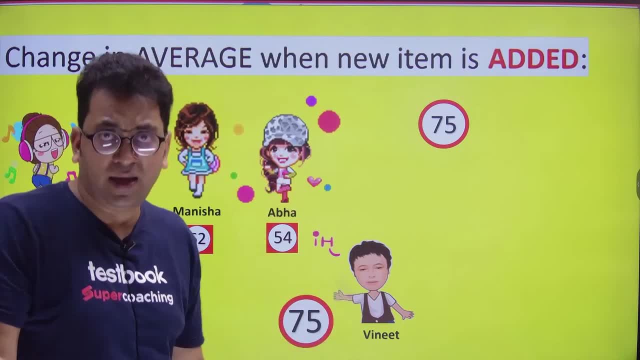 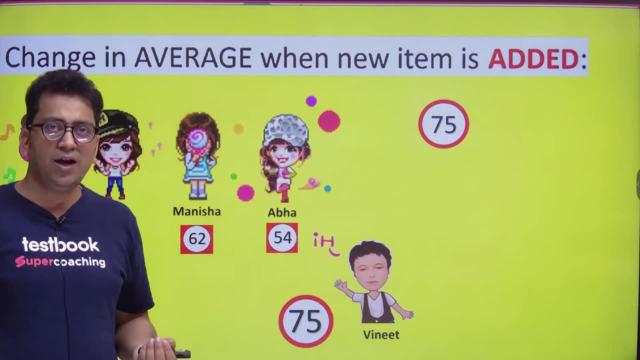 then come to the group and sit. why are you saying hi hello to us, hey brother? why are you saying hi hello to us, hey brother? we have seventy-five already. you will also bring seventy-five. yes, see, one child said: there will be no difference. there will be no difference. 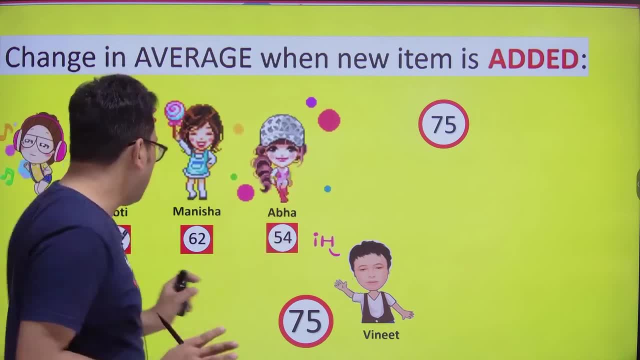 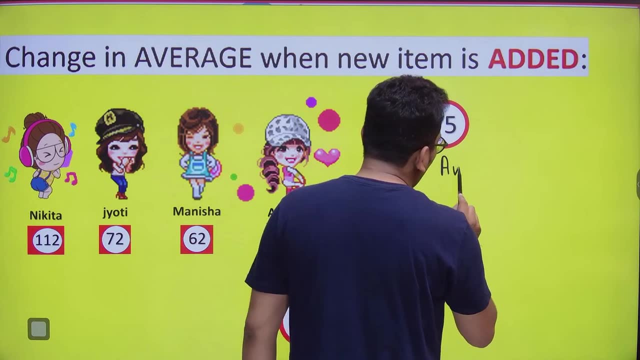 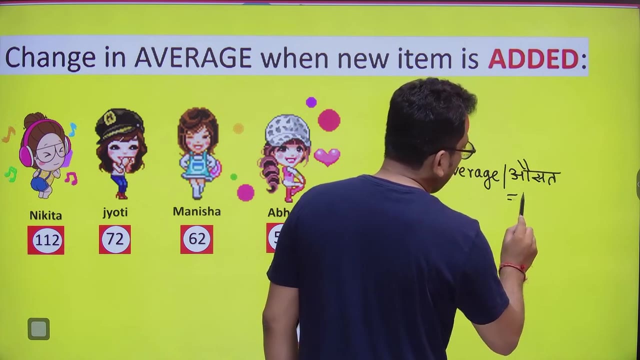 because this is also seventy-five, this is also seventy-five, it is perfect. that means, if we talk here, you can write in your copy that the average, that is the rate, it will be equal. do you agree, all of you? yes, sir, the rate will be equal, it will be equal. 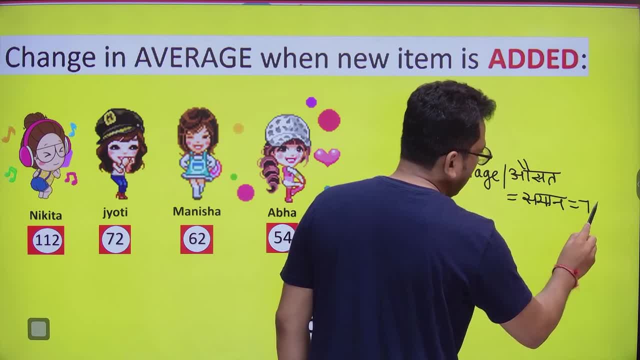 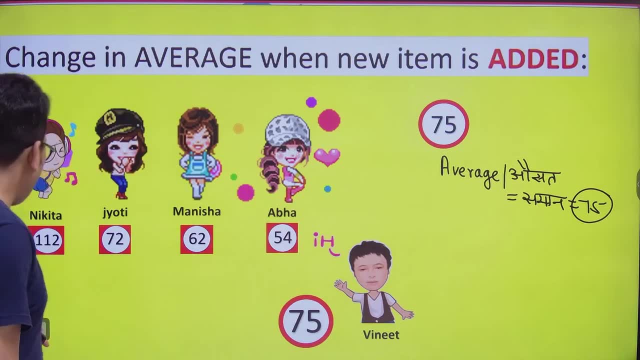 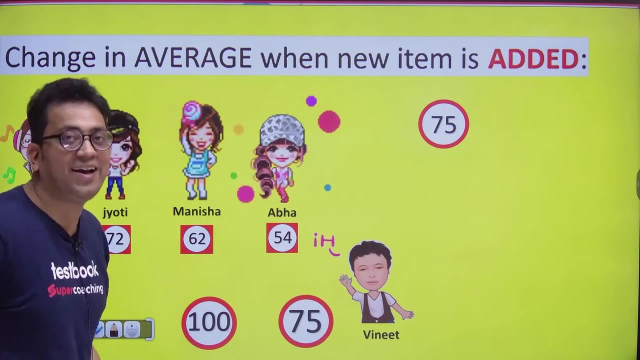 there will be no effect on it. it will be seventy-five only. ok, note down this thing in your copy, because now it will be removed. this was the first case. this was the first scenario. ok, now let's assume that they brought hundred. they brought hundred, they brought the note of hundred. 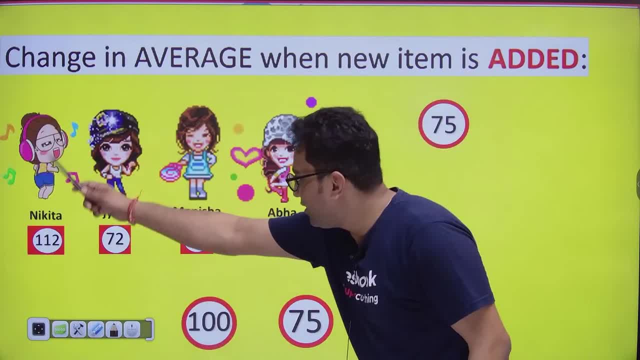 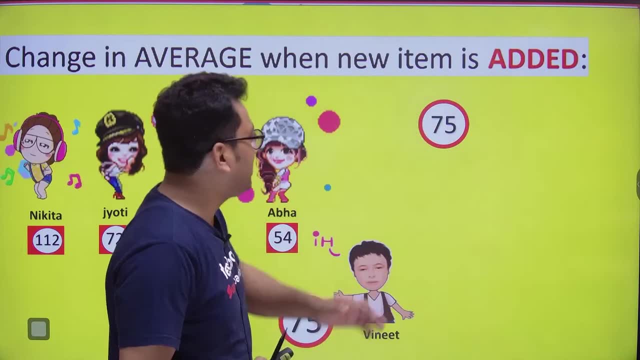 now tell me, son, on the face of these four lionesses, will you see happiness or not? absolutely, absolutely, why? because their average was seventy-five, but the head was seventy-five. now they brought the note of hundred. now everyone will be happy. do you know what they will think? 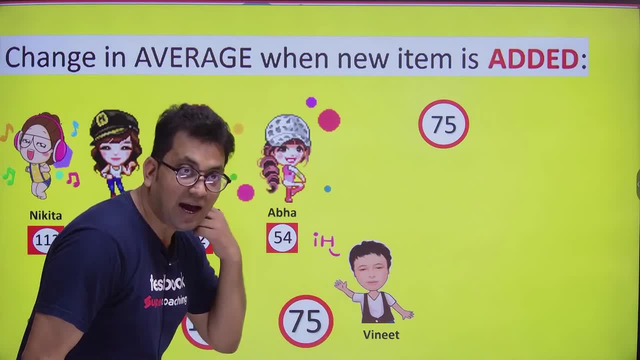 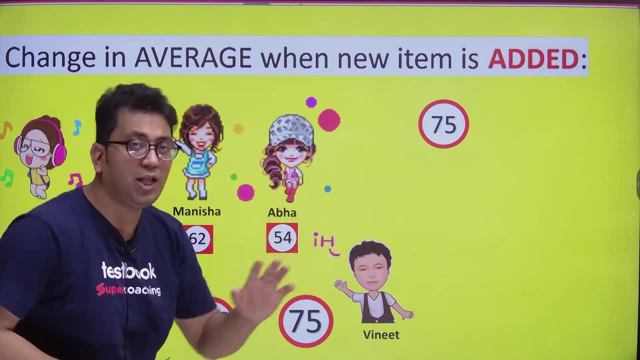 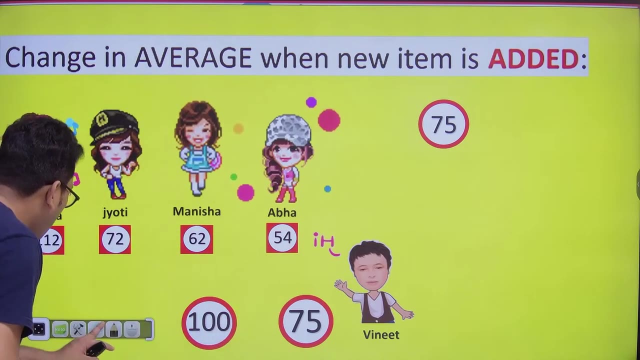 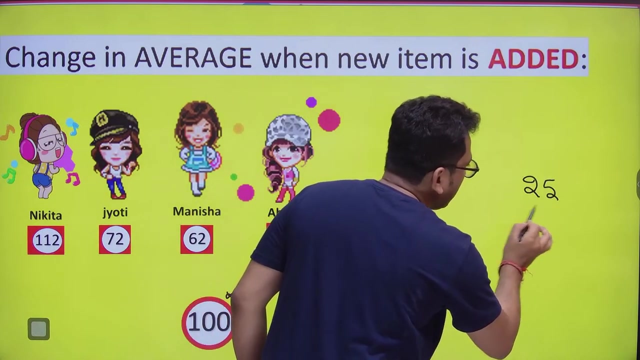 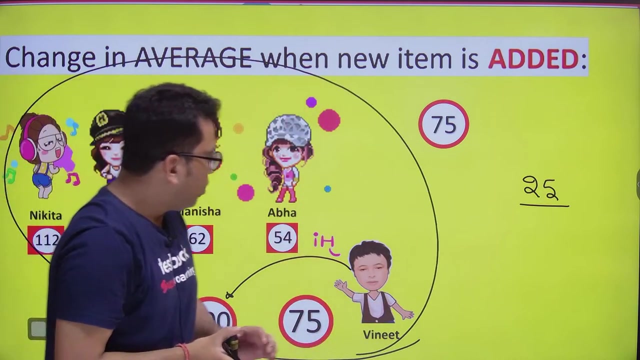 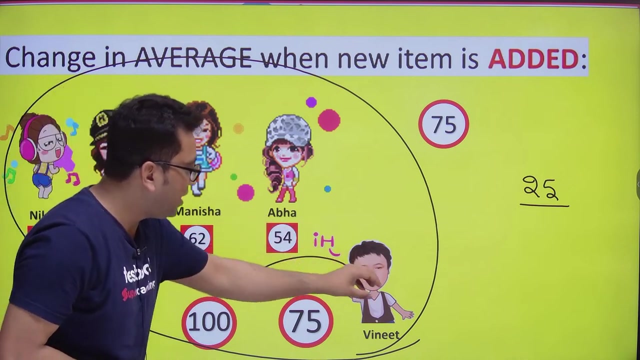 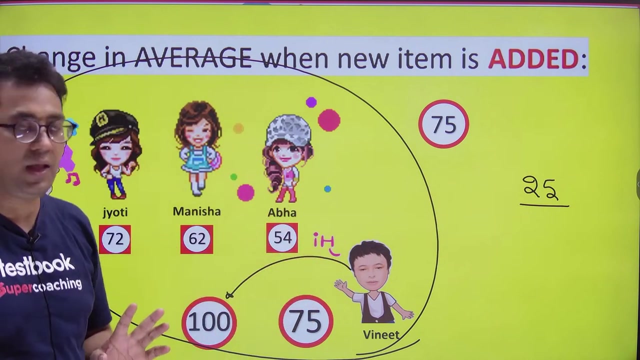 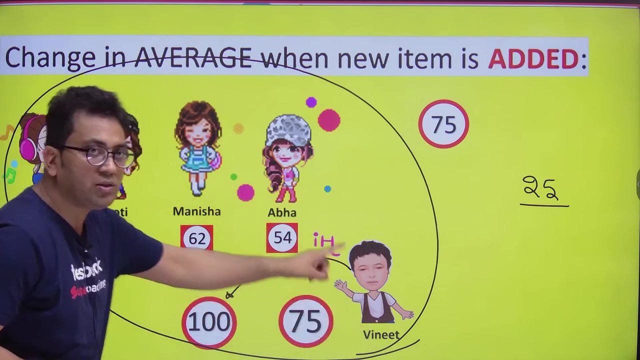 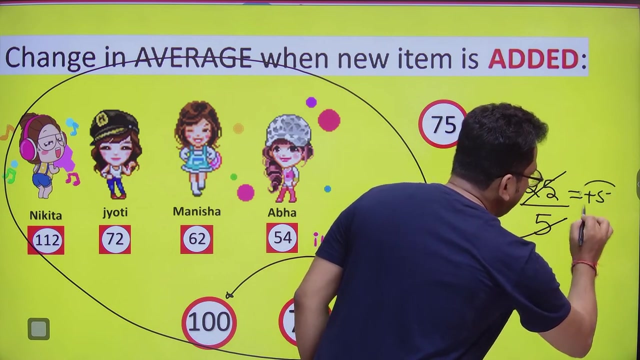 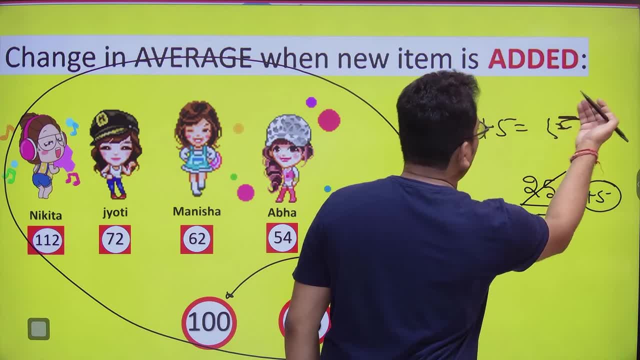 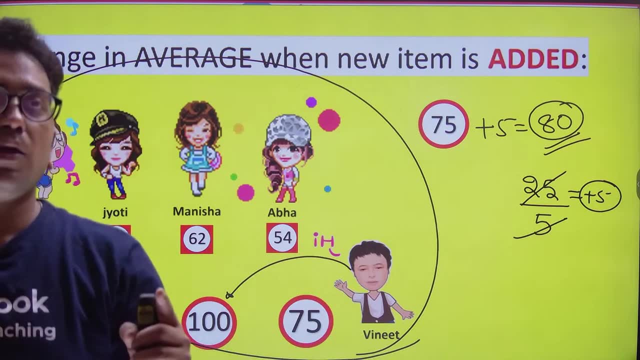 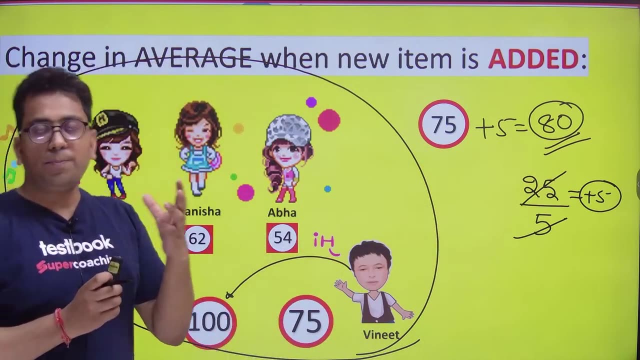 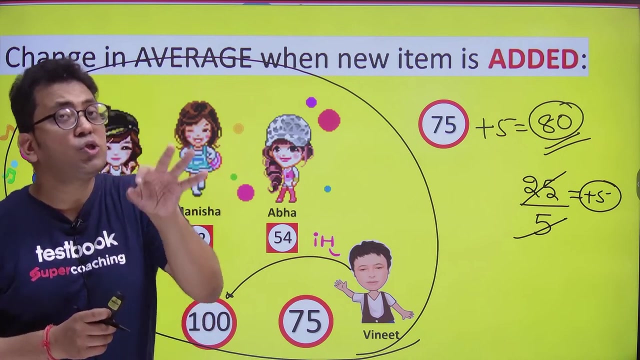 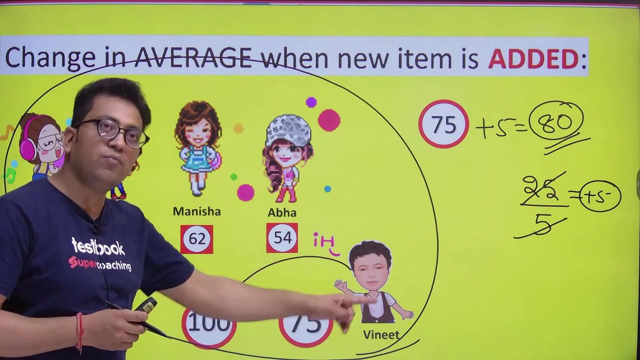 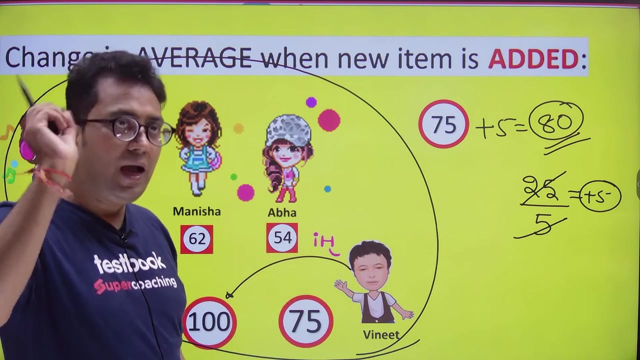 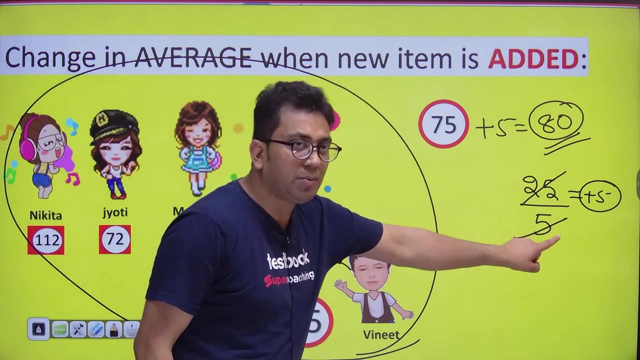 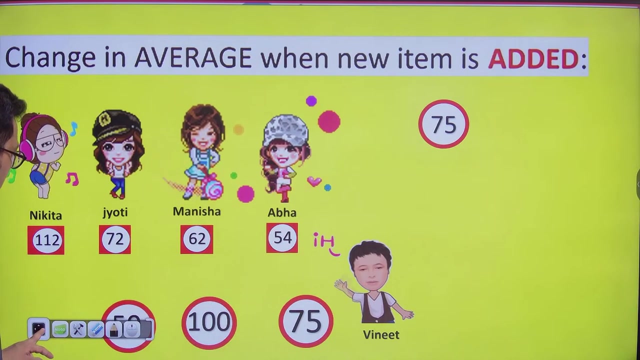 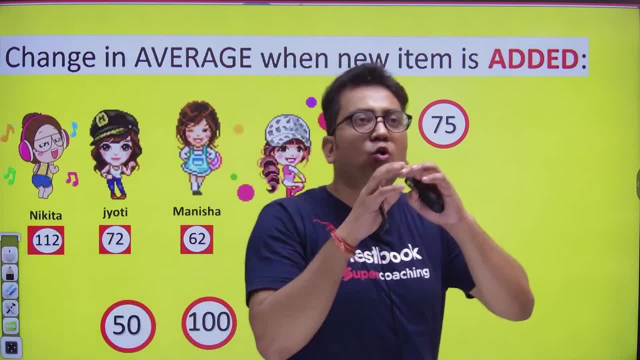 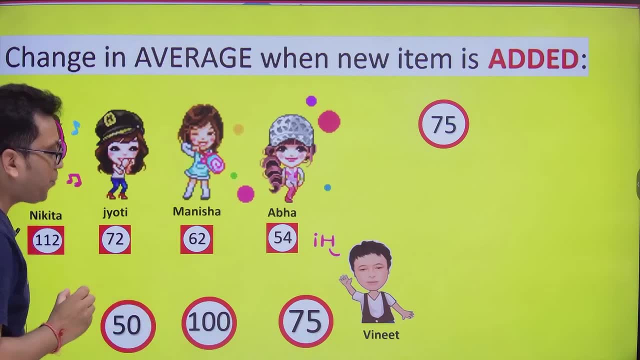 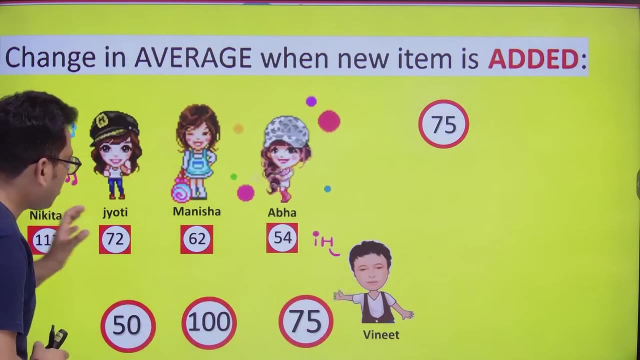 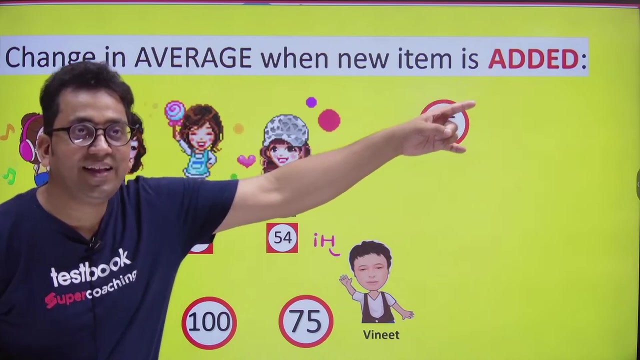 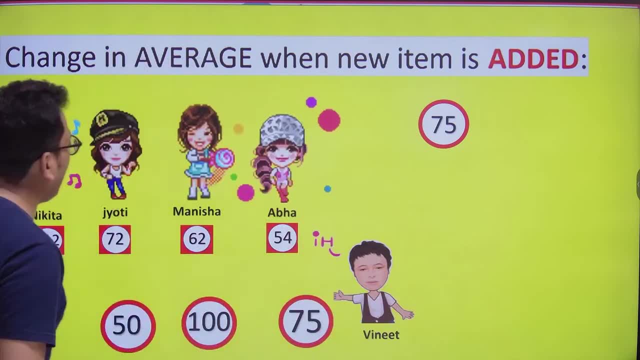 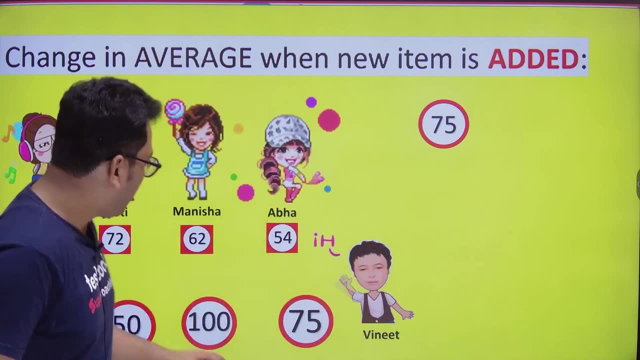 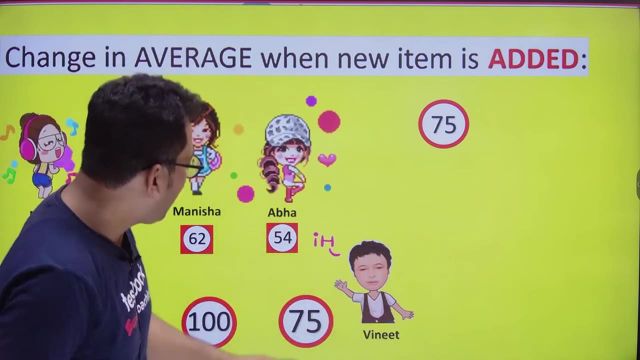 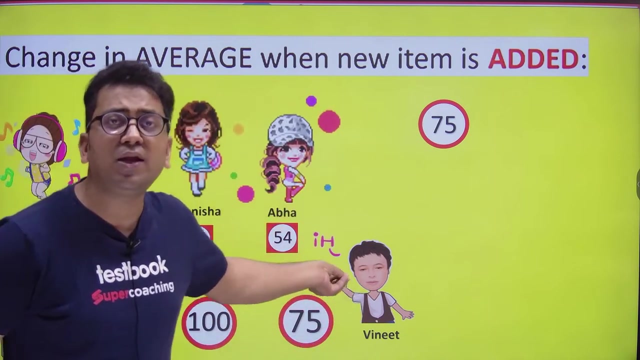 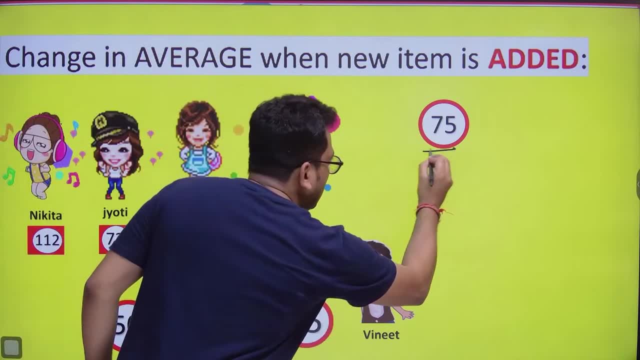 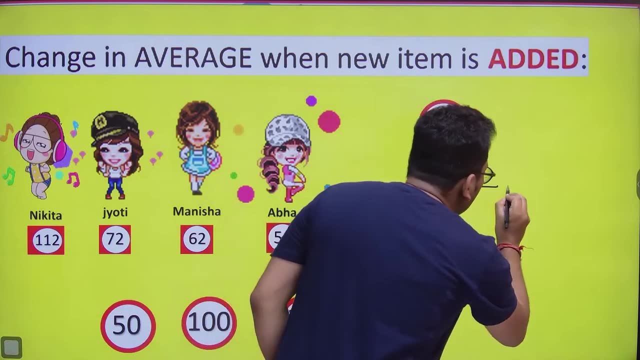 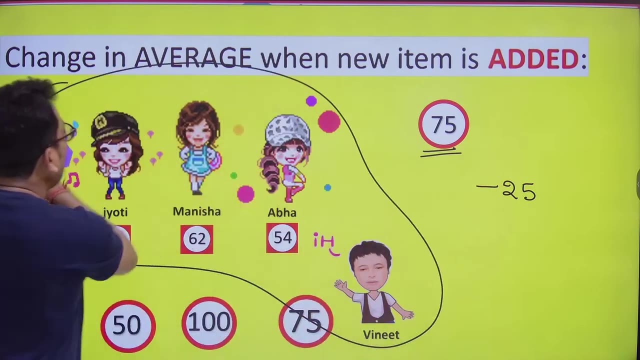 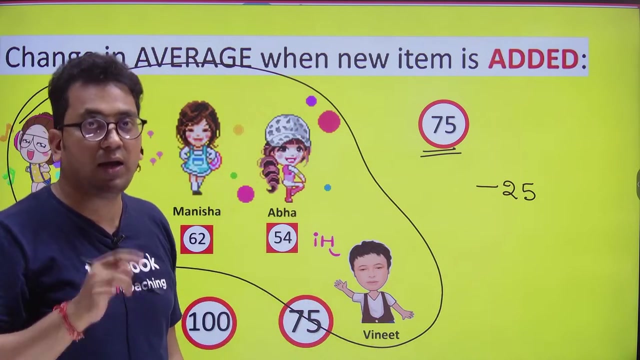 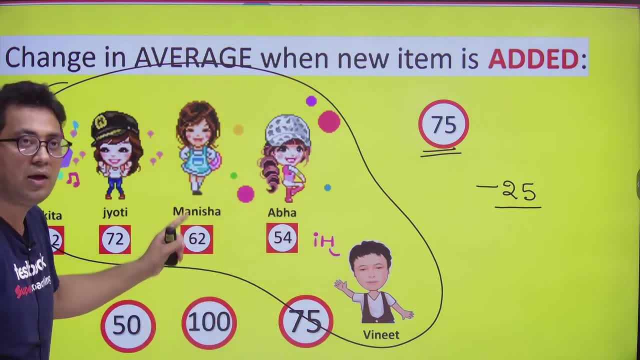 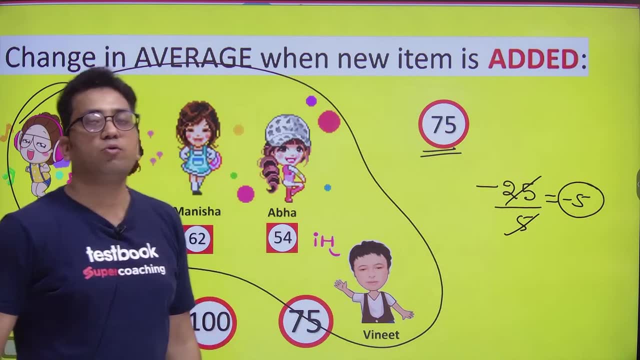 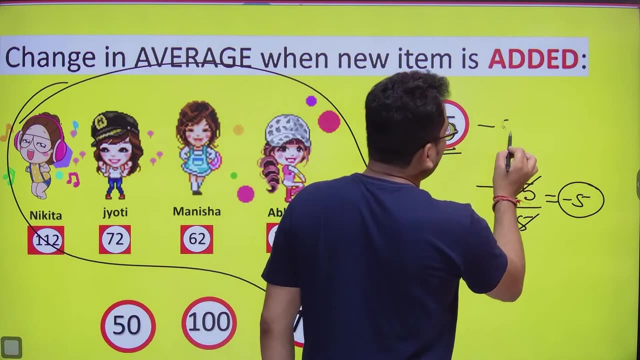 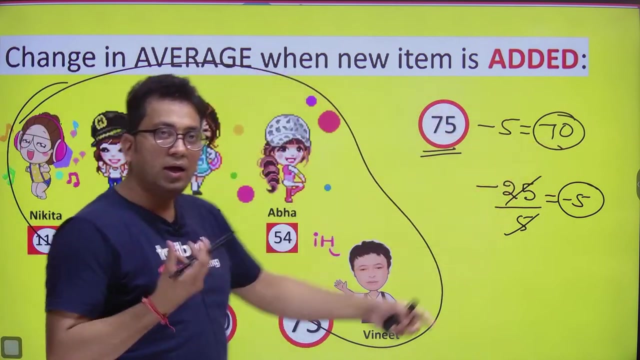 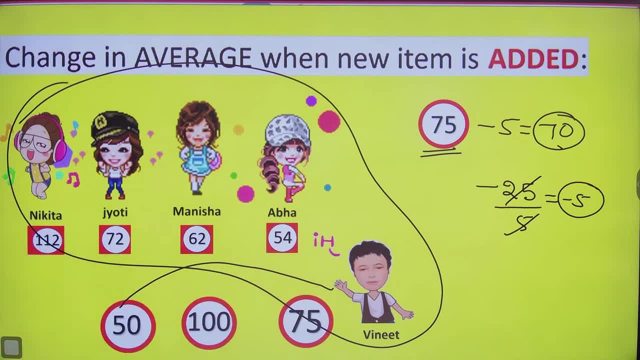 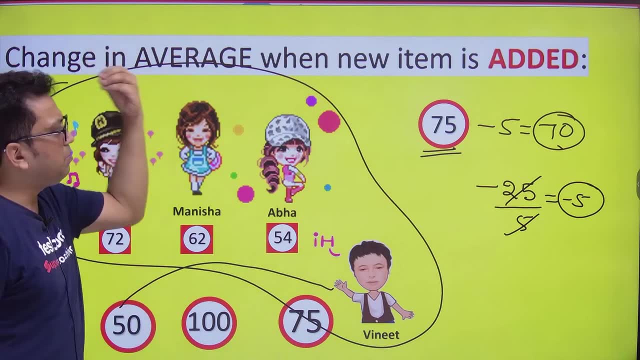 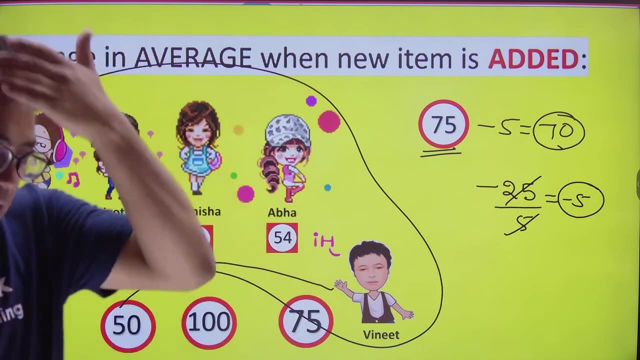 If you have understood this concept, then you can go ahead and ask any question. You will be the one to answer. You will be the one to answer. Tell me quickly, did you understand? Did you understand? Is it clear? Now come to the questions. How are the questions being asked to you? 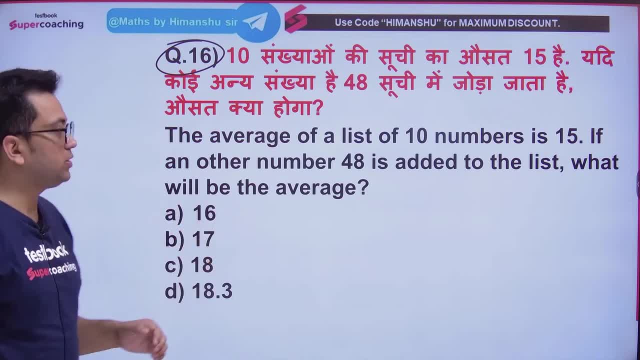 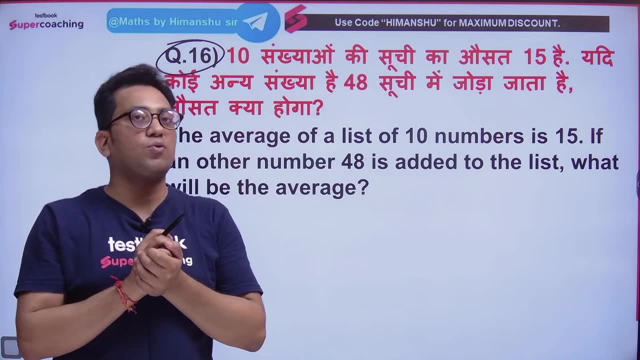 Question no 16 is in front of you, Question no 16 of today's session. What is the ratio of 10 numbers to the list of numbers? Now see the ratio. What is the ratio of 10 numbers to the list of numbers? 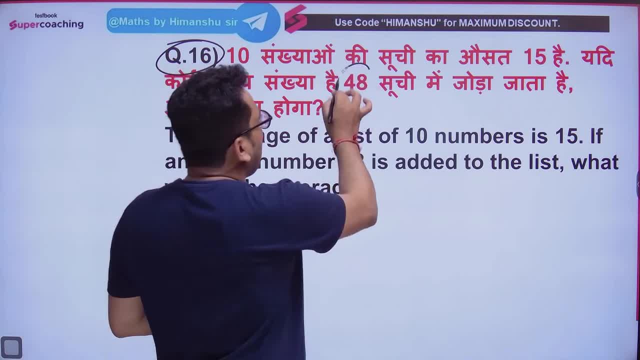 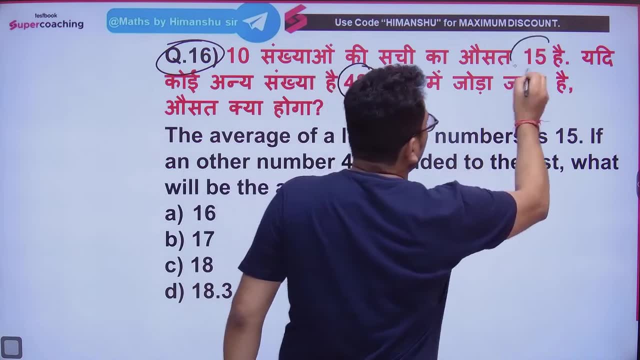 If the other numbers are added to the list of numbers, then what will be the new ratio? It has come more than the ratio. It has come more than the ratio. It has come more than the expectation. They will be happy. How much more is it? 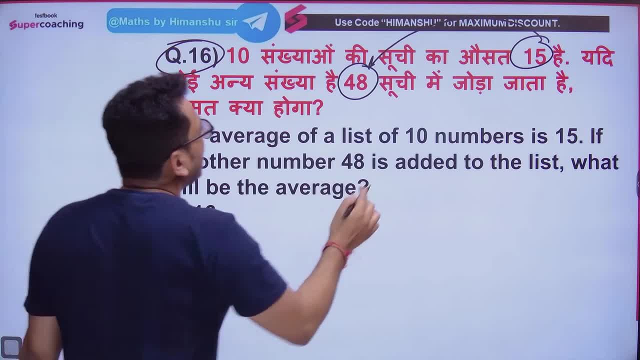 The more it is, it will be equally divided among all. The child will only see how much more is it from 48 to 15.. Sir, 33 is more. It is visible. 5 out of 8 is 3.. 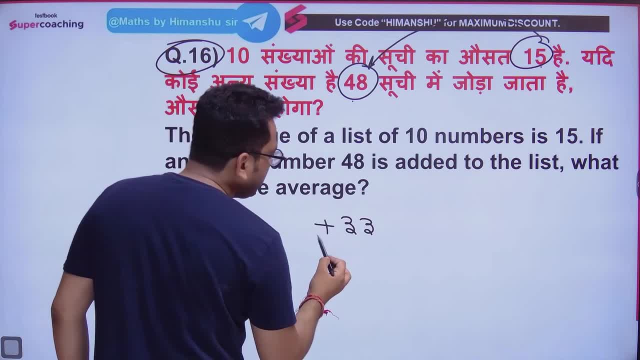 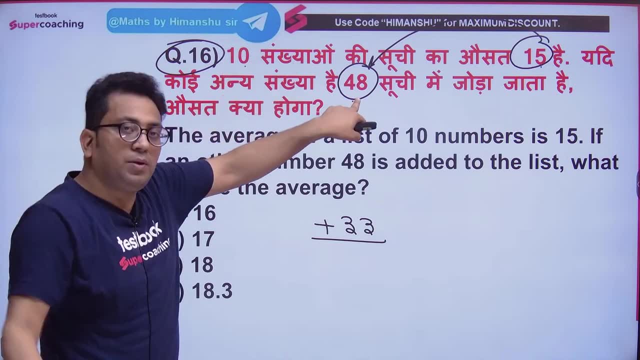 3 out of 4 is 1.. 33 is more And this more the benefit. in how many will it be divided? Sir, earlier there were 10 numbers. 48 was also included in the list, That is now. the total number is 11.. 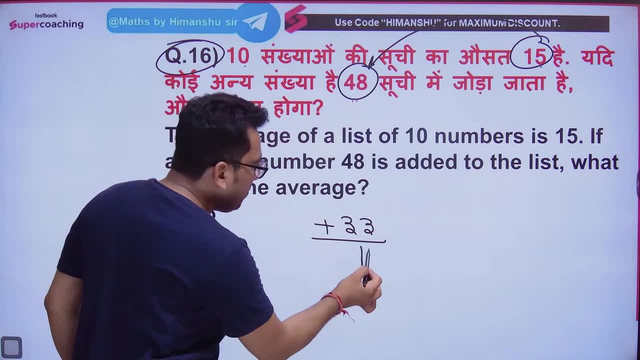 So this is going to be equally divided among 11.. So this is going to be equally divided among 11.. That is, each one will benefit 3 by 3.. That is, the first ratio was 15.. Now each one will get 3 more in it. 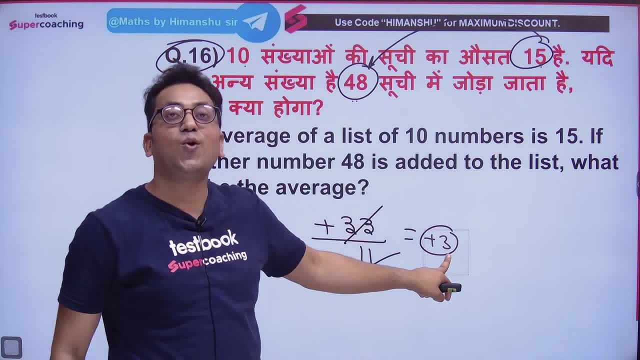 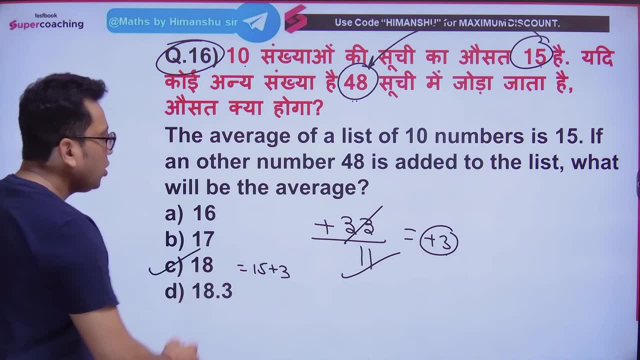 Now, each one will get 3 more in it. Now, each one will get 3 more in it. Yes, That is now. this will be 18.. 15 plus 3 is 18.. Tell me if it is clear or not. 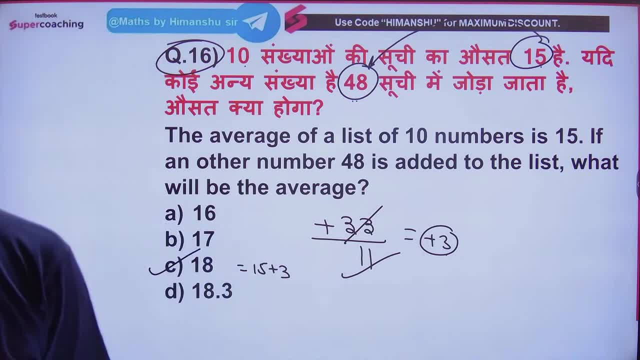 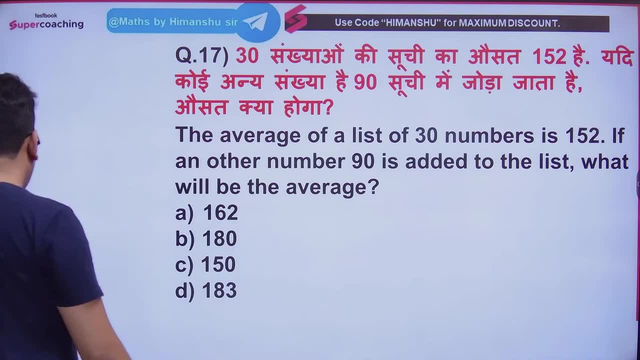 Tell me if it is clear or not. Is it clear to everyone? Is it understandable? Is it fun? Let's move forward, Answer this question. Try it. Let's see how many children are able to answer. Tell me what will be the answer. 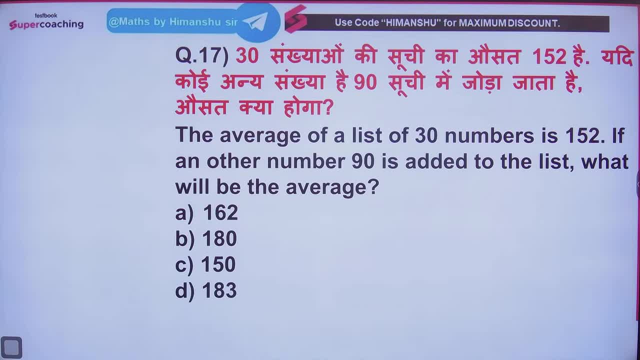 Your likes and shares today are very good. Your likes and shares today are very good. Your likes and shares today are very good. You have good kids. Answer the question. What will be the answer? What will be the answer? Did you get the answer? 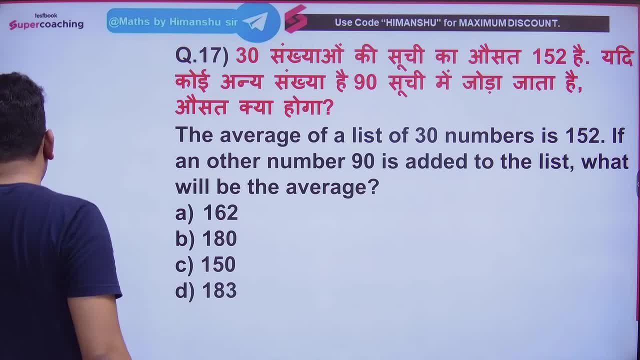 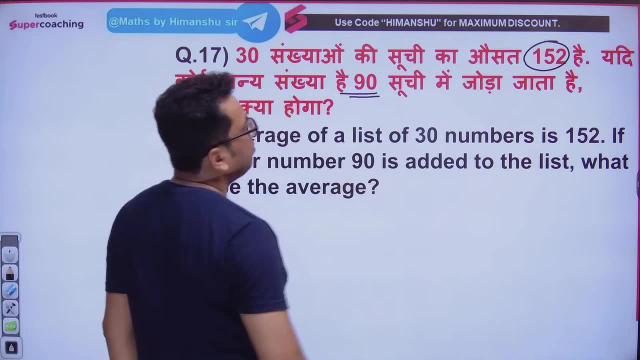 Let's see How much is the average of 30 numbers. It is 152. How much is the average? It is 152 If we add it to 90 numbers. Now tell me, is it less or more? You will say it is less. 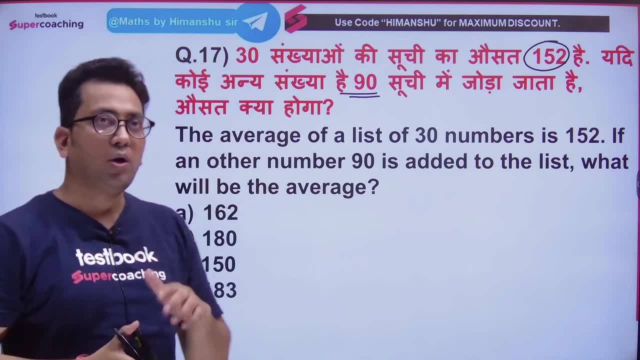 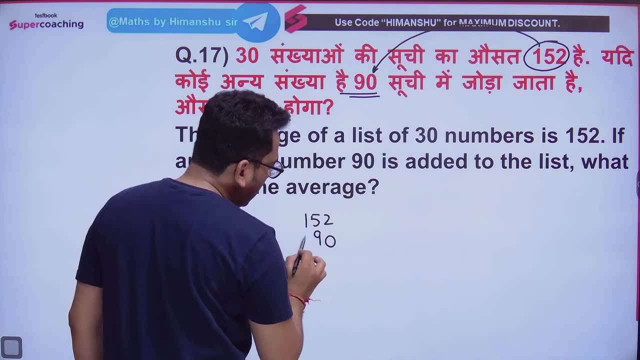 So see how much is less. The less it is, the less it will be. So from 152 to 90. So see how much is less, Isn't it? Decrease it and see how much is less It is. 62. 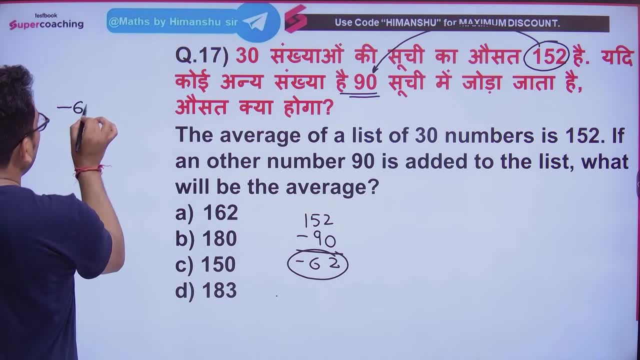 So the difference of 62, It will be equal to all. How many? Earlier it was 30, Now it has come to 90 too, That is, 31 numbers have been made, And if 62 is equally divided in each, Then each one will have a difference of 2. 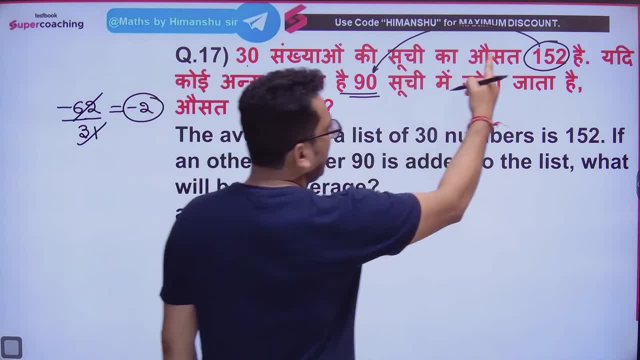 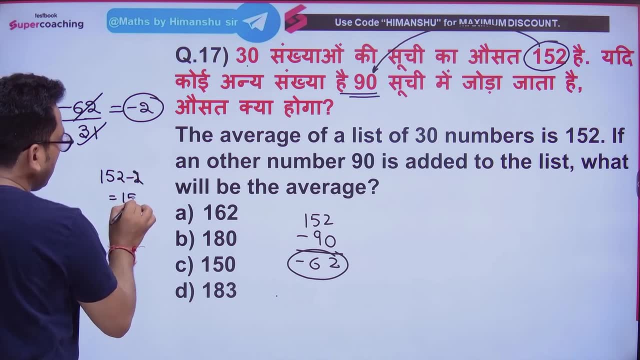 Isn't it? That is, the previous average was 152. Now there will be a difference of 2, That is, the average will be new. How much? It will be 150, That is 150. The problem is our answer. In my opinion, every child will be able to answer. 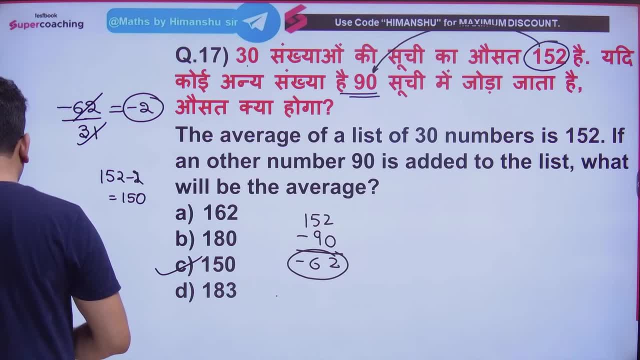 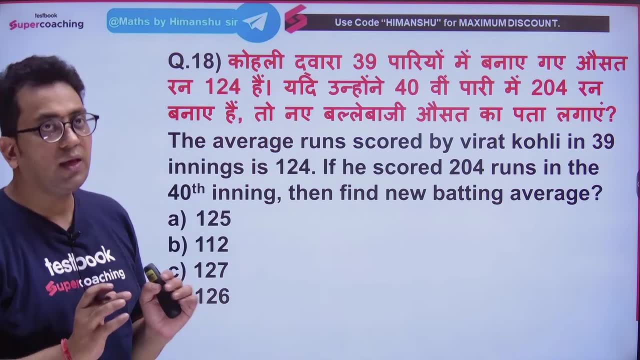 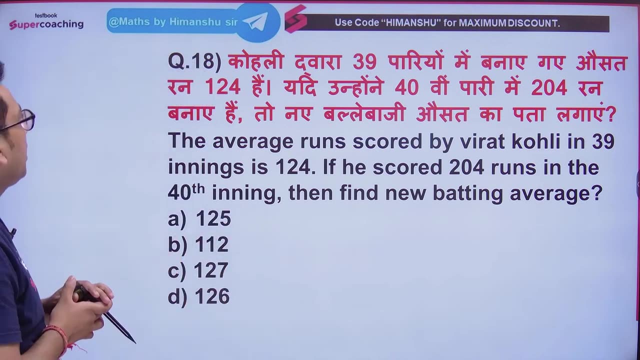 Now I am moving on to the next question, Question number 18. You can join whoever wants to take the BPSC batch From this week. in this batch, Live practice class sessions are starting. Okay, And I will tell you the code: Himanshu, this is the code. 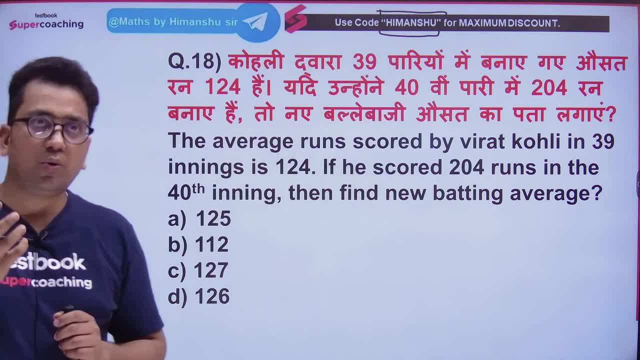 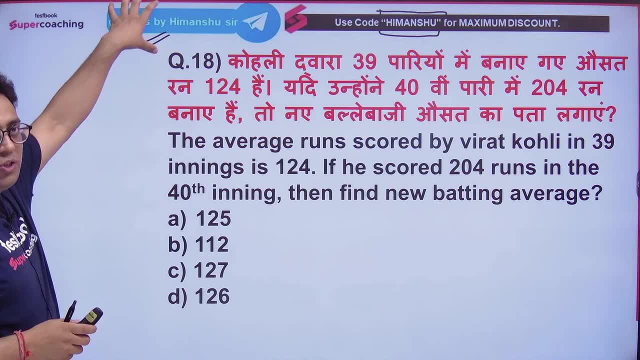 You can apply this code. You can take maximum discount here. Rest any issue, any query? Maths by Himanshu sir Telegram channel. There is a discussion group in it. You can ask me about your doubts there too About the course. Okay, Come on answer quickly. 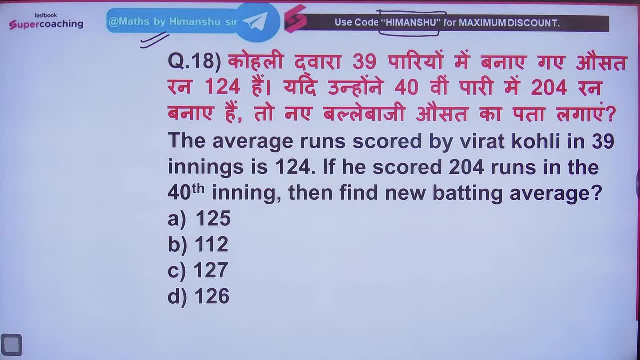 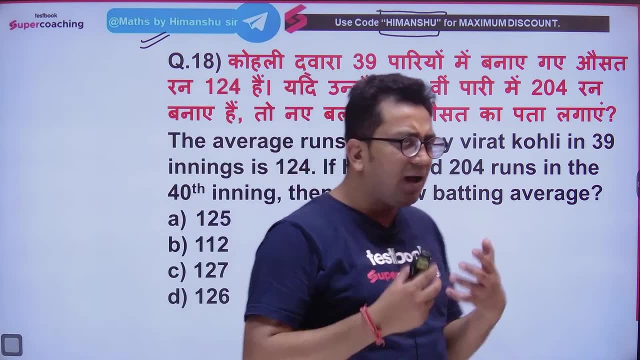 The average runs made in 49 batches by Kohli are 124. If they made 204 runs in the 40th batch, Then what will be the new ball game average? Look at this. So many different questions will be asked based on this Right. Ranandheer Kumar is repeatedly saying that there is no reaction. 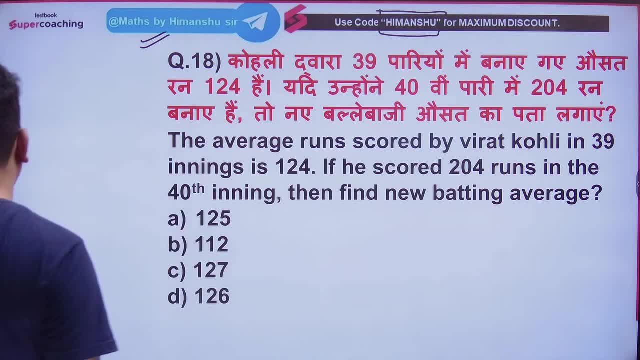 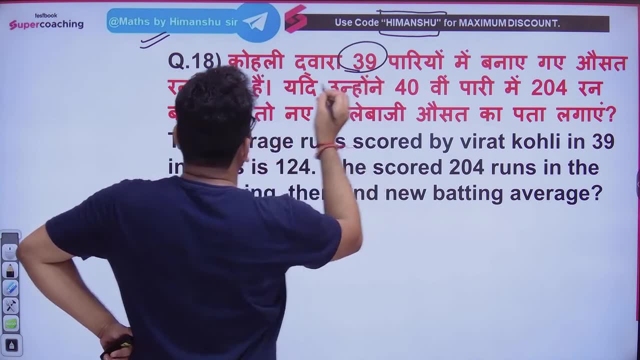 What happened, son? You are repeatedly saying the same comment. There is no reaction. This is your late reaching me. Look here. There were 49 batches. What was their average? 124. If Kohli had made only 124 runs in the 40th batch? 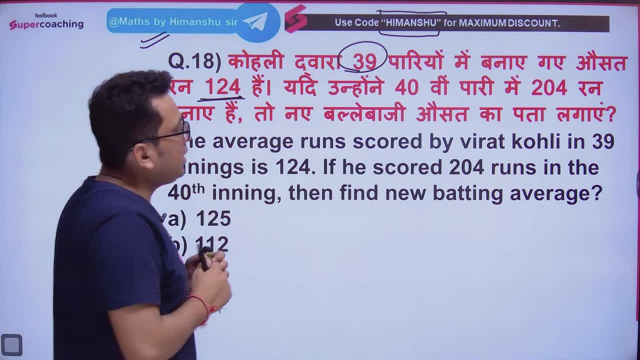 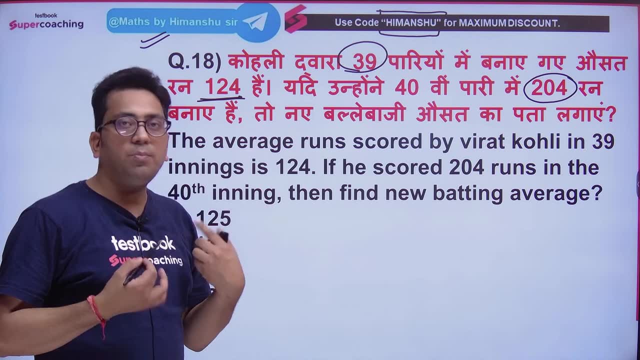 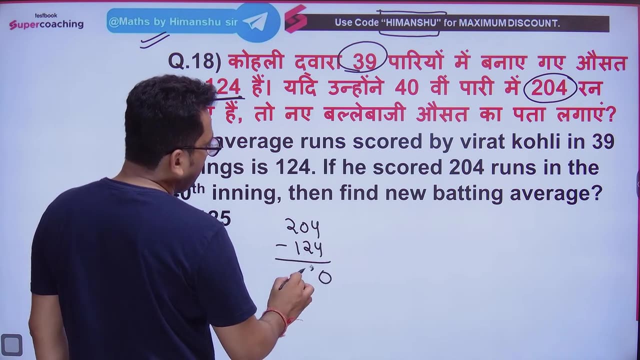 Then there would have been no reaction. But here they made 240 runs. Sorry, 204 runs That means more runs, So the average is going to increase. So we will see how many more have been made. From 204, 124 is reduced, So we will know that more than 80 runs have been made. 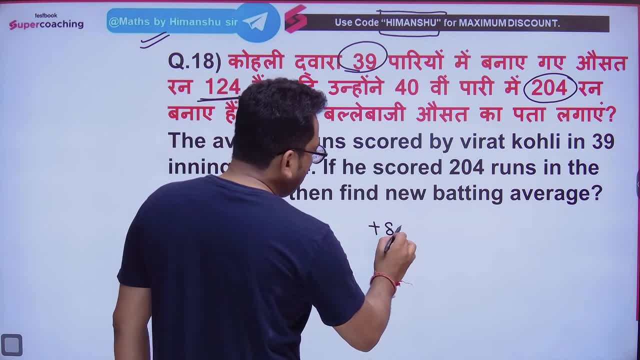 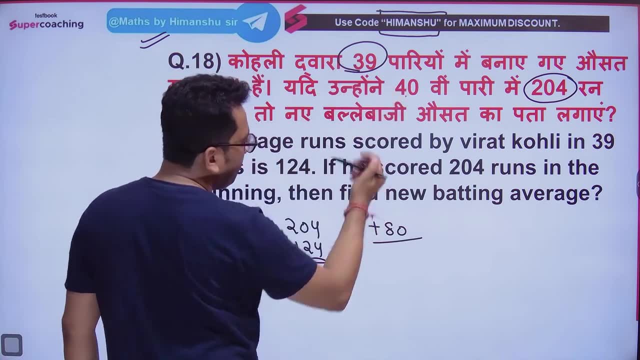 And the benefit of these 80 runs In all the innings, In all the batches. It is going to divide equally. The first was 49th batch. Now the 40th batch has played more, That is, the total batches have become 40. Each batch has more than 2 runs. 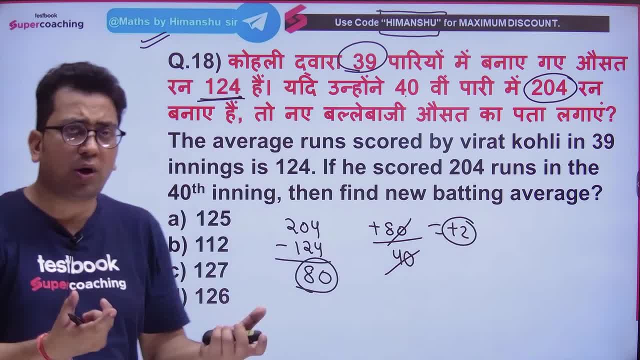 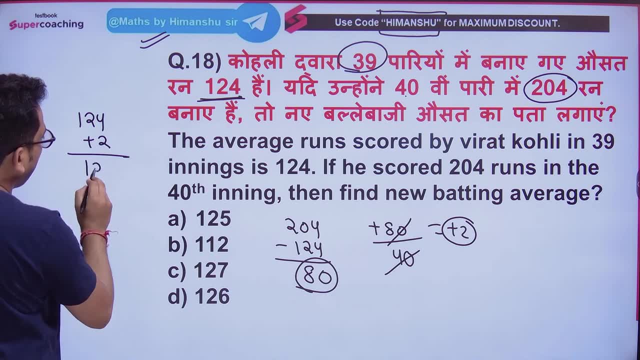 So we are going to get more runs. If you run from 80 to 40, 2 runs have been made. So the previous average of 124, Now there are going to be 2 more in it, That is, the new average will be of 126 runs. 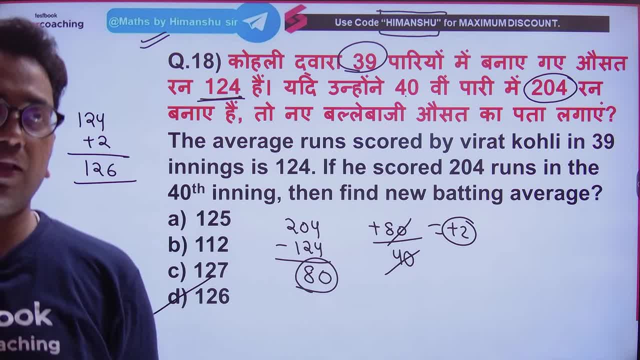 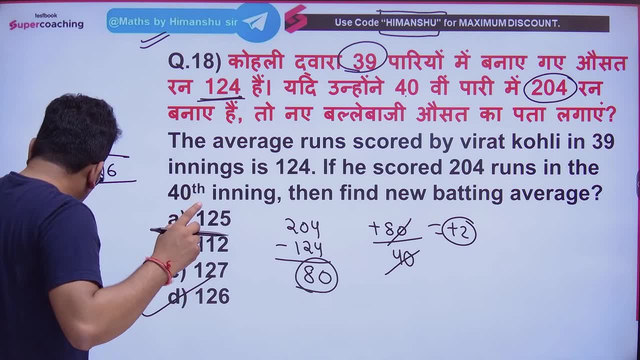 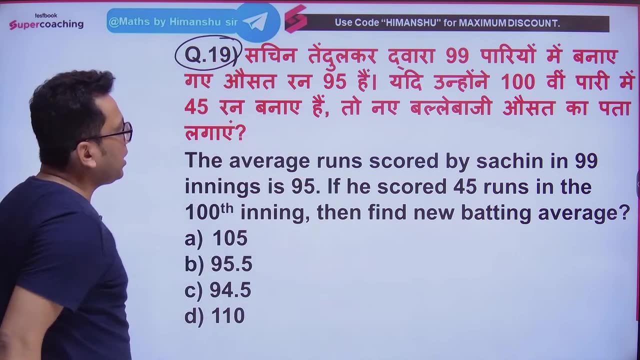 That is option number D. Our answer is going to be: You are understanding. These are the questions Which are of good level, But now you are able to shine Because you have understood the concept. 19th question: Look here, son. What does Sachin Tendulkar do? 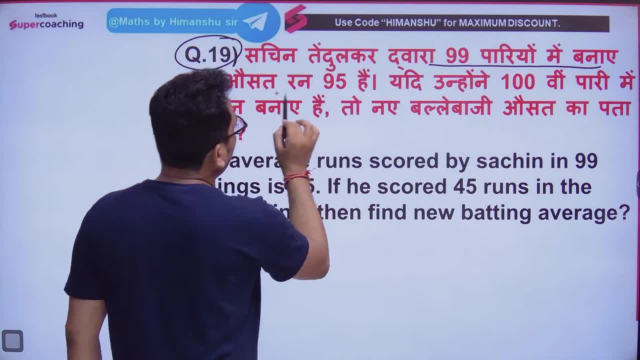 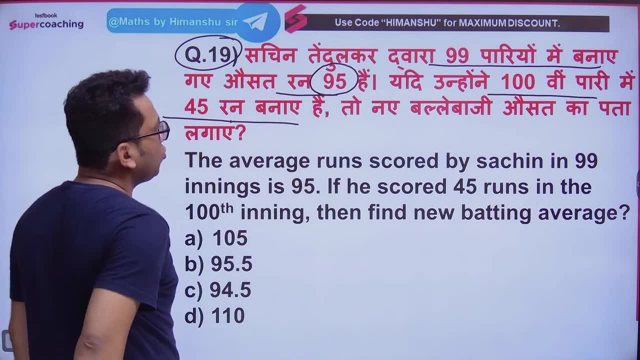 In those 99 innings. In those 99 innings His batting ability is of 95 runs. Ok, In 100th innings He made 45 runs. So you have to tell What will be the new batting ability. Let's see How many children are able to answer. 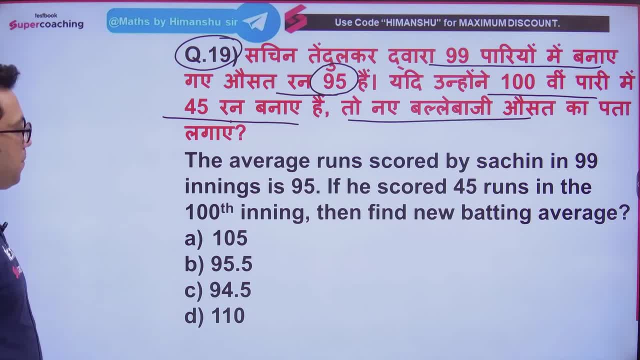 Answer all of them: A, B, C or D. What will be the answer? All of them, Everyone. One time Click on the like button, Son. The session is fun. Like the session. Then one time Click on the like button. Ok, Son, with a lot of hard work. 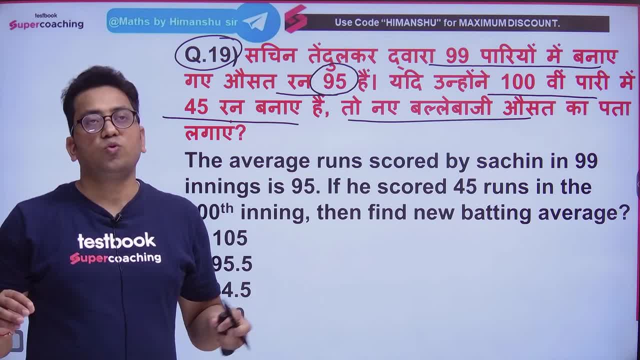 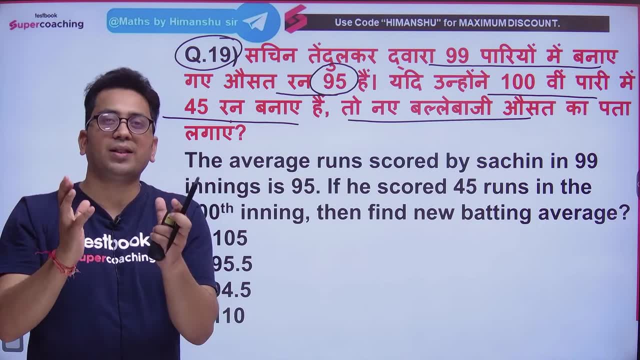 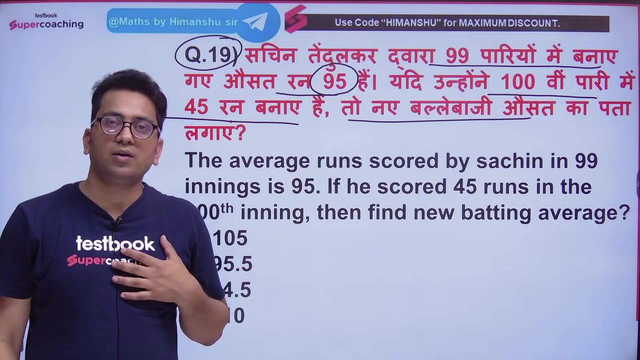 I make content for you. It takes a lot of hard work. So this is your request. You don't have to give anything to it. Don't do anything. Ok, It just tells me how much my child is liking the session. The comments that you guys get are my Guru Dakshina. 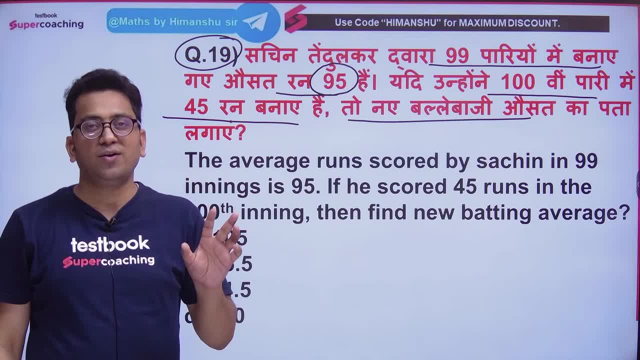 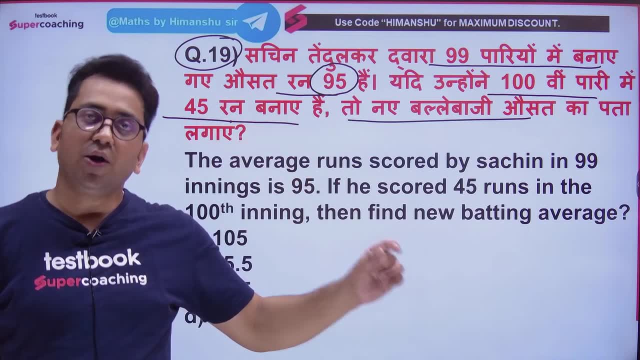 You just answer the homework question in the comment section. that's enough for me. So I am asking you so much that the new kids first of all go and subscribe to the channel And once click all the kids on the like button. 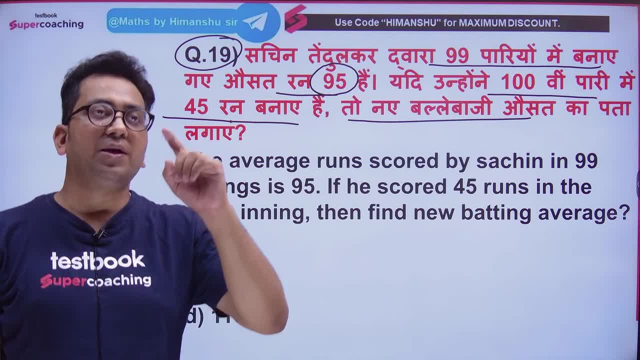 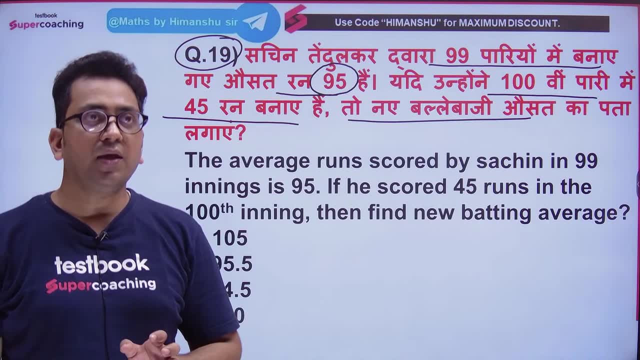 One kid is saying that he doesn't understand. You will understand when you join the session at 12 o'clock. If you join late, you won't understand anything. The one who doesn't understand will make a dirty face because he came late. 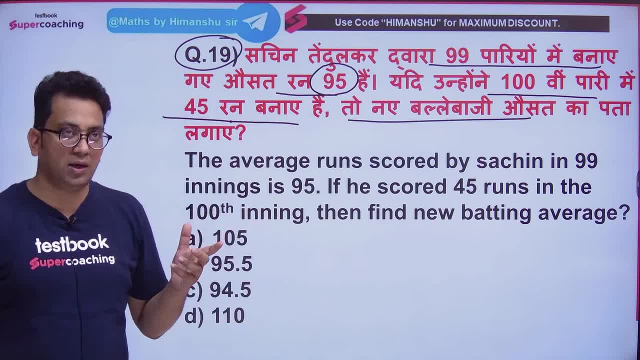 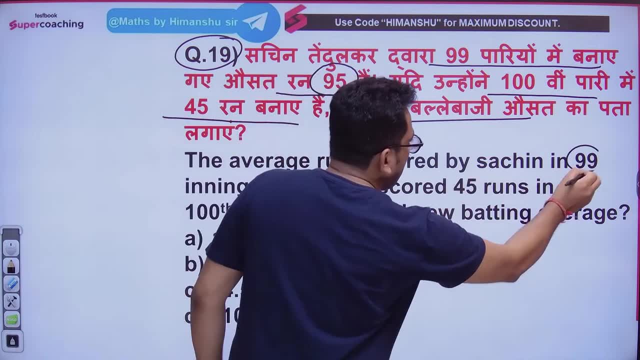 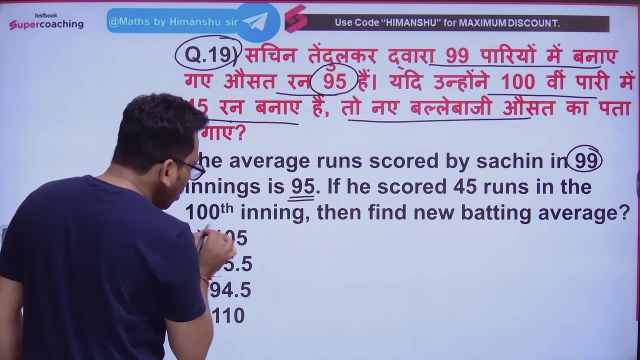 The one who will come first will always have a smile on his face. Come here carefully. Sachin says that. how many ausat runs has Sachin done in 99 paris? There are 95 ausat runs. Now he is telling you that he has made 45 runs in 100 paris. 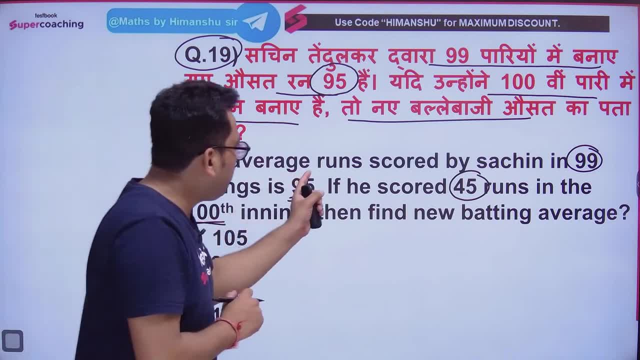 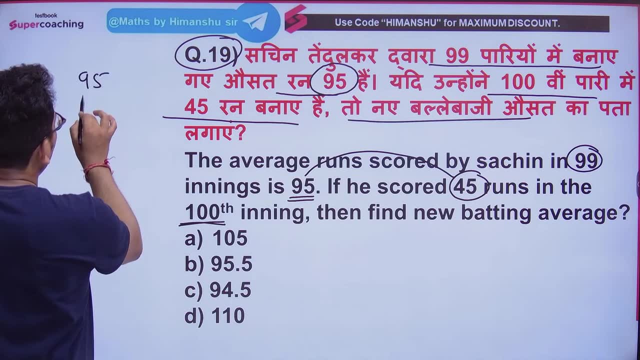 You tell me whether it is less or more, You will say that it is less than 95.. That means there will be a loss. How much loss will there be? See the difference Now. see the difference by reducing 45 out of 95.. 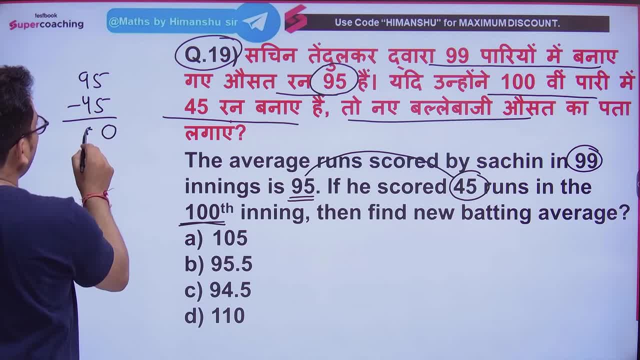 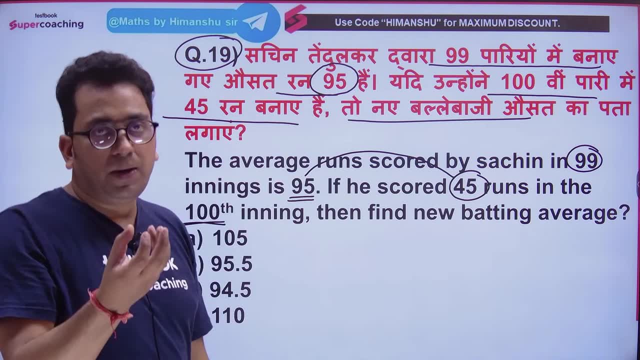 How much is the loss? 5 out of 5 is 0.. 4 out of 9 is 5.. There will be a loss of 50.. How many paris is this loss going to be equal to In 100 paris? 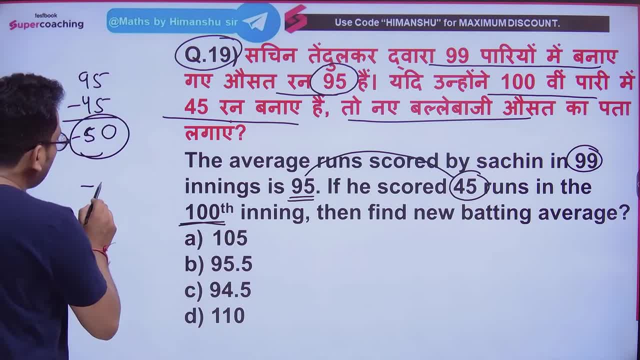 Because now there are 100 paris, So the loss of 50 will be equal to 100 paris. That means- each one you are able to understand- There will be a loss of half and half. And what does half mean? It is 0.5.. 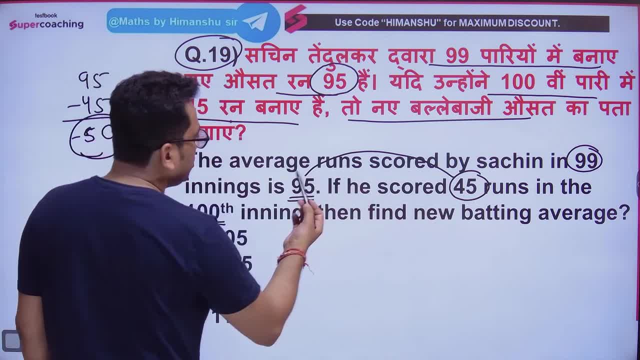 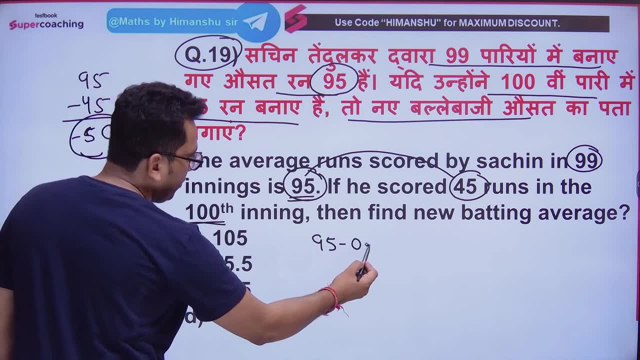 So the first ausat- Sorry, The first ausat- you had 95. Now there will be a loss of half in it. That means 95 minus 0.5. That means 94.5 will come. Our answer is 94.5.. 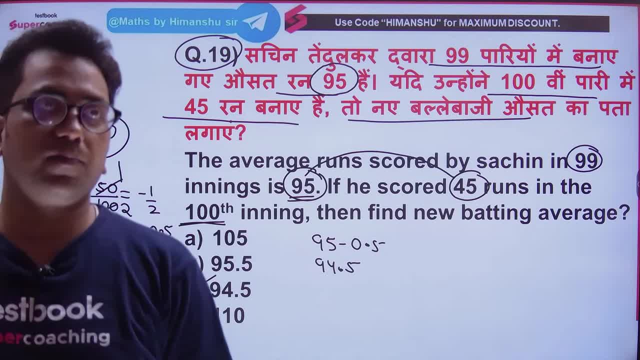 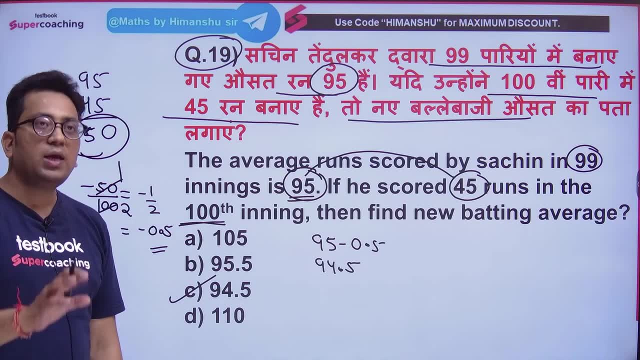 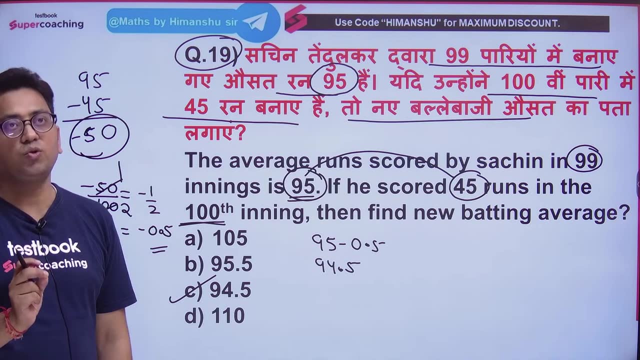 Now you are able to understand, C will be the right answer. Okay, C is our answer. Those who did not understand, repeat the session once. Okay, And try to join at exactly 12 o'clock, Then you will understand everything. 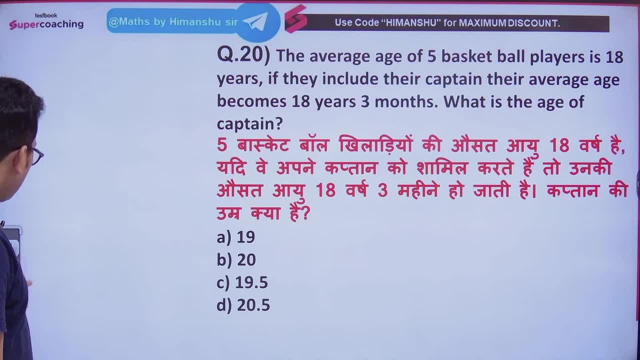 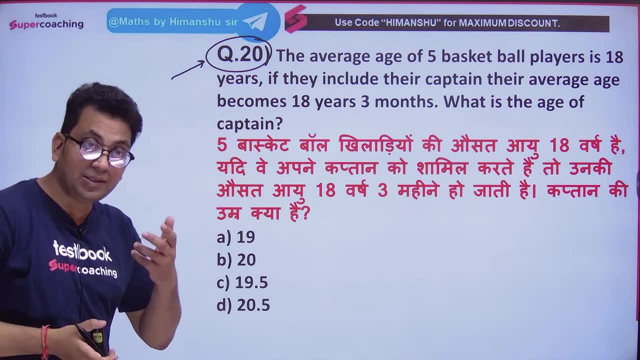 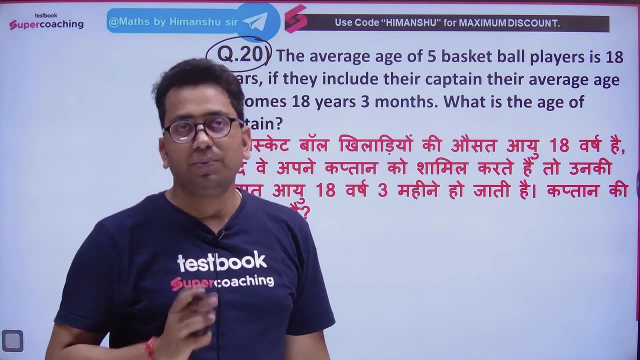 Okay, Last question of today's session. This will be your homework question. All of you have to answer this in your homework. Okay, It is a good question. I want everyone's answer in the comment section Tomorrow, What I have brought for you at exactly 12 o'clock. 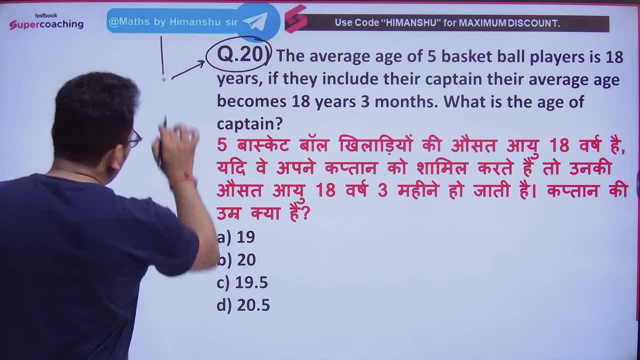 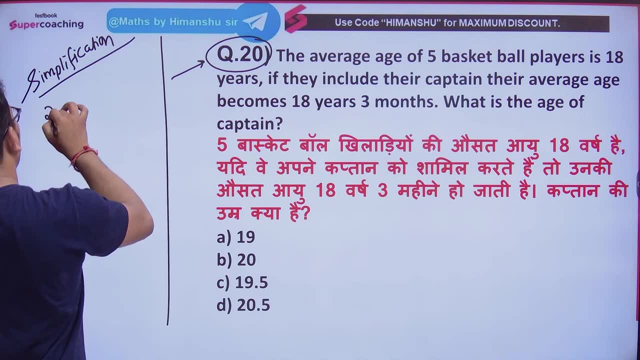 First of all, listen to that Very important topic. Tomorrow, I am going to teach you. Simplification means to do it easily. Simplification means to do it easily. It is a very important topic From the point of view of all exams. 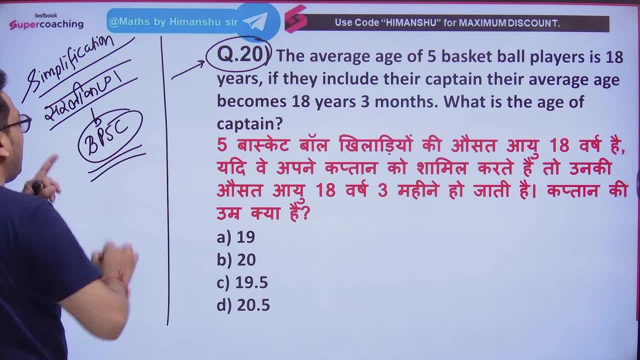 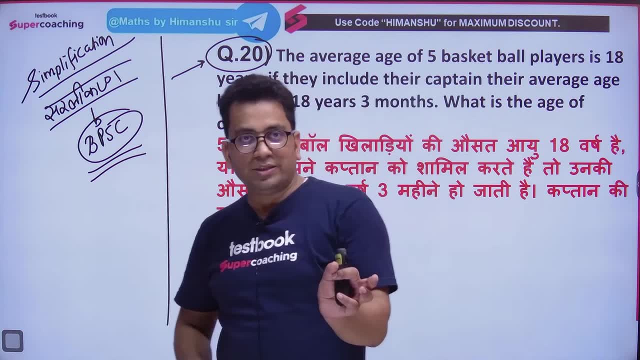 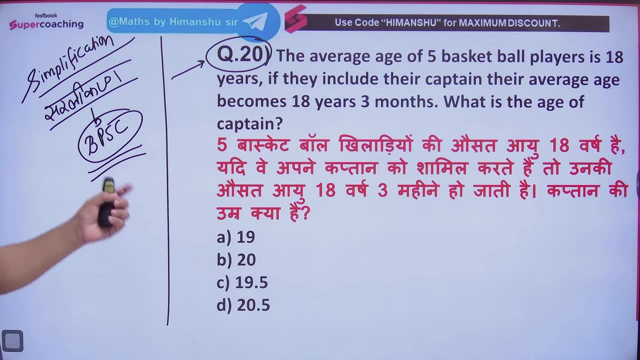 And especially in BPSC, Because we are studying for elementary math And here simplification becomes very important. Simplification, Approximation, Simplification- This can be a part of our BPSC pattern in elementary math. So we are going to study simplification in tomorrow's session. 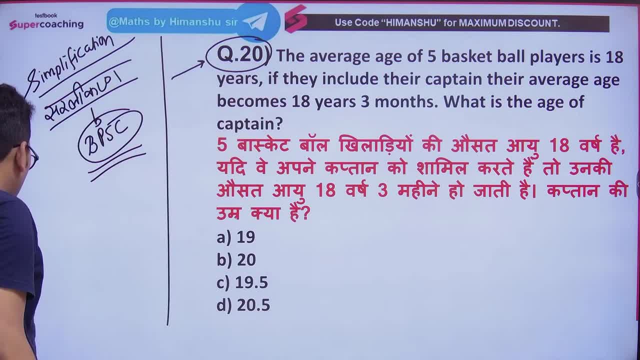 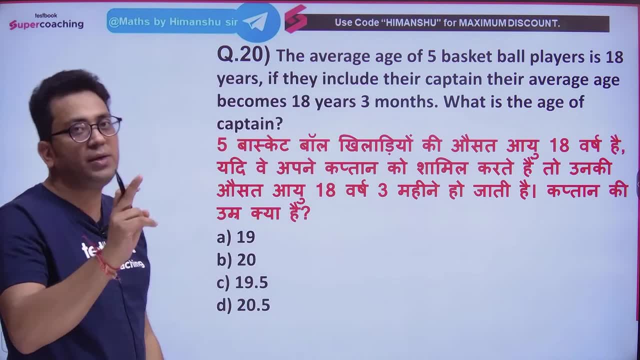 Okay, Let's go So. I hope so today's session will be beneficial for all of you. I would like Every child who is watching my session The answer to this question in the comment section. Be sure to do it Along with. 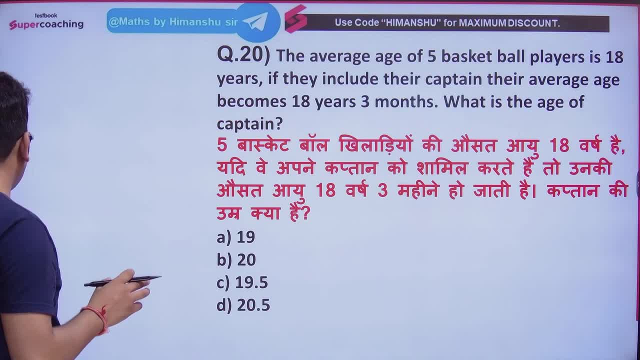 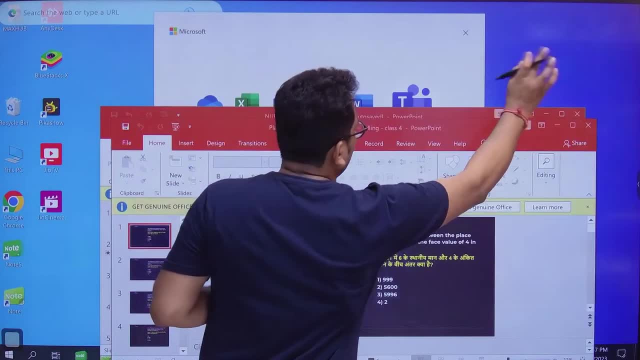 I will tell you all. If you want to join with Bihar Shikshak Bharti batch, Then how can you join? So you don't have to do anything, You have to go here. I will tell you everything here, Okay. 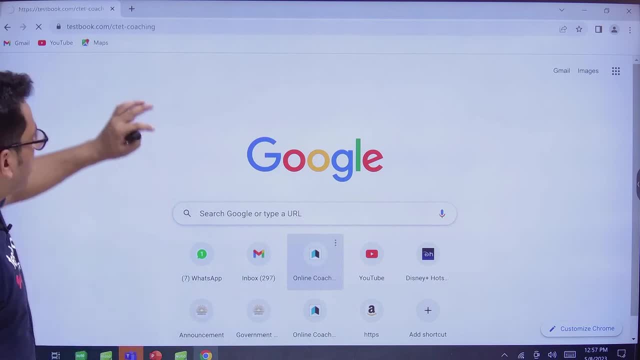 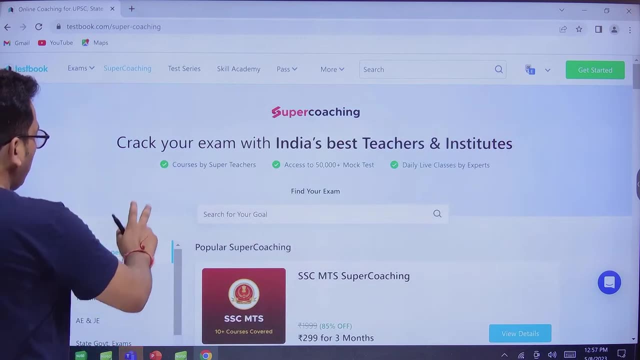 You will go here And as soon as you go to testbookcom. So you have to go here, Super coaching section, Click on super coaching And here you have to pick Teaching exam. Okay, As soon as you pick the teaching exam. 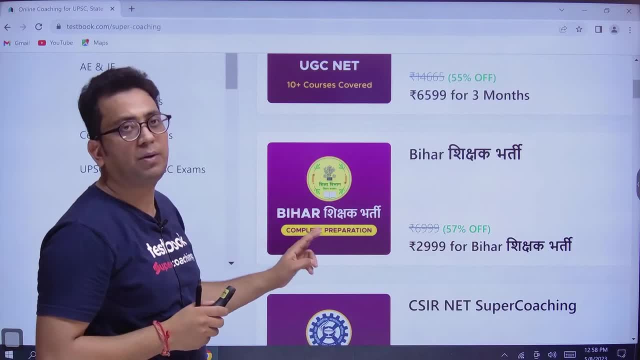 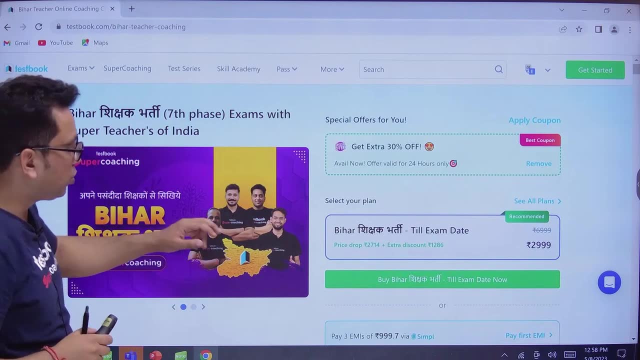 You will see. on the second number, Bihar Shikshak Bharti batch, You will click on this banner. After clicking on this banner, You have to click on this banner again, Which you must be seeing here: Bihar Shikshak Bharti batch. 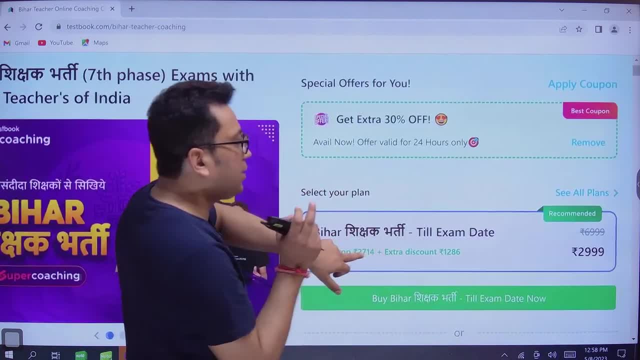 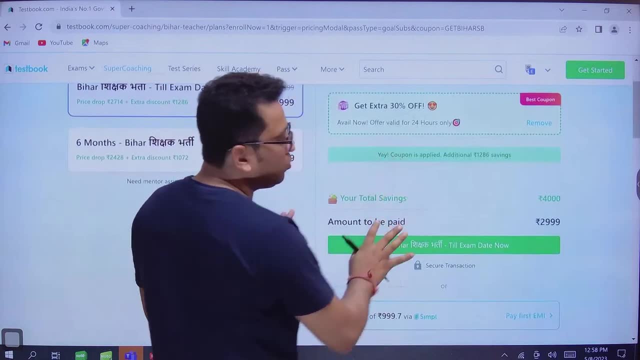 This is till exam date. That is, the batch is going to be with you till the exam date. Okay, So as soon as you click on this banner, You will have this option here. Payment option will open, But before paying I will tell you the code. 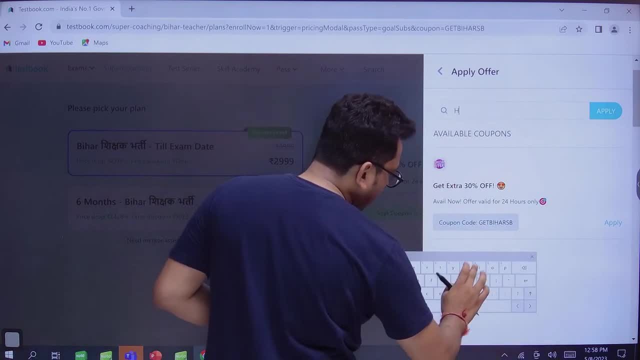 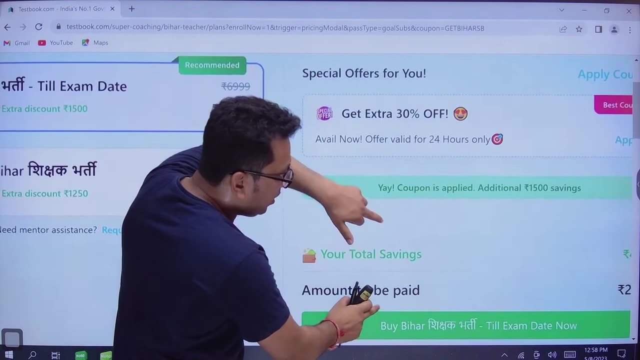 Which you will apply, the code here Which I have told you many times: H I M? A N S? H? U Means Himanshu. When you will apply this, Then your price here, The fee of the batch, will be reduced here And you can go here and enroll in this. 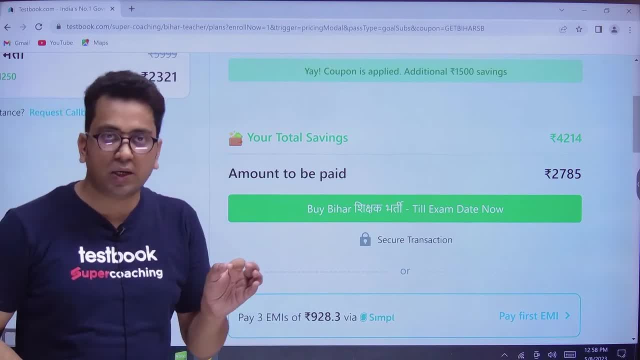 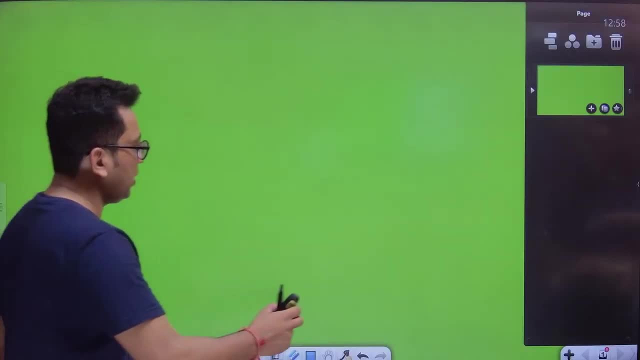 Any query, Any doubt? Maths by Himanshu. There is a telegram channel. From this telegram channel, Every child, Whichever child, is not connected till now, You all will connect with this telegram channel. Okay, So here This telegram channel. 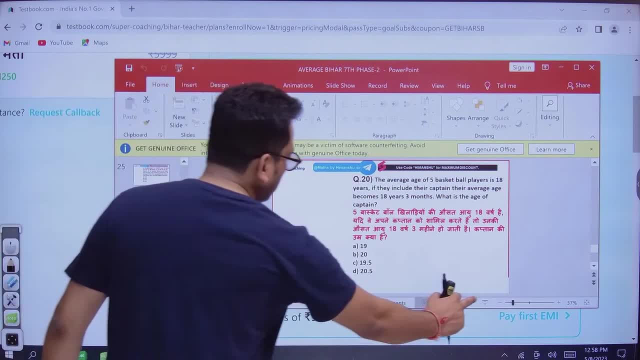 Maths by Himanshu. sir. Here you will get all the links of all the sessions And PDF notes. You will get them here, So I will meet you all In tomorrow's session, Exactly at 12 o'clock. Till then,